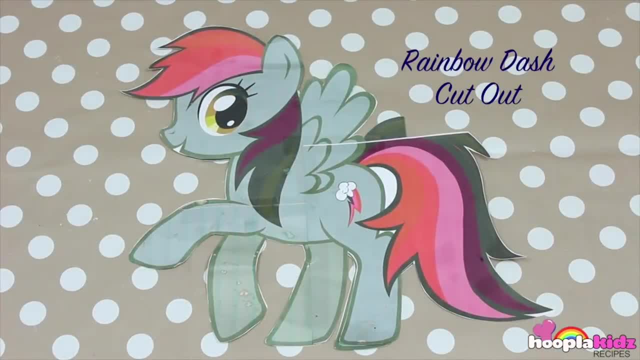 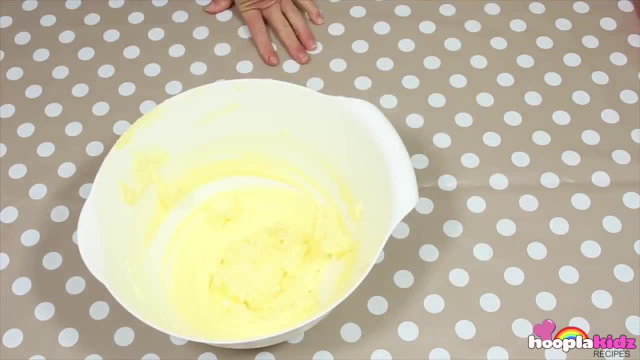 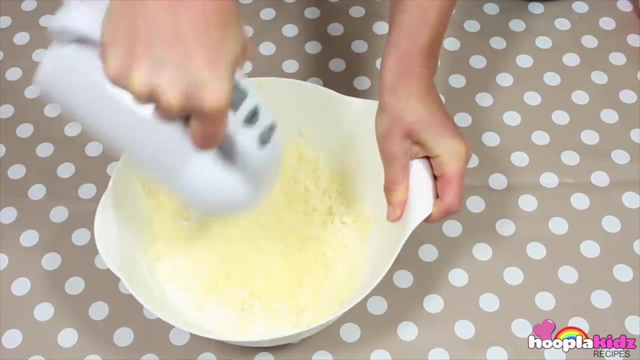 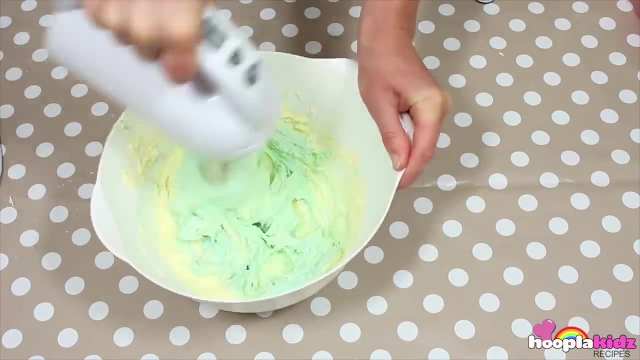 You're also going to need a rainbow dash cutout the size of your cake. It's to add our butter and icing sugar to a bowl. We're going to mix this using an electric whisk. Add some blue food colouring to colour the mixture. 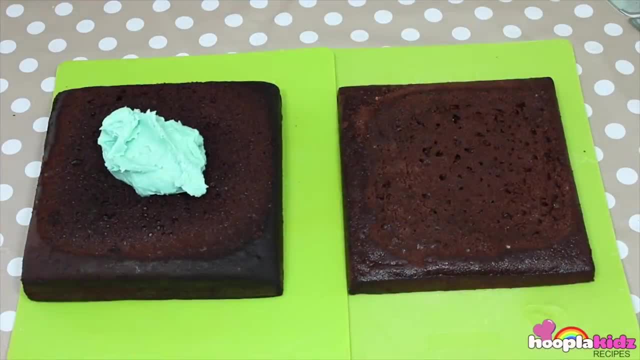 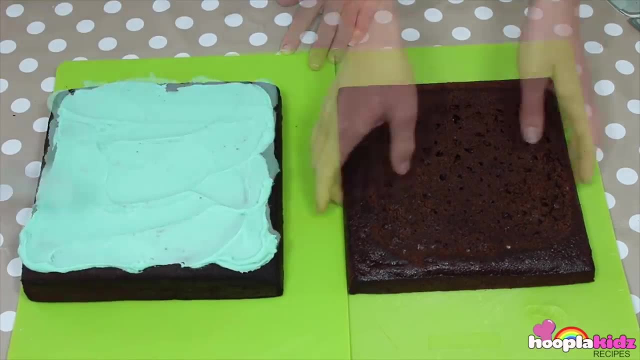 Once you're sure you've got no lumps, we're going to take our blue icing and we're going to spread it on top of one of our cakes. We're going to add the other cake on top. It's kind of like a giant sandwich. 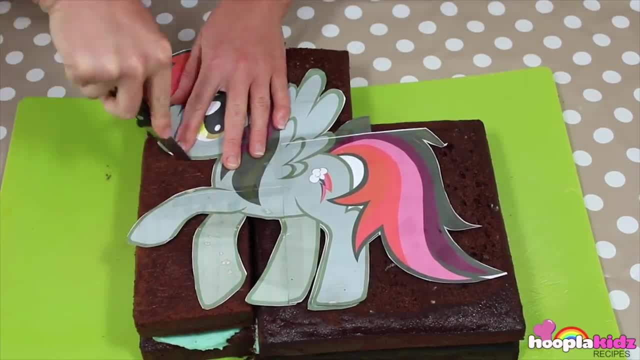 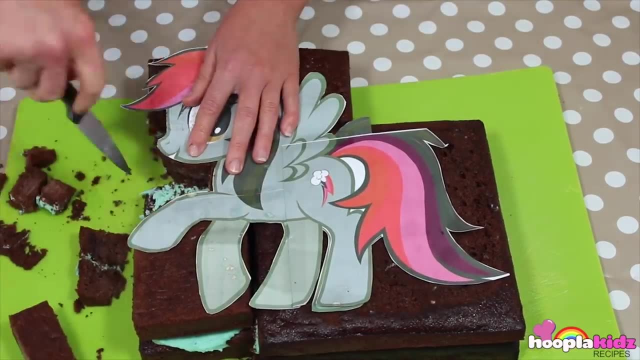 Now we want to put our rainbow dash cutouts on. We're going to add the blue icing to our rainbow dash cutout on top of our cakes. We're going to cut around the edge. This means we'll get a giant rainbow dash shaped cake ready for decorating. 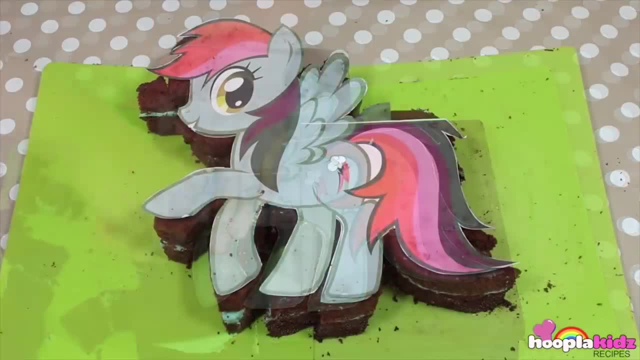 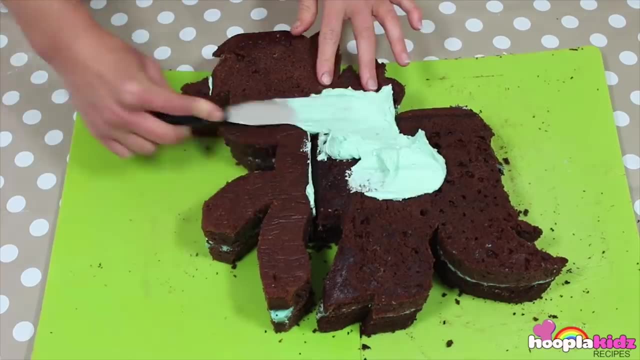 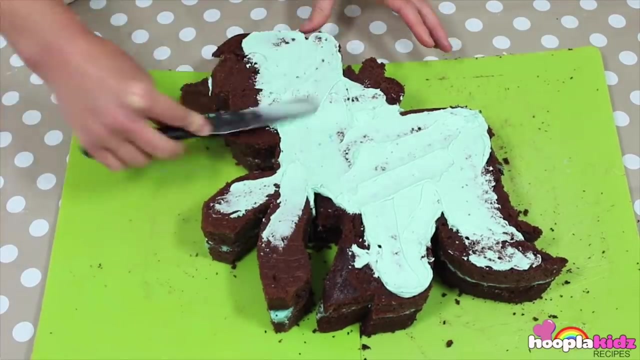 This will take some time, so be patient. And there you have it. It's not meant to look perfect yet because we haven't decorated it, So we're going to cover the entire cake in blue icing. This is only a base coat, so it doesn't matter if you. 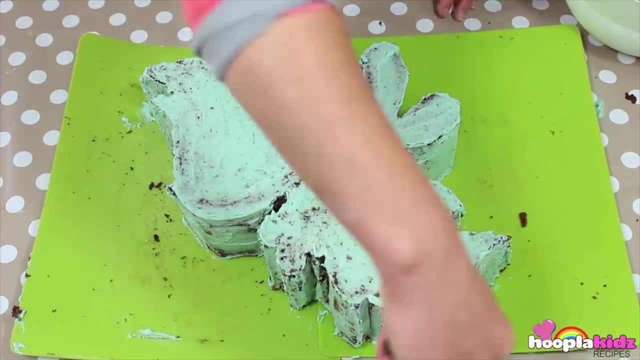 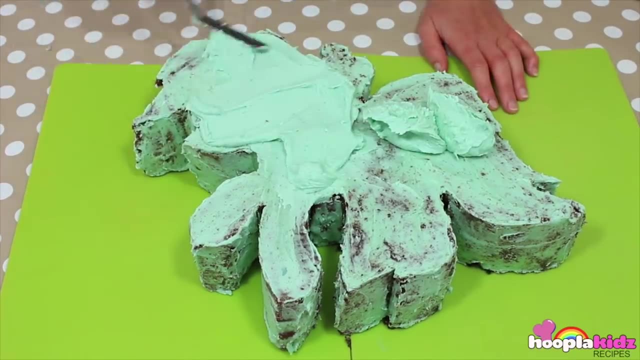 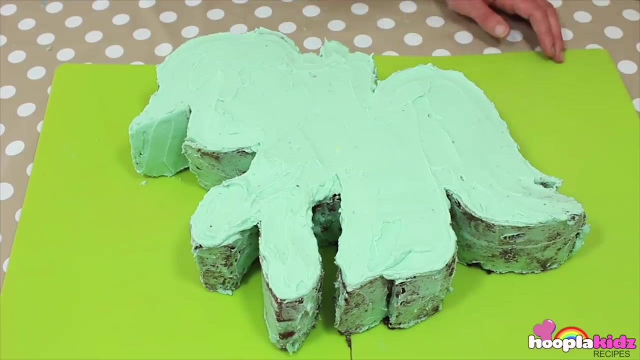 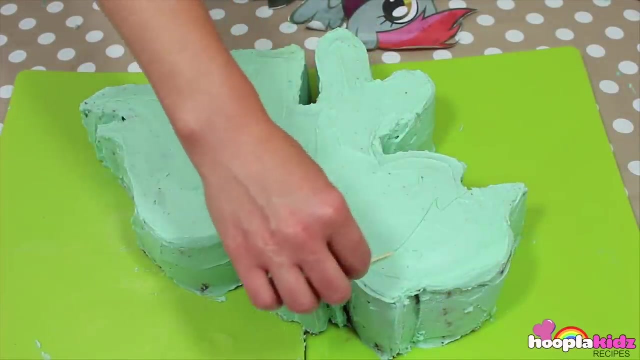 can see some of the cake underneath. We're going to refrigerate for two hours. Now that's done, we're going to add a second coat of icing Smooth down the edges. Once you're happy with the icing, we're going to take a cocktail stick and we're 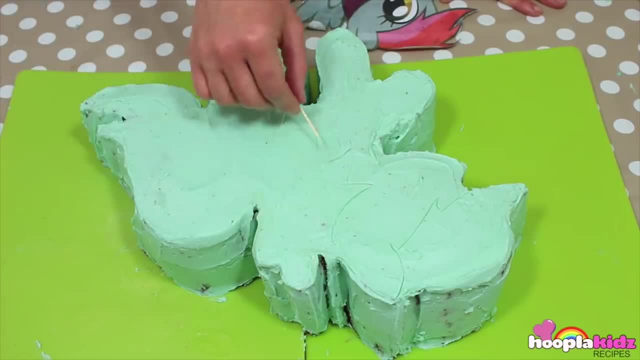 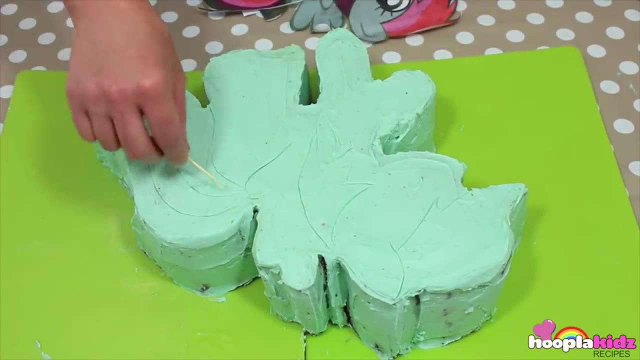 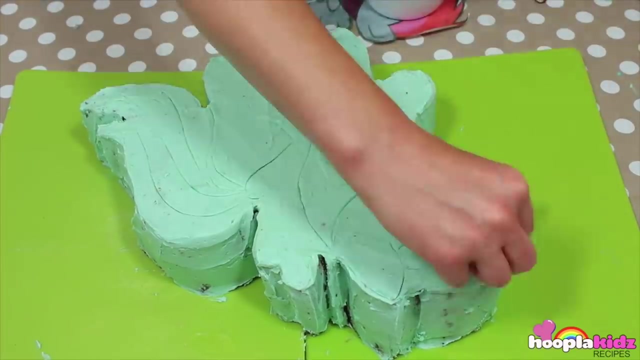 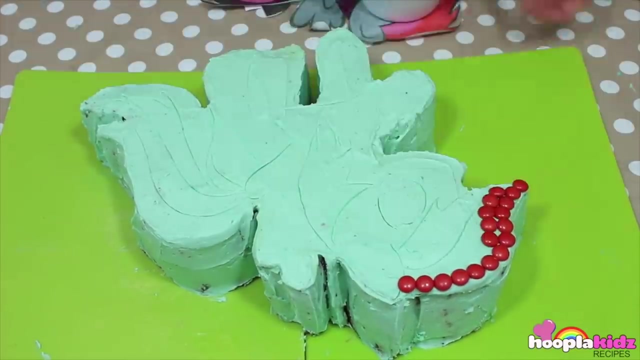 going to sketch the outline of rainbow dash's detail. This will make it easier when we add the M&M's. Now it's time for the fun bit: Adding the M&M's. I'm starting at the top, but you don't have to. You can start wherever you want. 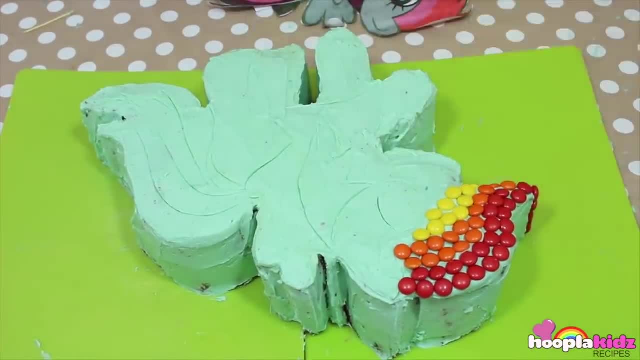 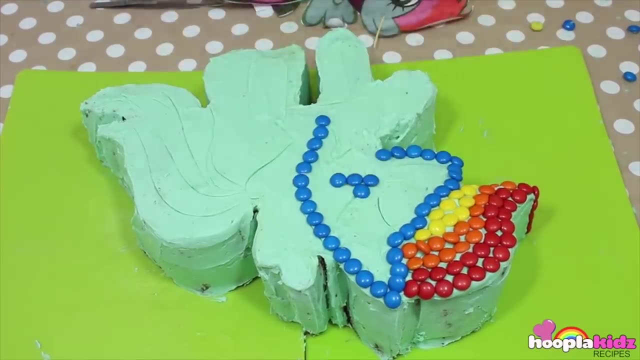 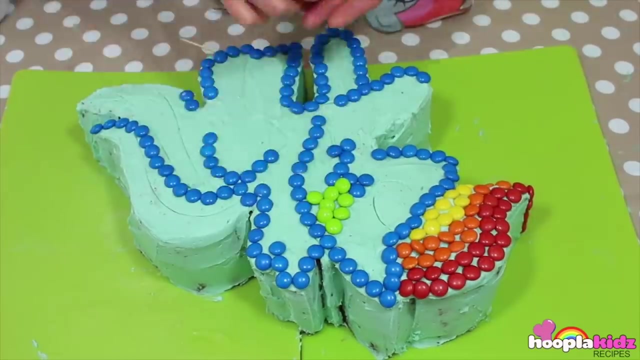 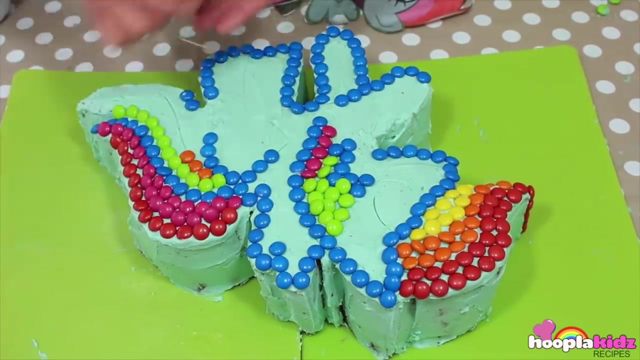 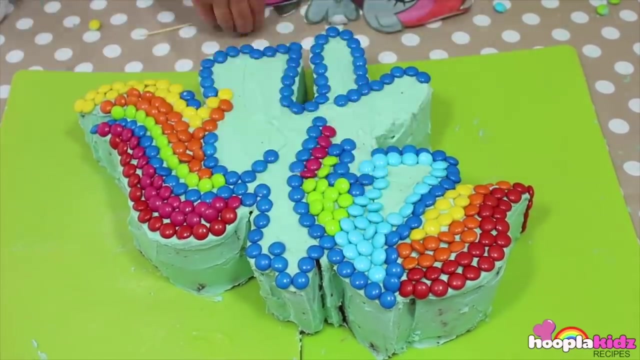 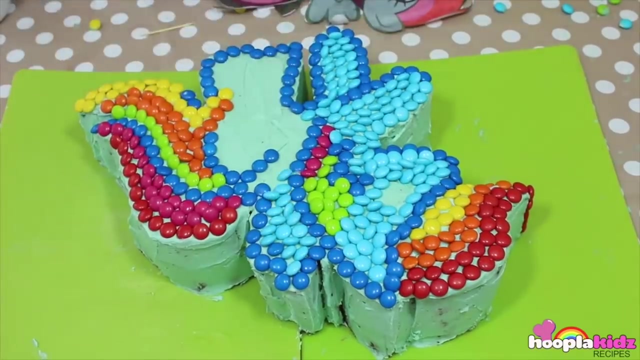 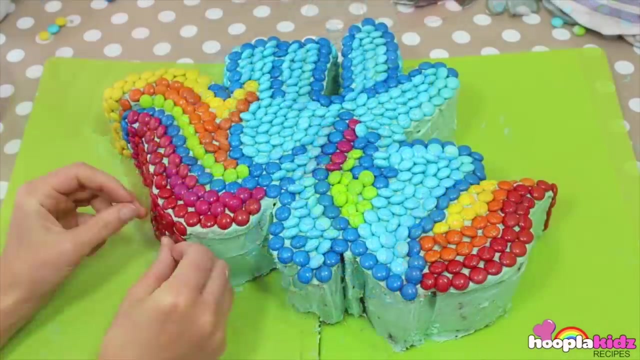 This is where it really helps that you've done an outline using a toothpick. This is where it really helps that you've done an outline using a toothpick. It's already looking amazing, right. It's already looking amazing, right. The rainbow tail looks great. 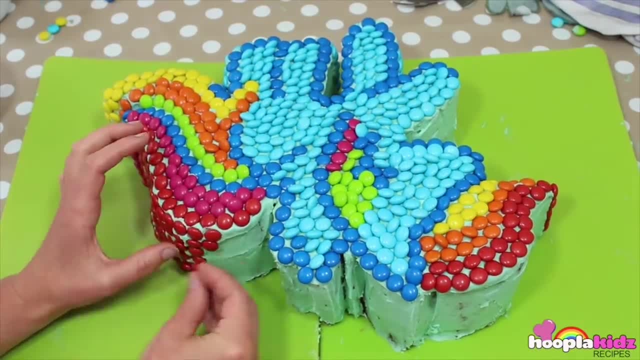 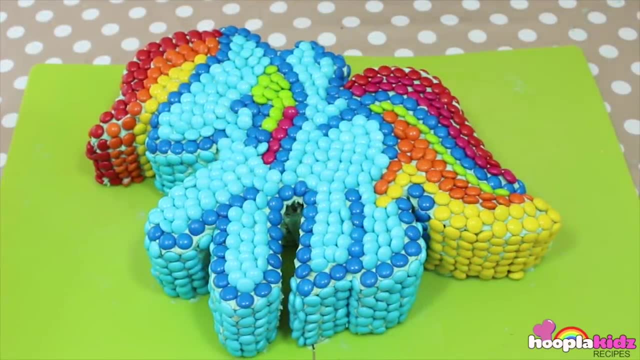 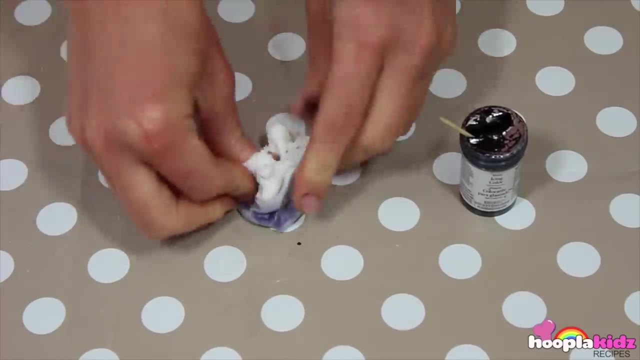 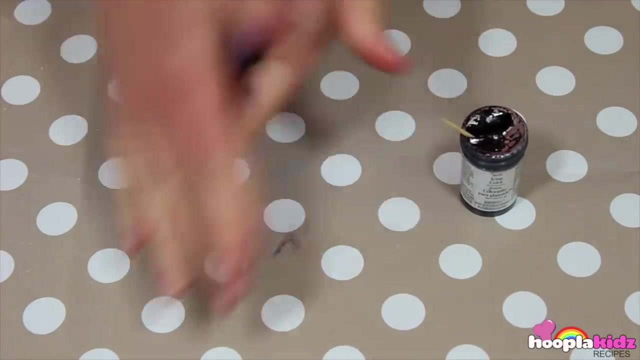 Don't forget to do the sides. And there we have it. It looks so cool. Now it's time to do some detail. I'm going to make Rainbow Dash's eye using white fondant icing. I'm going to add some colouring to make it dark purple. 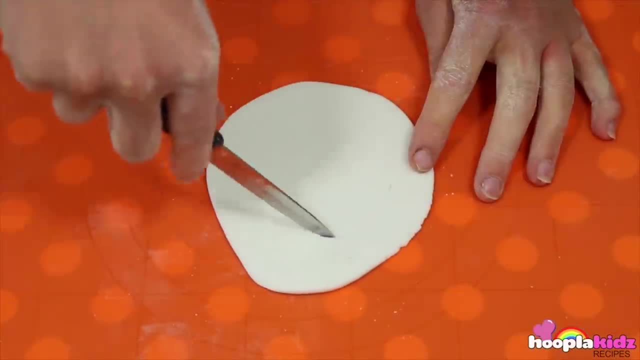 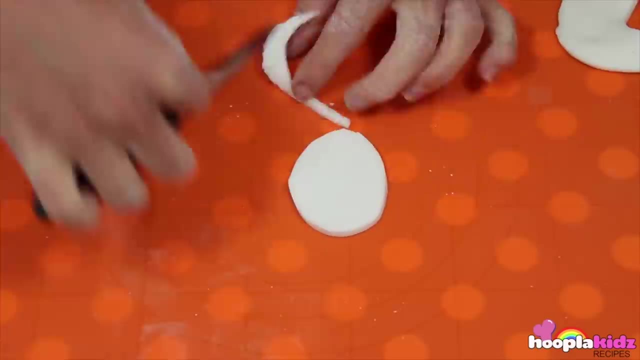 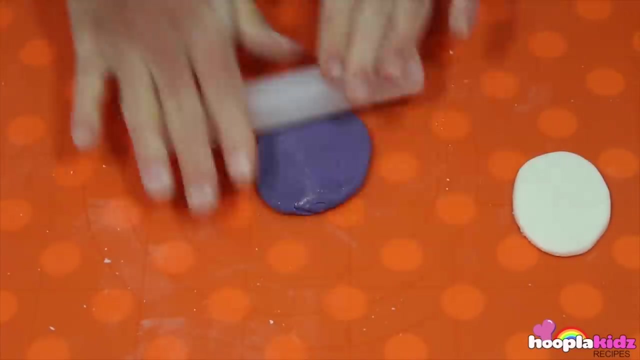 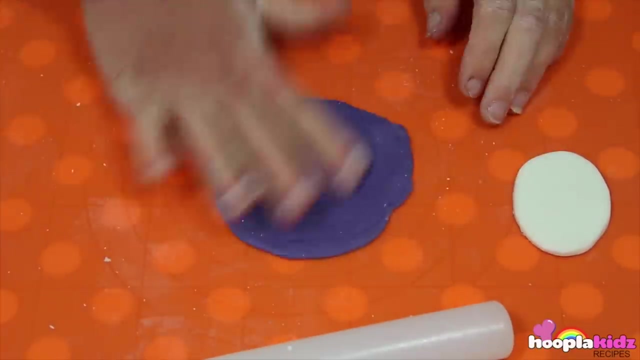 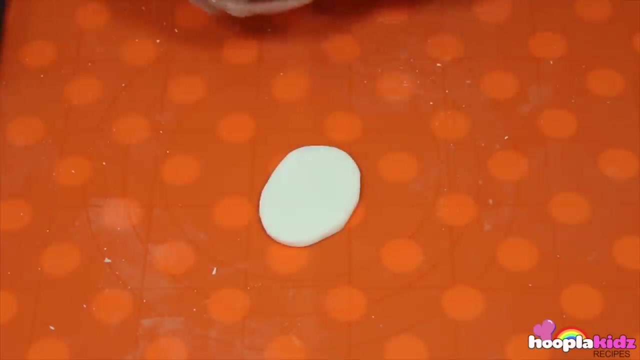 Set that aside And now we're going to take some white fondant icing And cut the shape of Rainbow Dash's eye out. Roll out the dark purple. We want to cut an oval shape. This is going to sit on top of the white fondant icing. 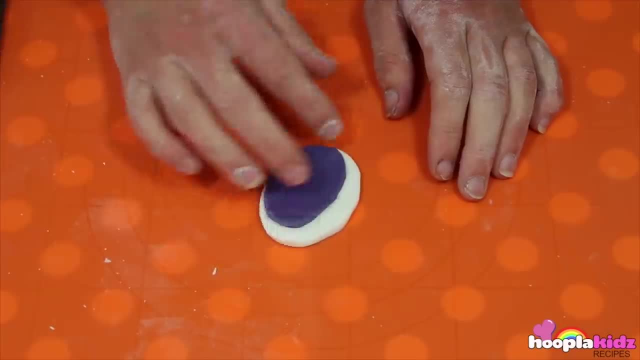 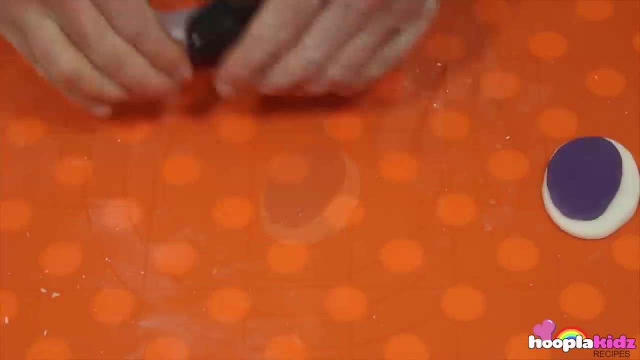 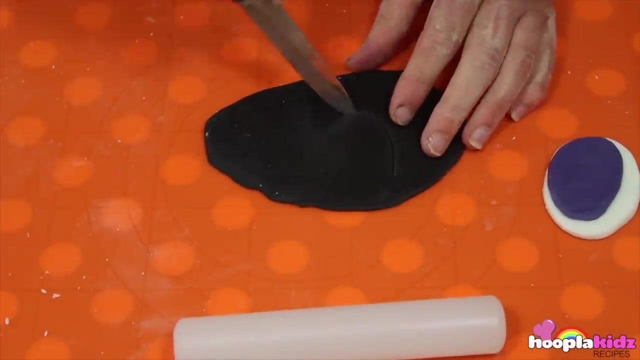 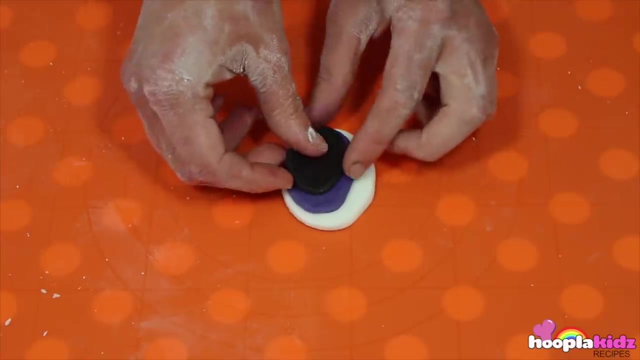 Just like so. Make sure you smooth down any edges. Now take the black icing. We're going to cut a smaller oval shape And add it on top of the purple. We've now got 3 layers. There's still one more to go. 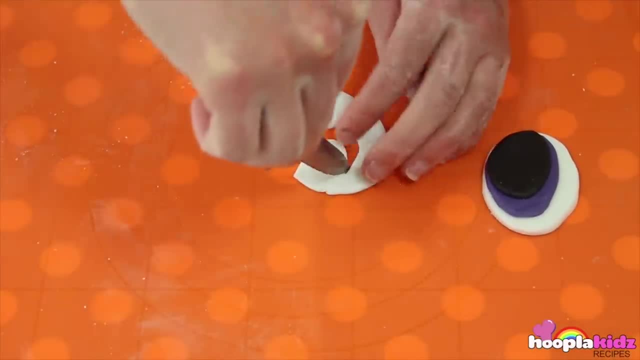 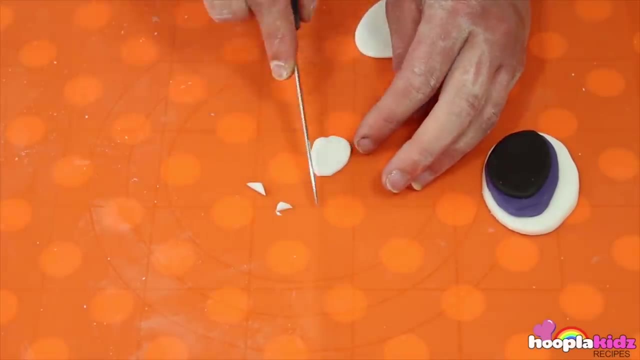 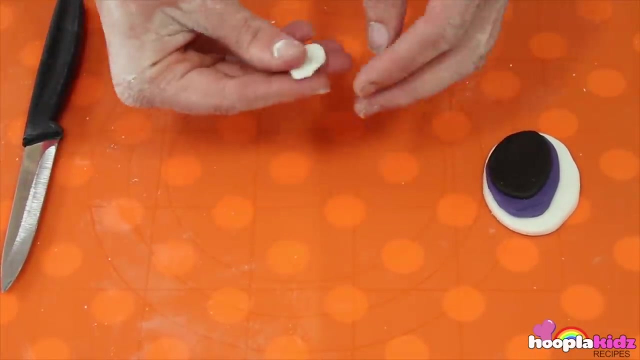 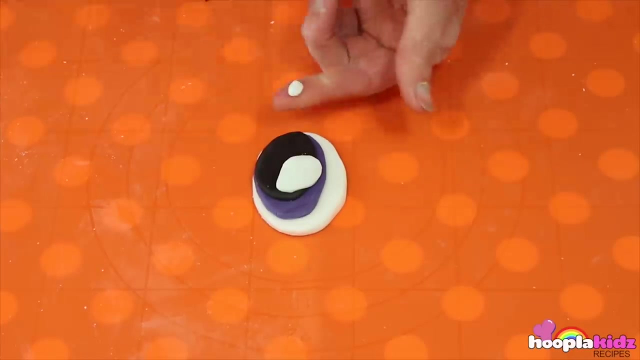 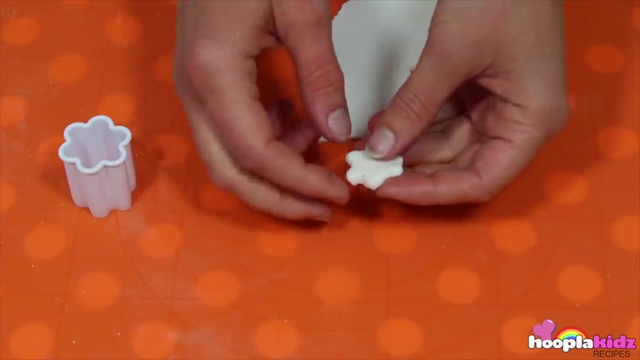 See you next time. and this is white. Add the white on top and finally, we're going to take a tiny ball of white icing just to add a little bit more detail. Now we're going to add detail to Rainbow Dash's body. I'm cutting out a cloud shape first. 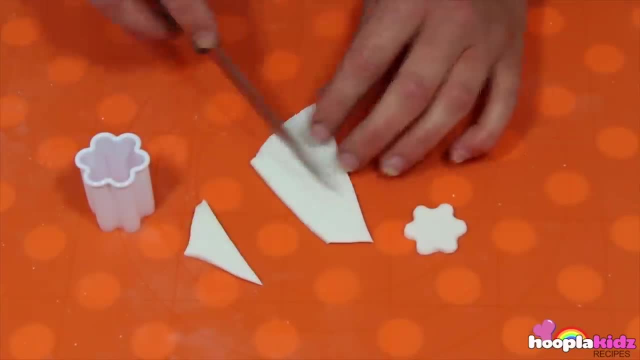 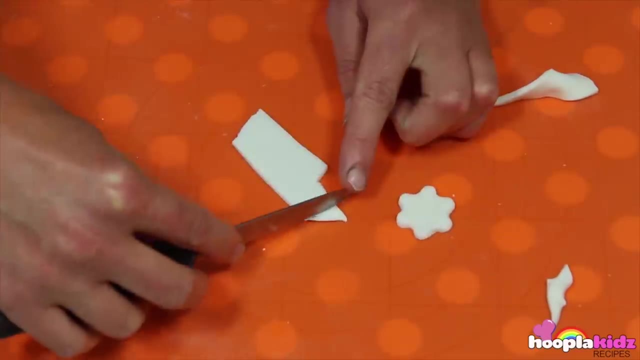 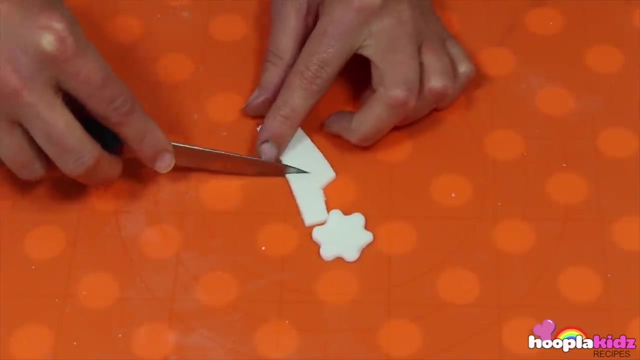 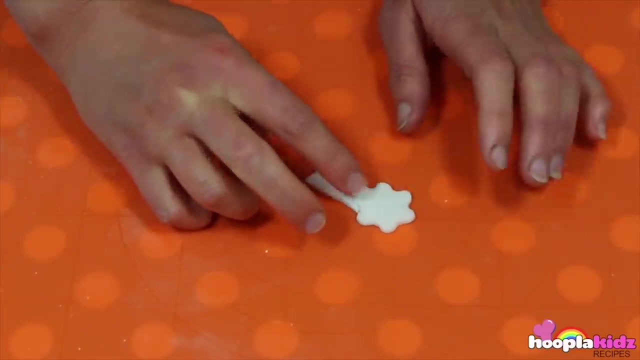 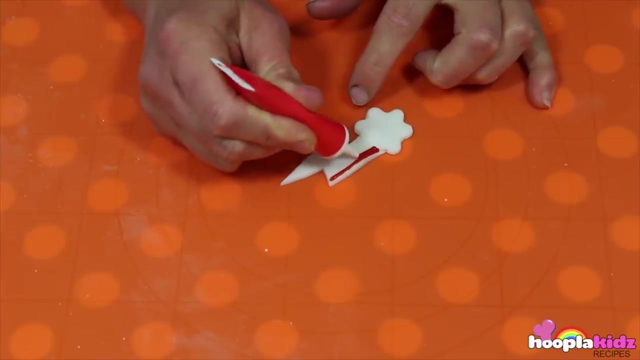 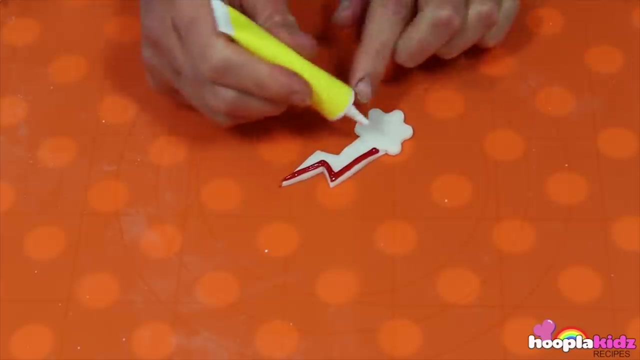 using a stamp. Now I'm going to use some flat fondant icing to make a lightning bolt. Stick the two together. Now, using icing, we're going to add color. I'm starting with red, Then yellow And blue. I'm outlining the cloud in black. 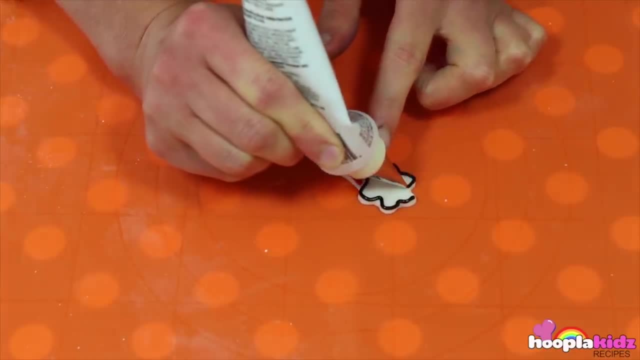 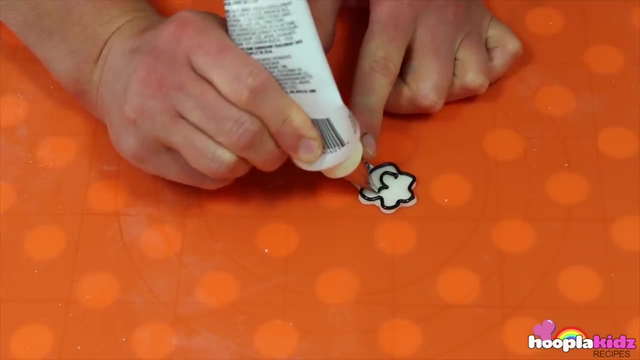 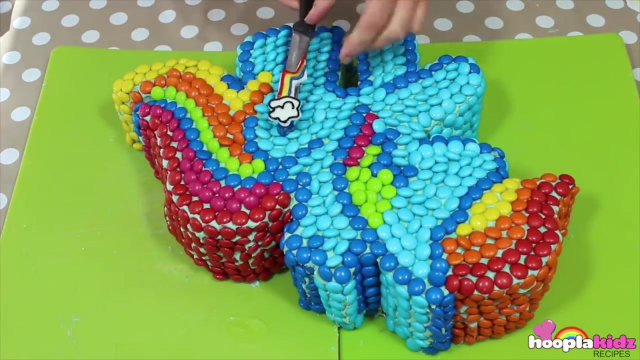 This is so it stands out on the amazing rainbow that we got on her body. Don't forget to subscribe to our channel for more videos like this, And don't forget to add detail And then add it Just like. so I'm using icing to stick the detail on. 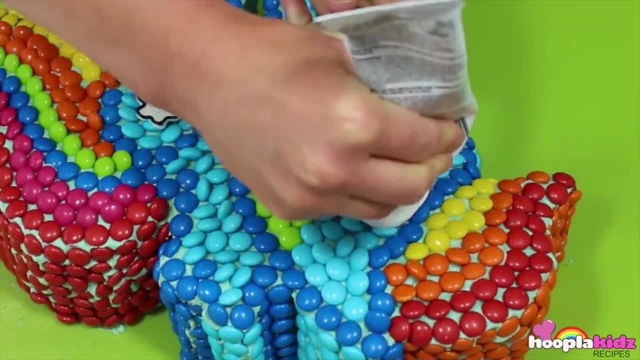 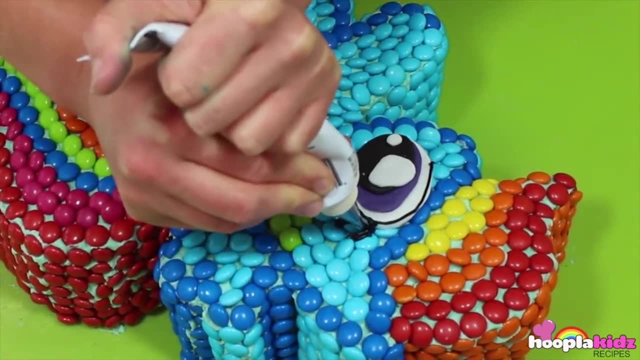 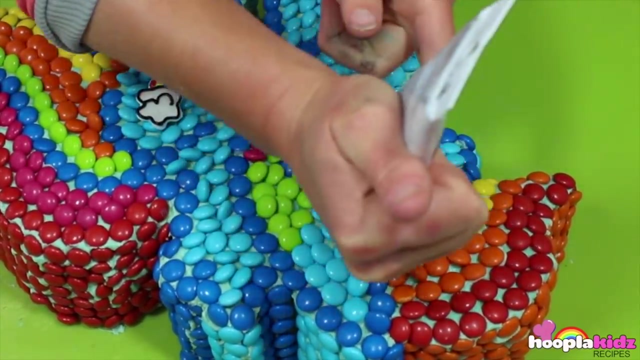 Including the eye. Once the eye is in place, I'm using the black writing icing to go around the edge and to add eyelashes. This looks amazing. I'm so happy with how it's turned out. This would be perfect for a birthday party. 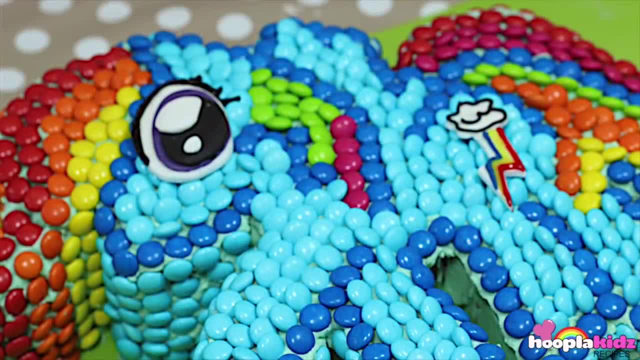 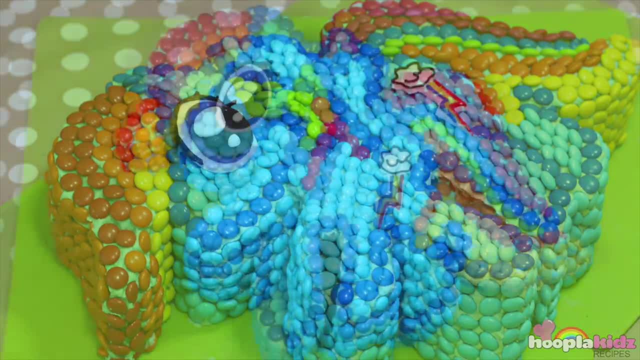 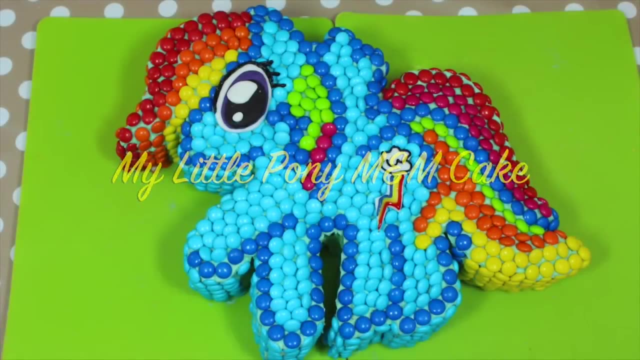 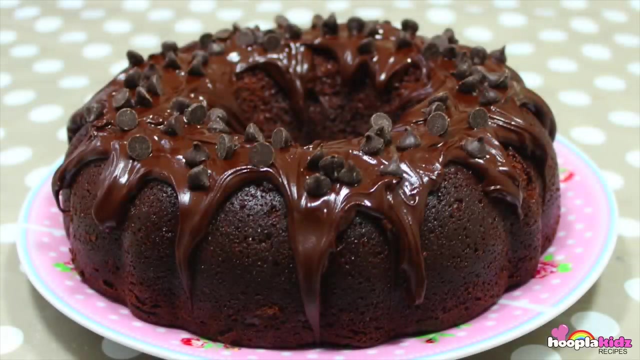 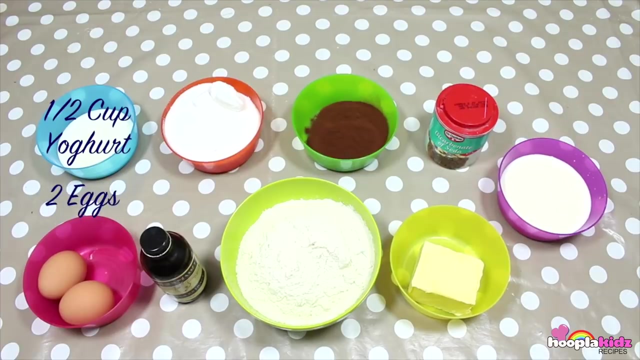 And it's going to taste delicious. A My Little Pony M&M cake. Great Chocolate cake: It's a classic, But it's super delicious. So for this you're going to need Half a cup of yogurt, Two eggs, One and three quarters of a cup of sugar. 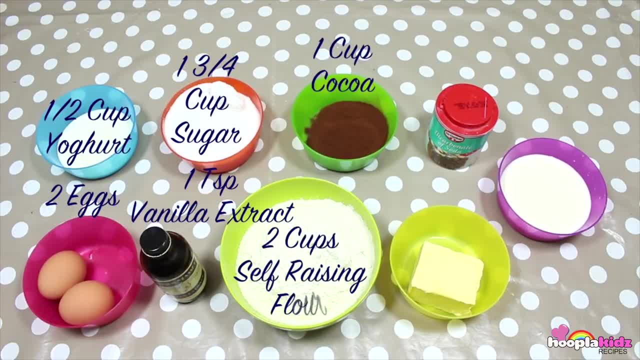 One teaspoon of vanilla extract, One cup of cocoa, Two cups of self raising flour, One and a half teaspoons of bicarbonate of soda, One cup of unsalted butter And one cup of milk. For decorations, you're going to need One cup of chocolate chips. 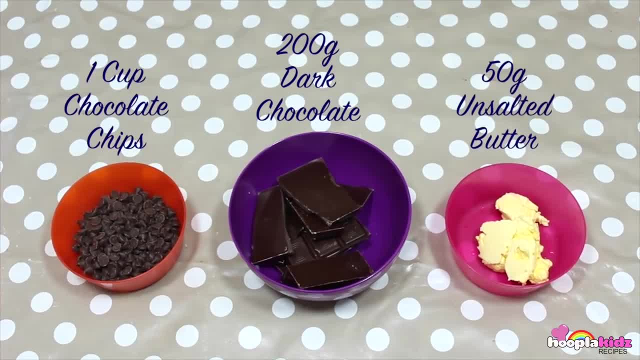 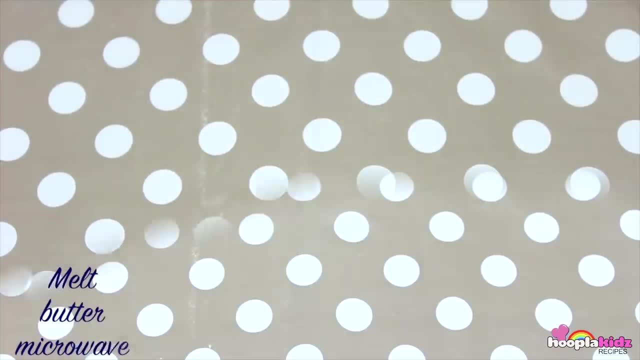 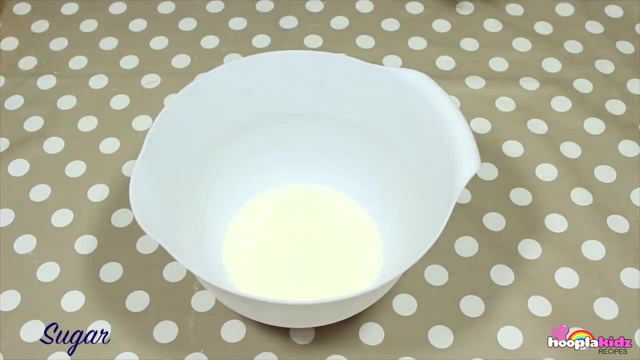 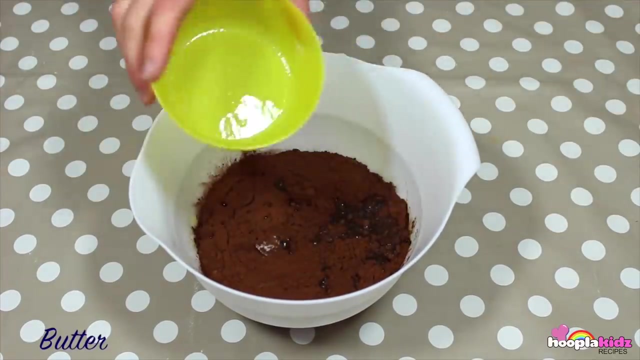 Two hundred grams of dark chocolate And fifty grams of unsalted butter. So the first thing we want to do is to melt our butter in the microwave. Now we're going to pour our milk, Sugar, Cocoa powder, The melted butter, Into a bowl. 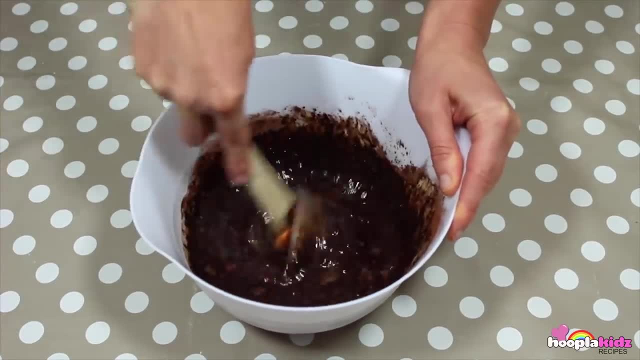 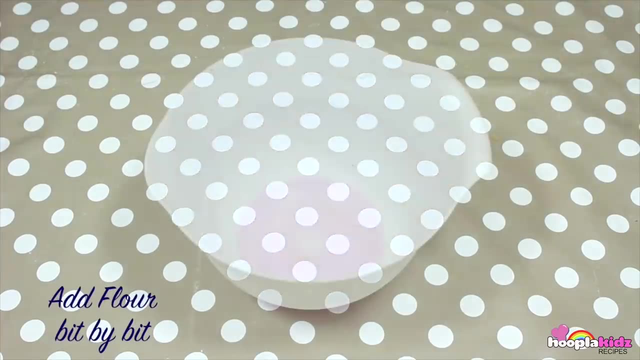 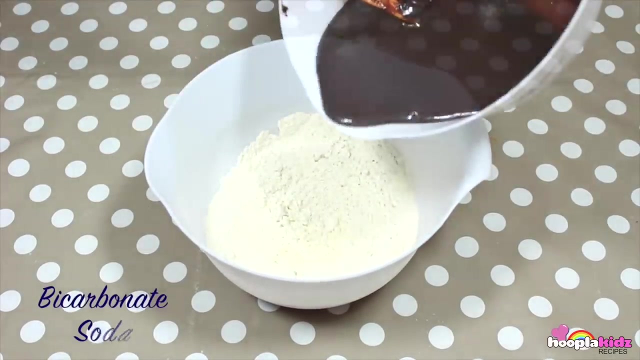 And we're going to stir. We don't want any lumps, So make sure you mix it really well. Now we're going to add our flour to a bowl And our bicarbonate of soda, Give it a stir, And then we're going to mix in our wet mixture. 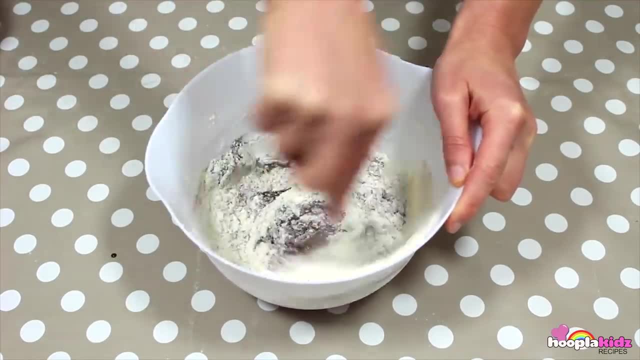 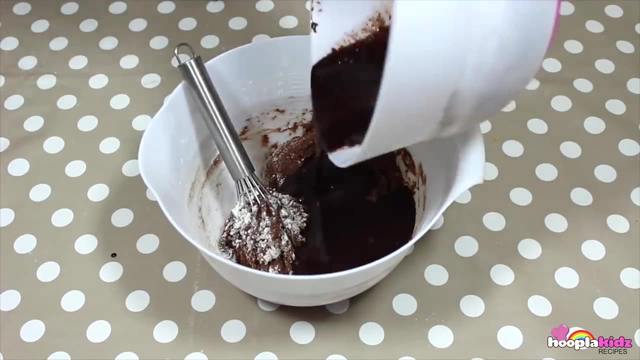 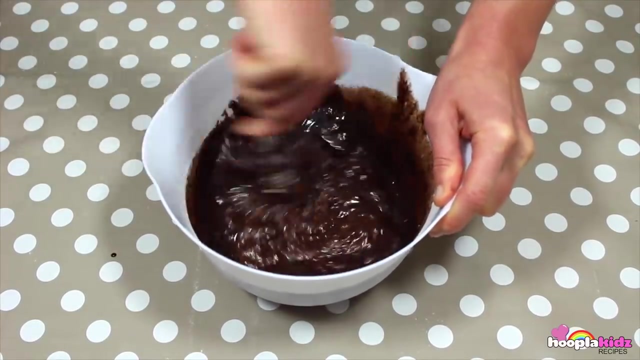 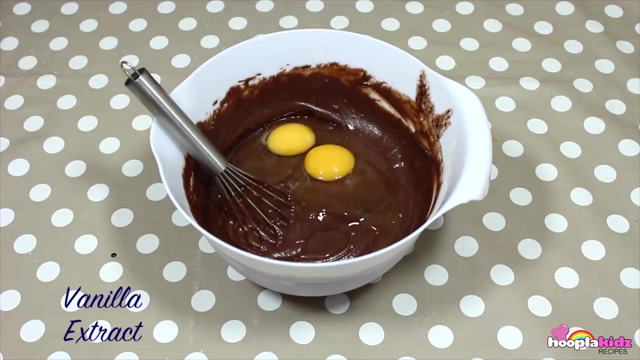 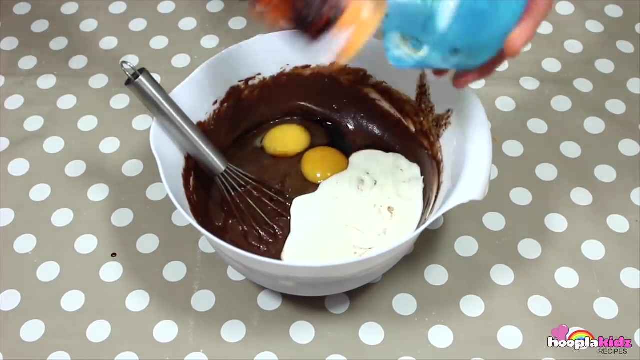 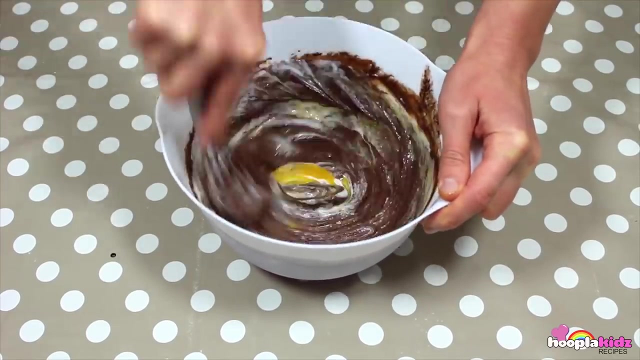 We're going to stir it in bit by bit. This will help make sure that there are no lumps. Keep mixing. Now we're going to add our eggs And our vanilla extract, As well as our yogurt. Mix together- Super delicious. 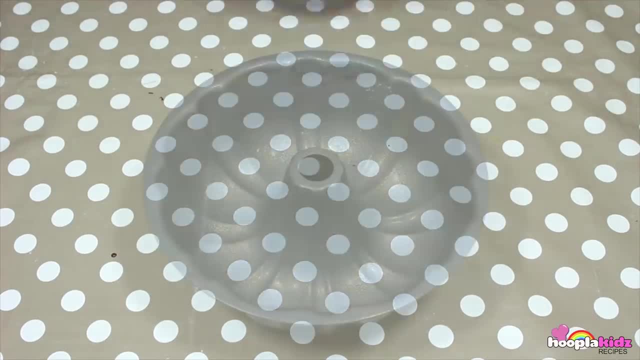 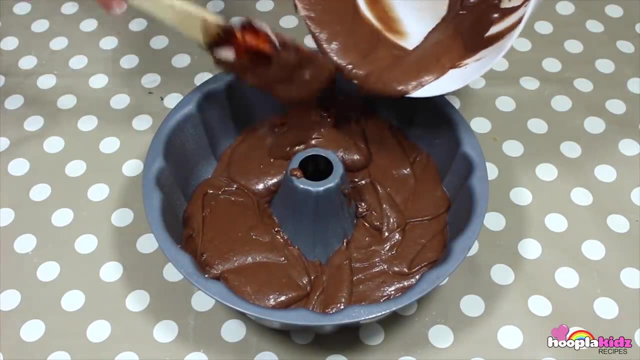 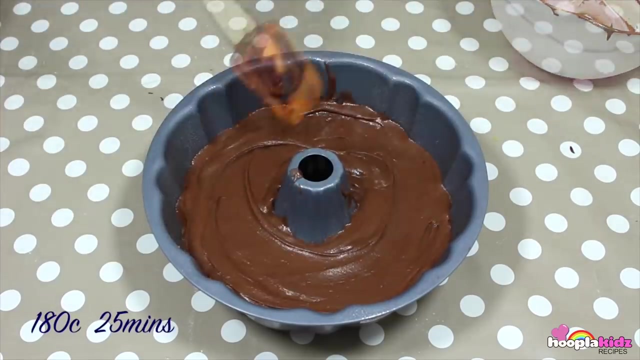 Who's going to lick the spoon? Now that the mixture is done, we're going to pour it into a cake tin. Pop that in the oven at 180 degrees for 25 minutes. Once that's done, we're going to let it cool whilst we make the icing. 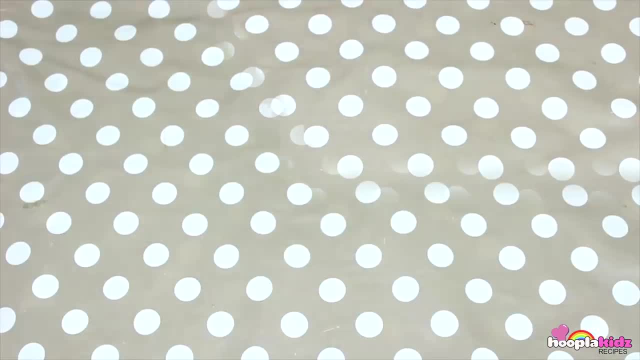 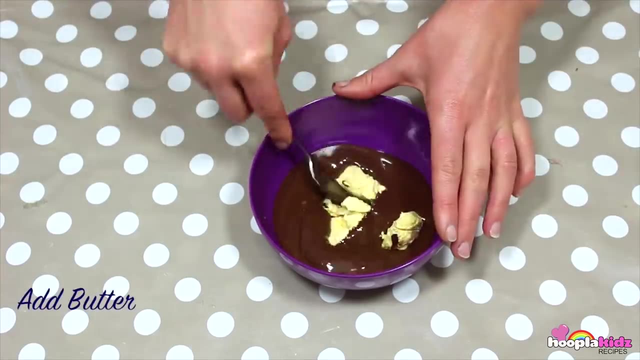 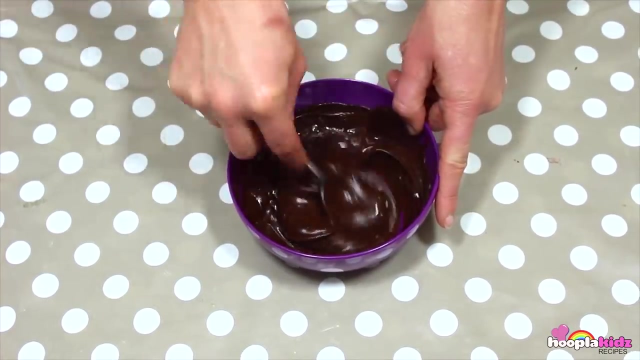 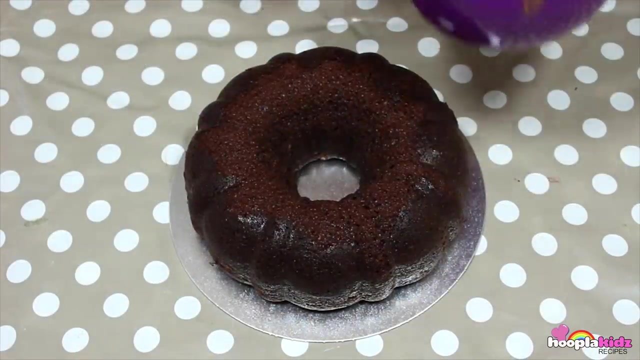 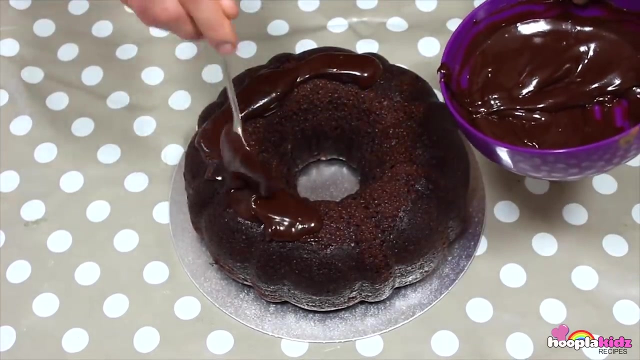 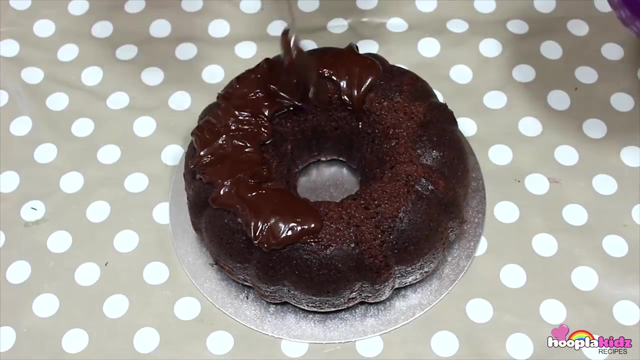 First we want to melt our chocolate. Then we're going to add our butter to that mixture, Give it a good stir. Now we're going to spoon the icing mixture over the top of our cake. I can't wait to eat this one. 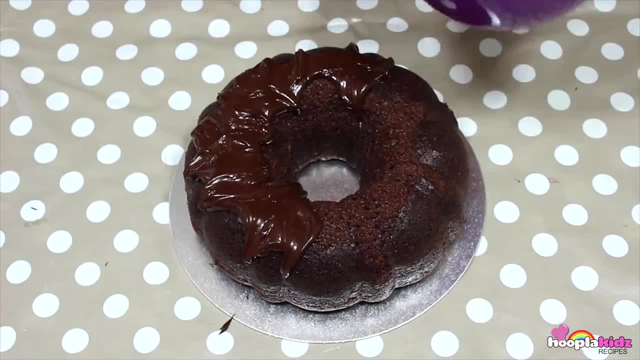 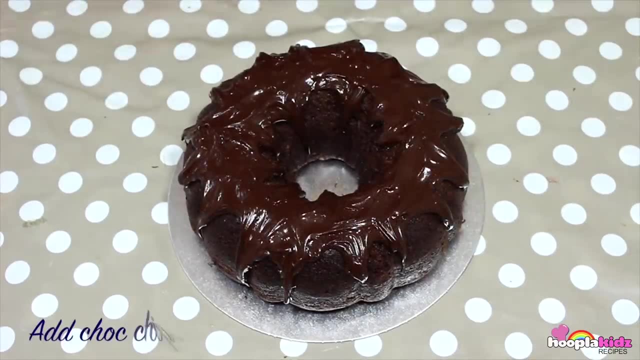 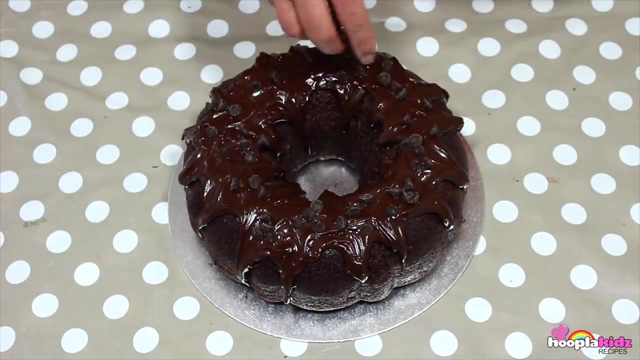 I'm letting the icing dribble down the side. Yum, We want to cover the entire top of the cake. And finally, we're going to add our chocolate chips. Super delicious, And there you have it: An amazing chocolate cake. 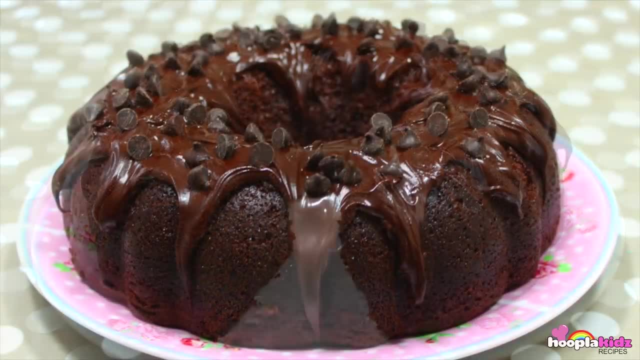 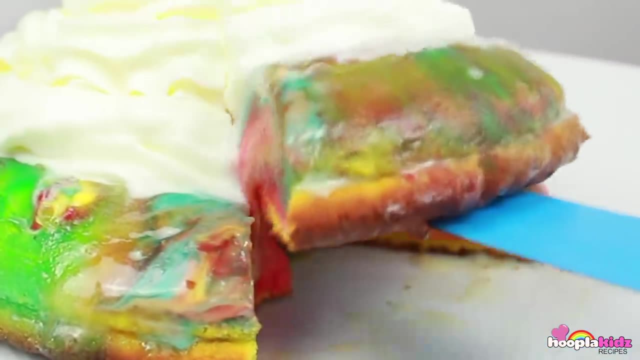 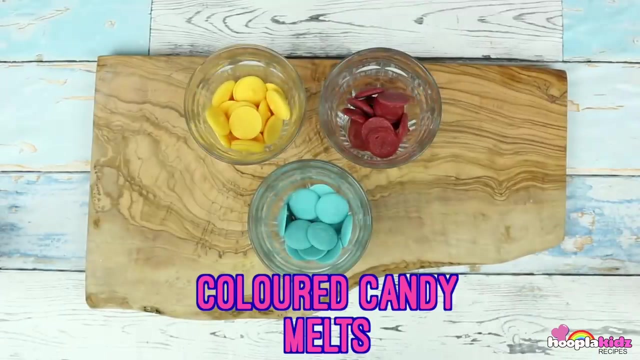 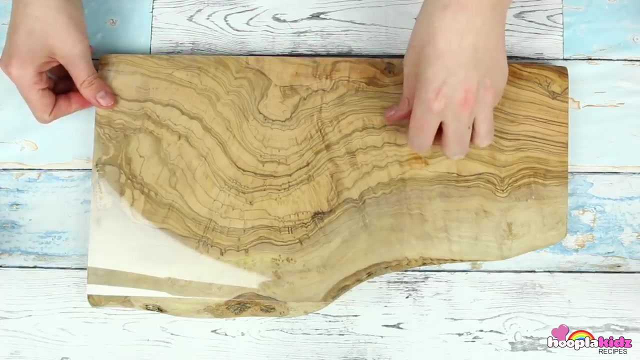 Moist and delicious. Yum, A rainbow lava cake. Look at that gooey rainbow centre Delicious. So let's get started with some coloured candy melts. We're going to melt them in the microwave. Now let's take some clear plastic film. 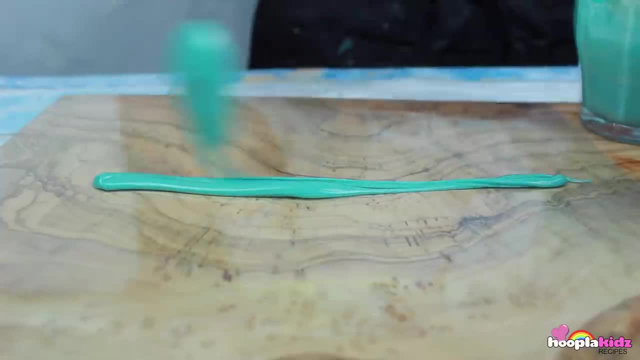 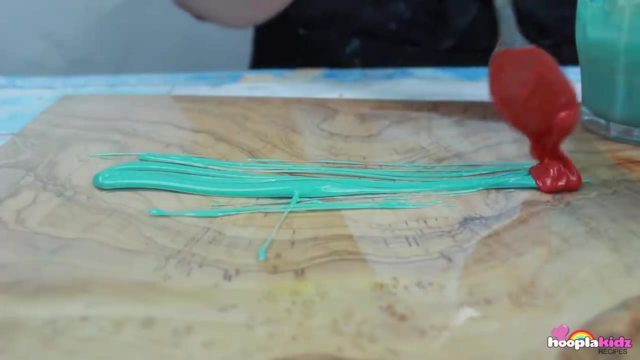 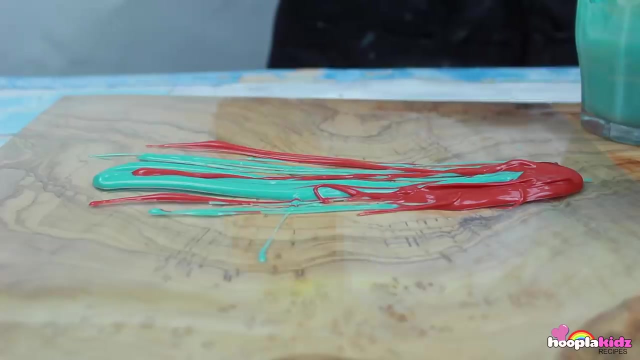 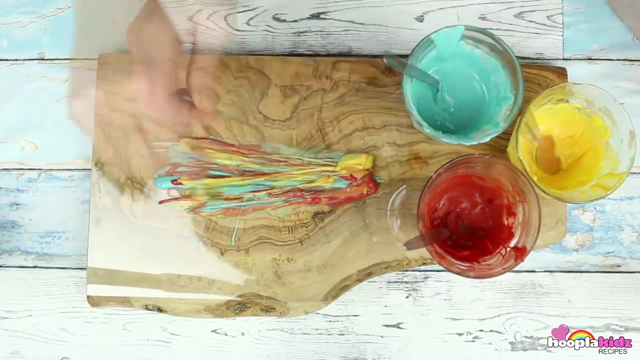 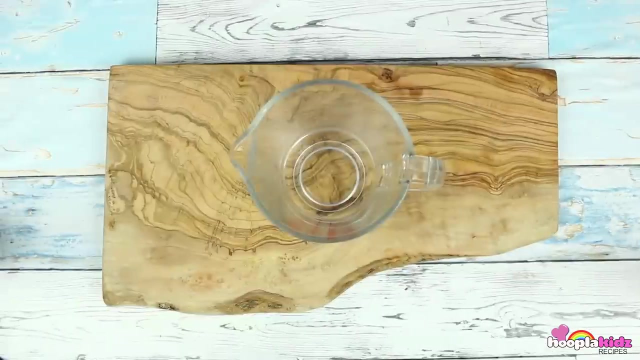 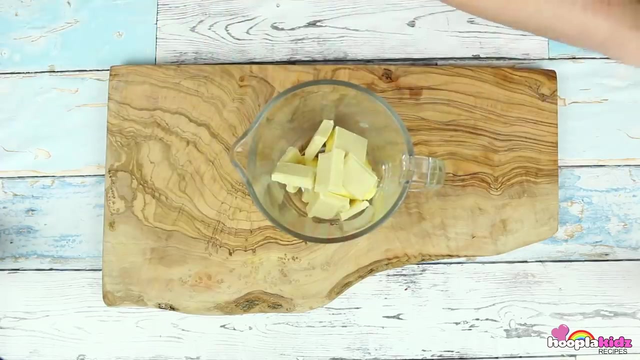 I'm adding the melted candy melts onto the clear plastic. I'm adding the melted candy melts onto the clear plastic. This is going to create a great decoration, so keep layering up the different colours. Allow that to set in the fridge. Now I'm going to take one third of a cup of butter. 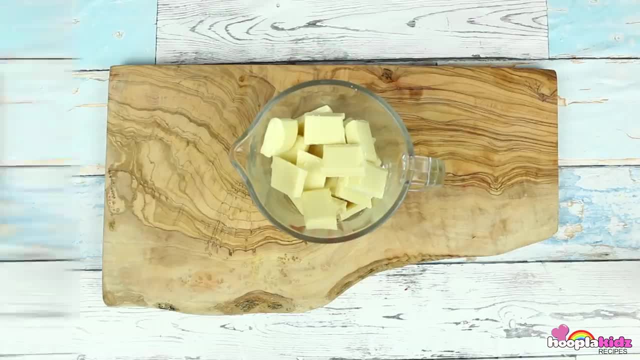 I'm adding six ounces of white chocolate to that. Melt that in the microwave. Now I'm adding two egg whites and four egg yolks. Using a whisk, I'm whisking it all up And then adding a quarter of a cup of sugar. 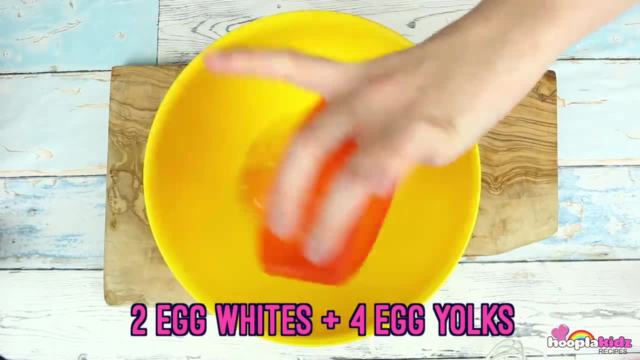 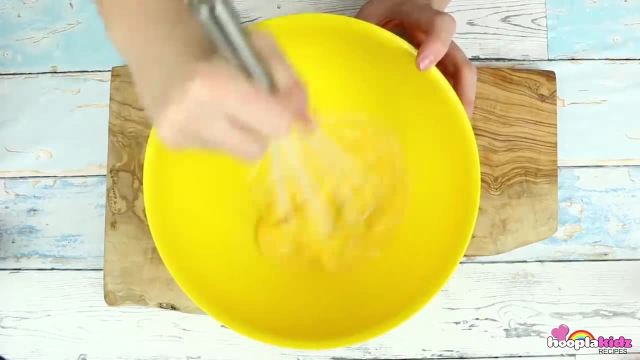 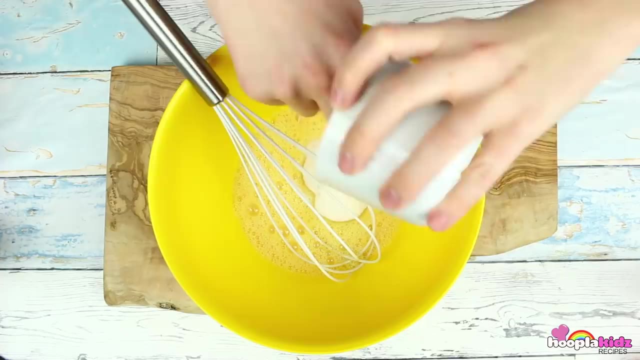 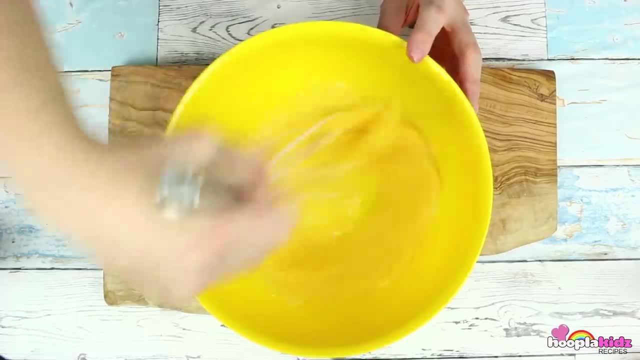 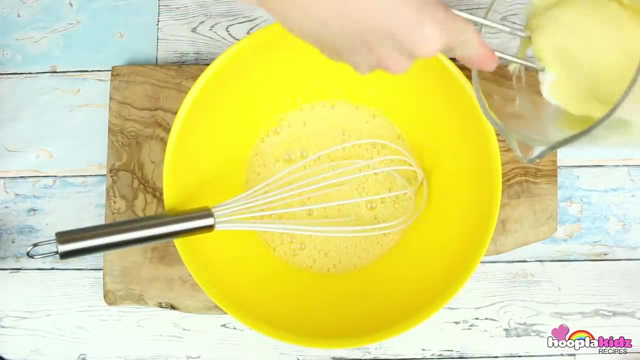 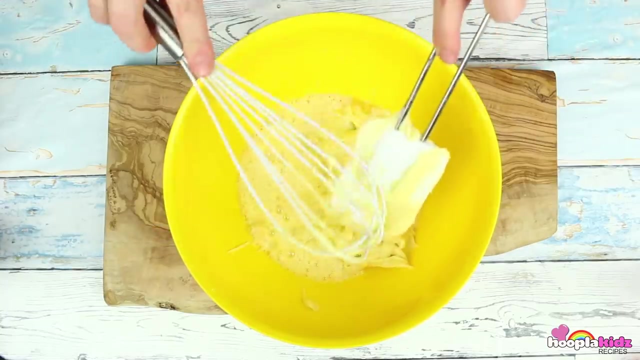 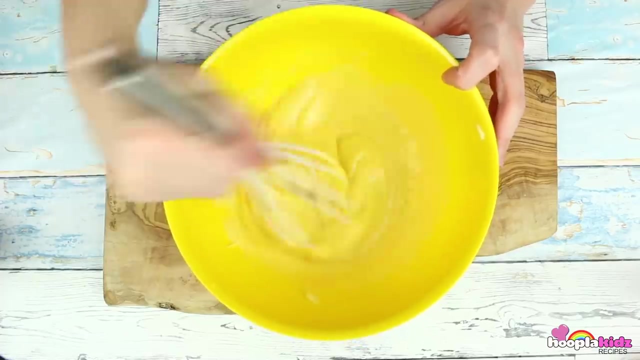 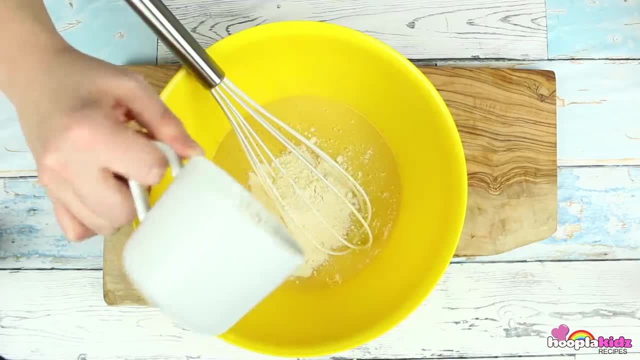 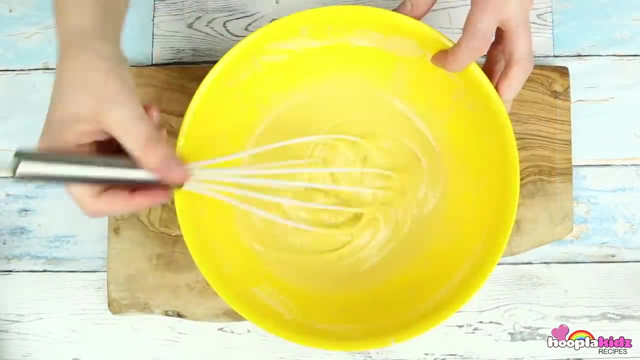 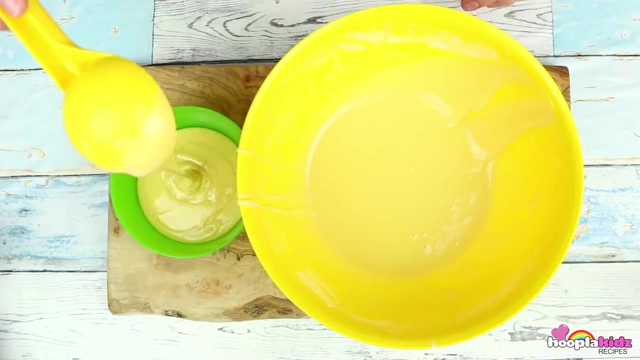 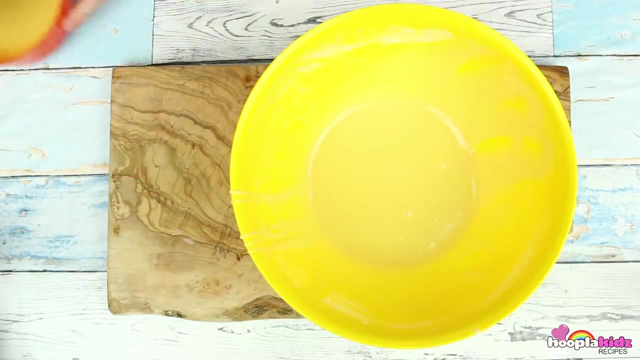 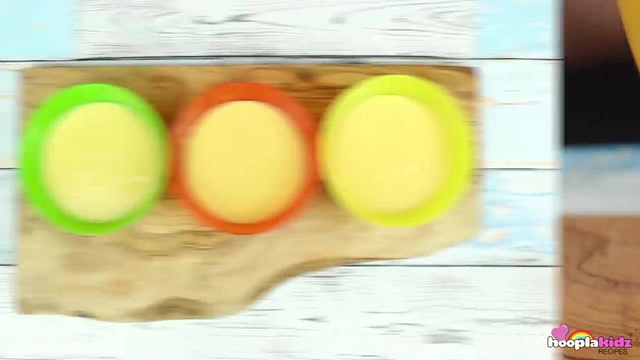 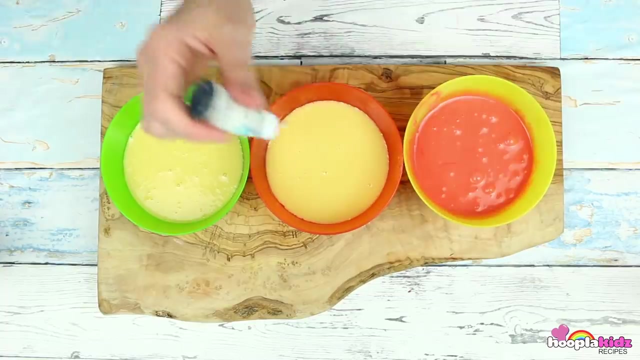 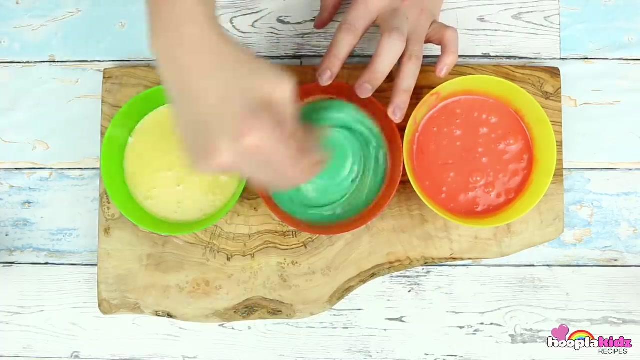 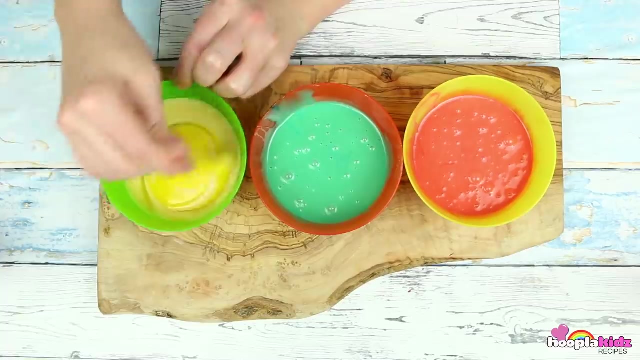 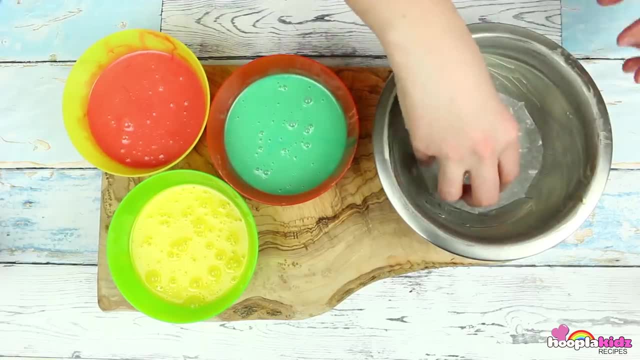 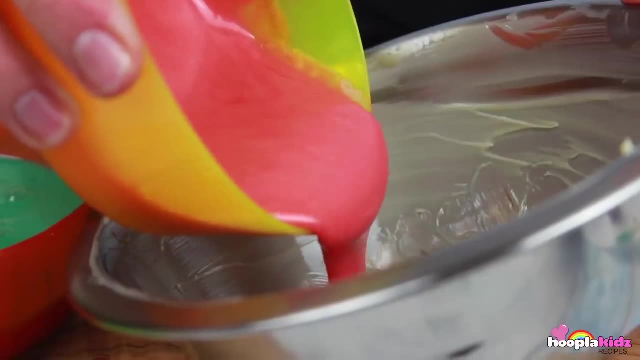 I have a cake tin that has been buttered and also has a bit of baking parchment at the bottom of it. Let's pour the mixture in, except we're going to try and cover only a third of the bottom each time we pour some mixture in. 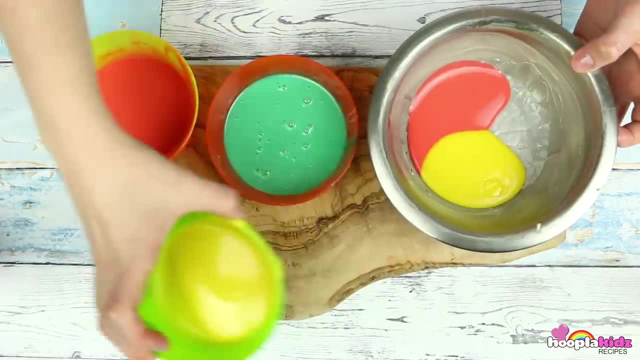 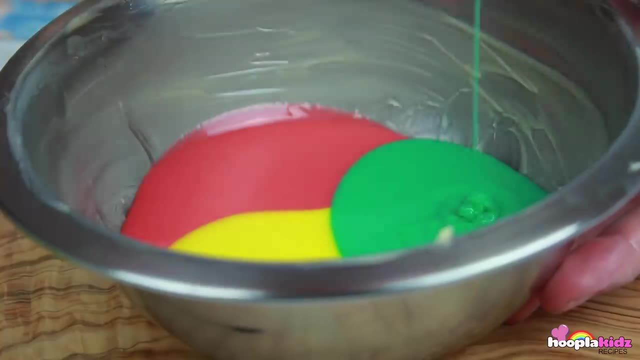 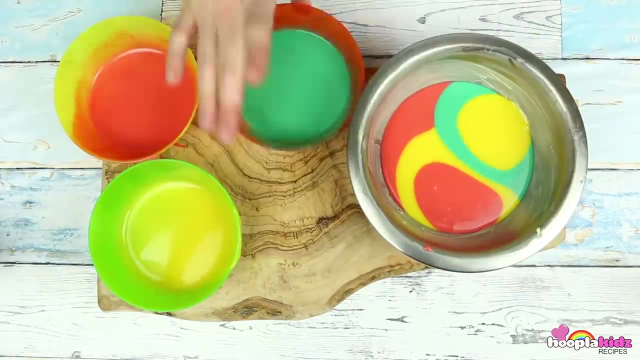 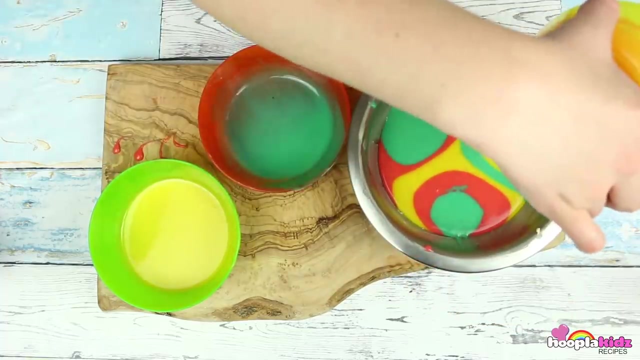 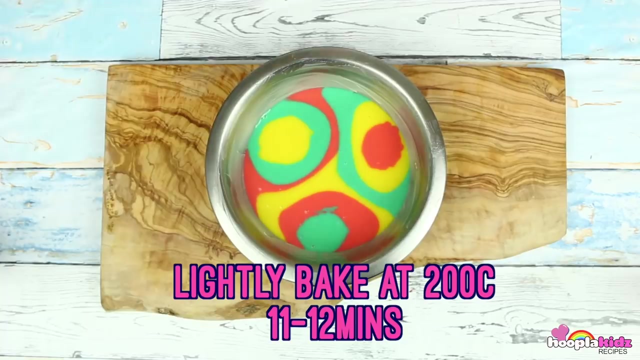 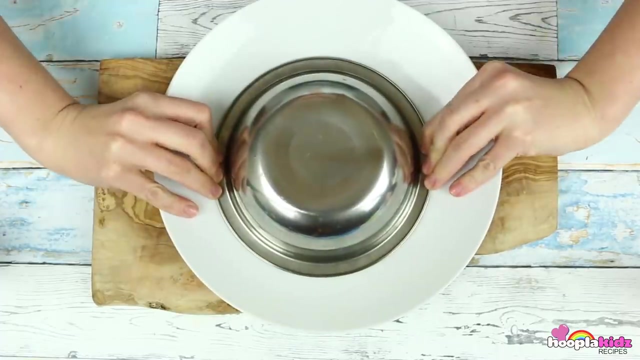 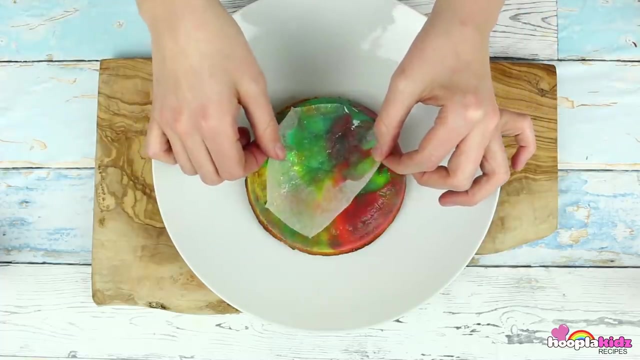 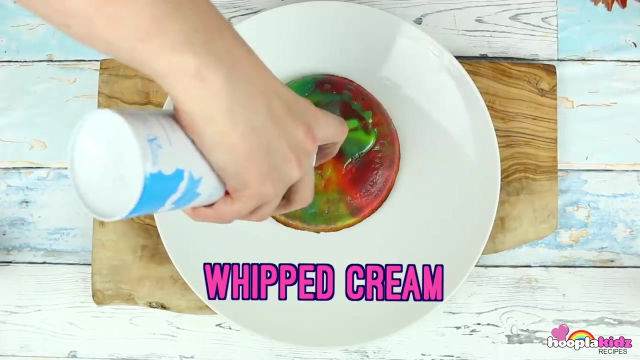 Let's create some fun patterns and keep pouring Looking good. Lightly bake that at 200 degrees for 11-12 minutes. Once you turn it over, you'll see, doesn't this look amazing. Peel off the baking paper and then top with whipped cream. 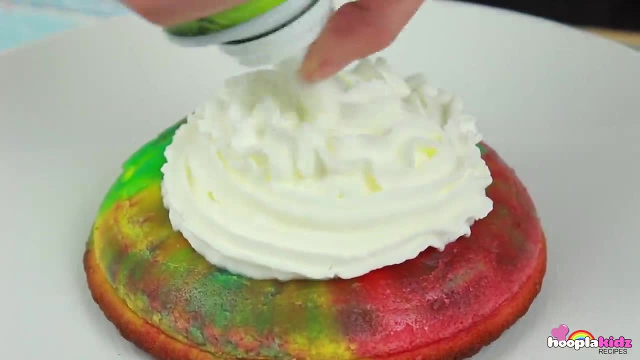 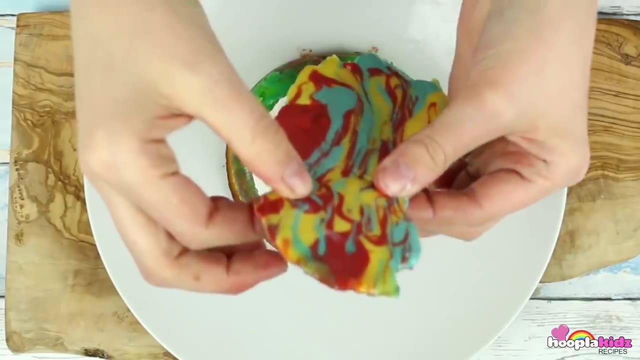 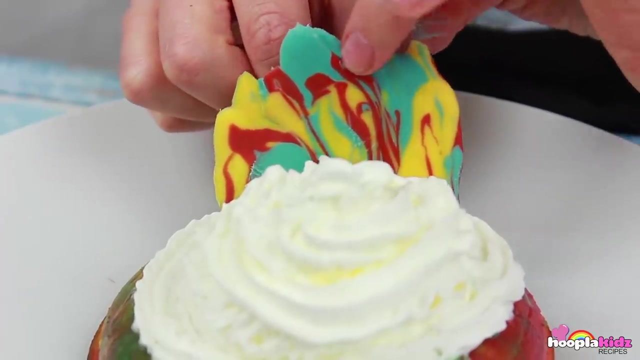 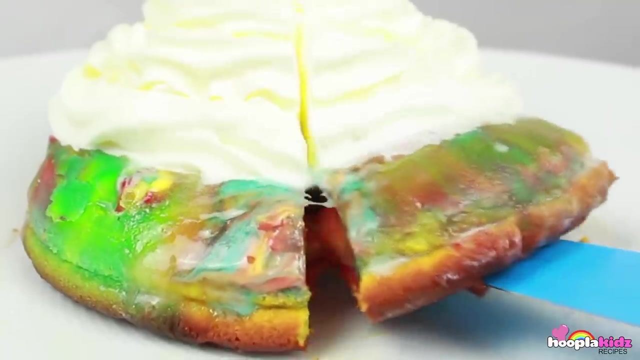 Finally, let's not forget our garnish. I'm adding that to the back, And there you have it. It's time to cut it in and eat. Look at that gooey centre. Doesn't that look delicious? I can't wait to eat it. 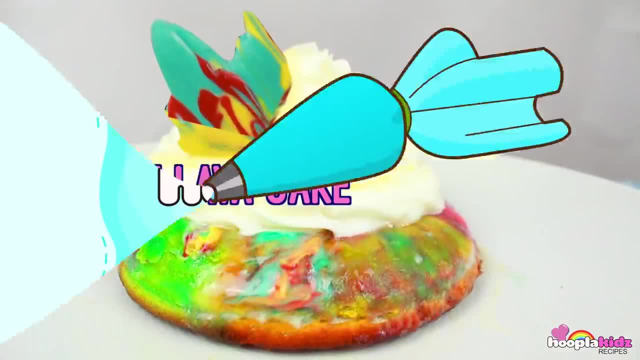 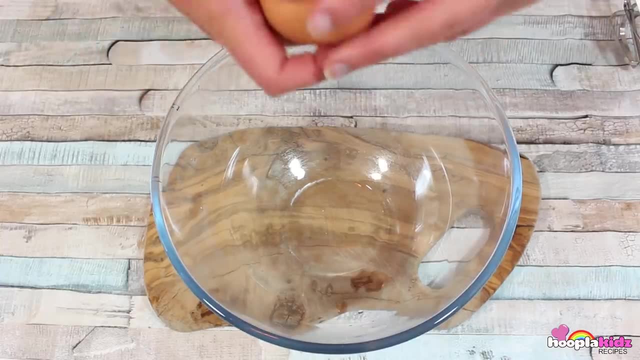 It's a rainbow lava cake, A giant Oreo cake. Doesn't this look incredible? So let's start off with some eggs. We're going to crack 14 into a bowl. That's right, 14 eggs. I'm then using my electric whisk to mix it all together. 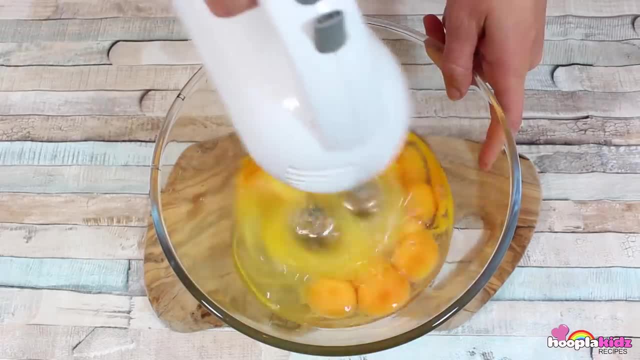 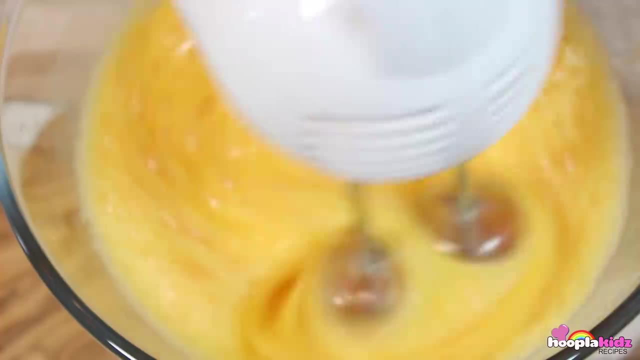 Once the eggs have been mixed in, I'm going to add the rest of the mixture. whisk to mix it all together. gradually, add 350 grams of sugar, mixing it as you go. this is gonna taste delicious. I'm also adding a pinch of salt and 210. 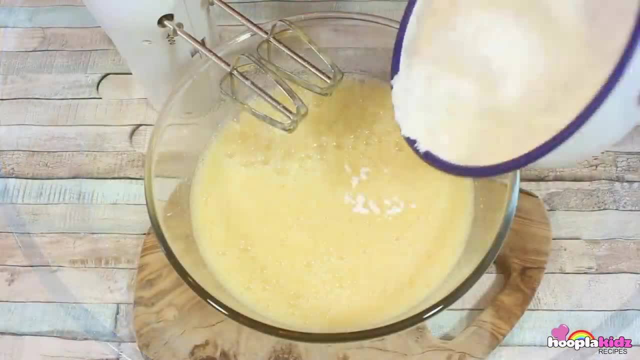 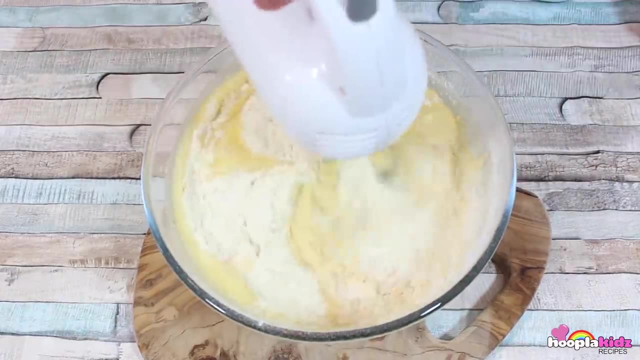 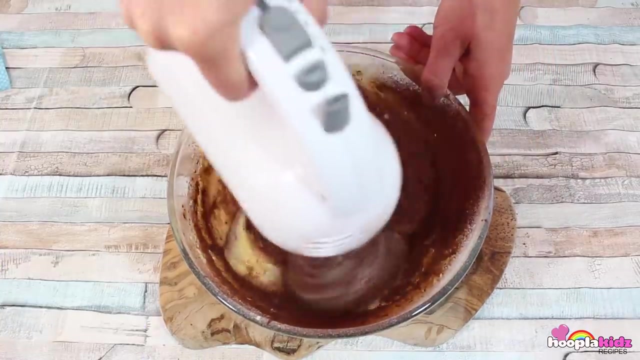 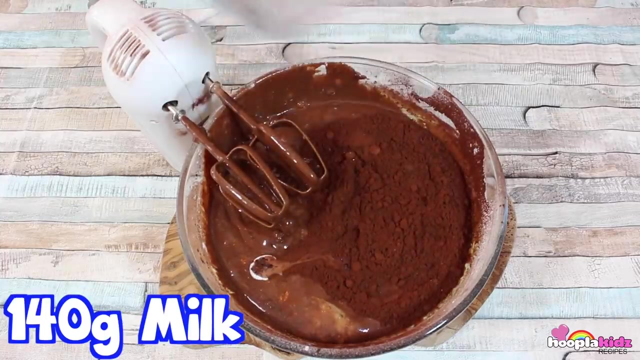 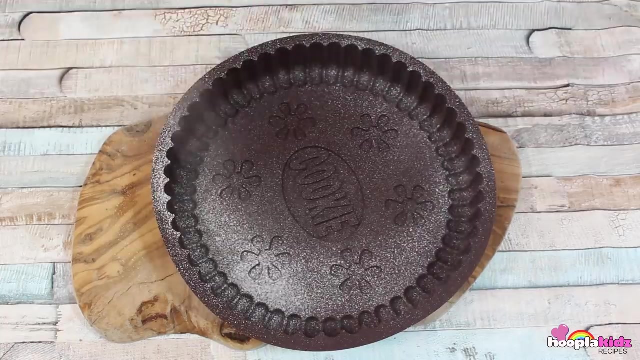 grams of vegetable oil. gradually add 530 grams of cake flour. make sure you mix it well. now I'm adding 170 grams of cocoa powder as well as 140 grams of milk. I'm I now have a giant cookie mould. I need two of them- and I'm greasing it with a spray. 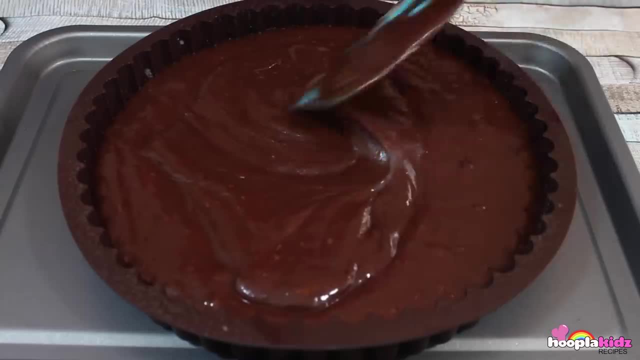 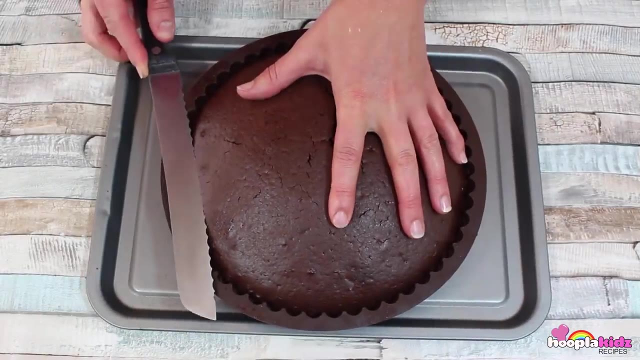 before adding half the mixture to each mould. The best type of mould to use is a silicon mould. We're going to bake for 40 minutes at 350 degrees Fahrenheit. Once that's cool, we're going to remove the top of each cake. You can't see it yet, but this is going to. 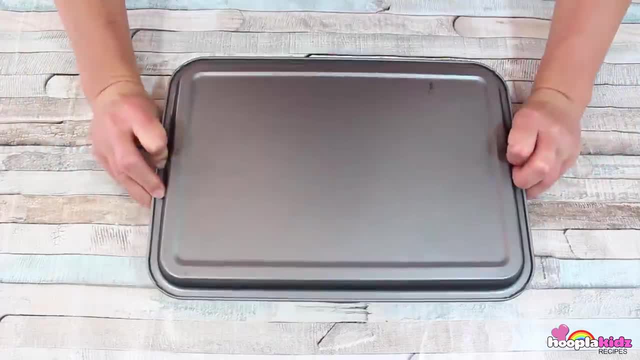 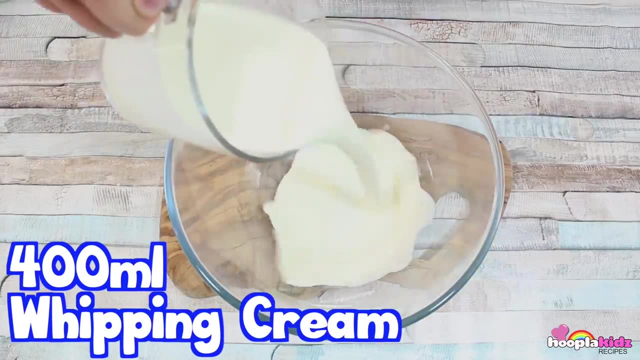 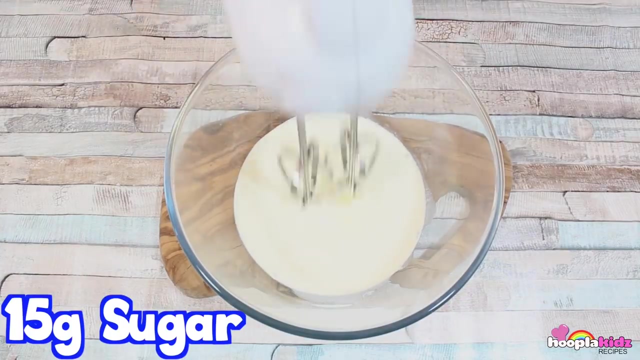 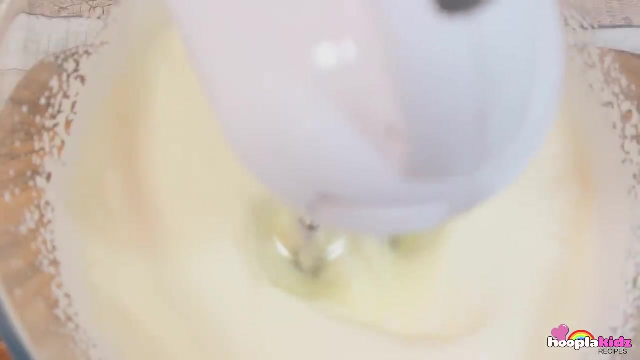 look amazing. Pop it onto a cooling rack and then remove the mould. Now let's make the middle. Add 400 mils of heavy whipping cream to a bowl. Also add 15 grams of sugar and give it a good whisk. We want to make the cream light and fluffy. It should be able. 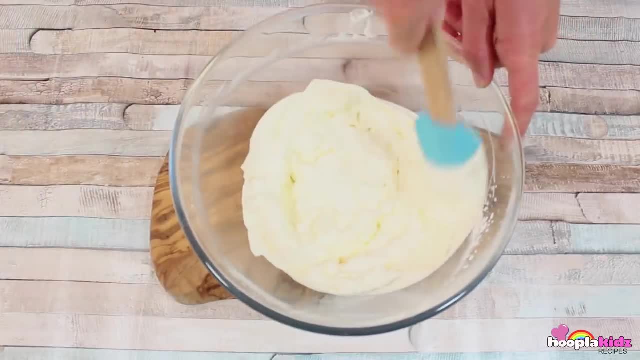 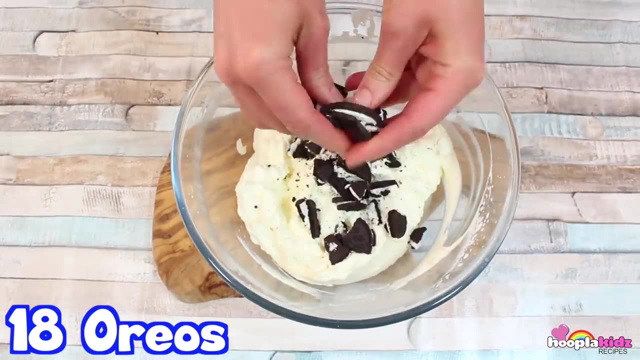 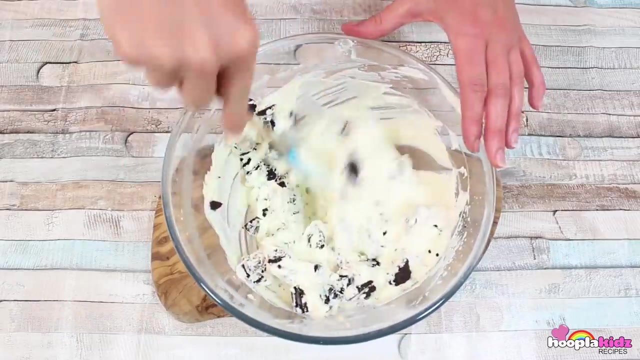 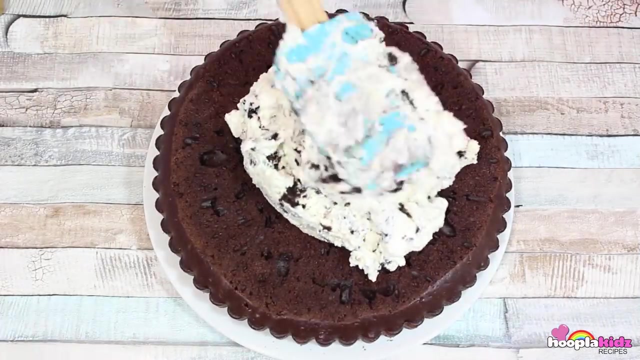 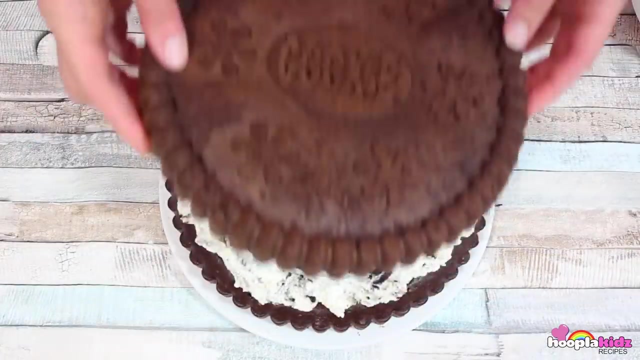 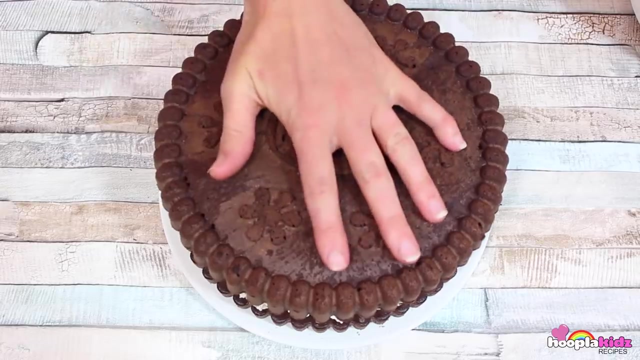 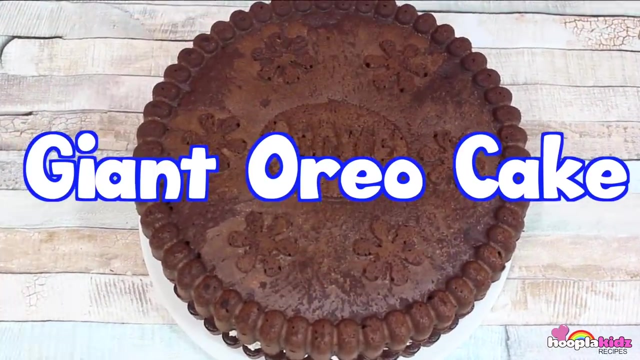 to stand up on its own with stiff peaks, Perfect. I'm crumbling 18 Oreos into the mixture. Give it a good stir. This cake is going to taste amazing. Spread the mixture onto one of the cookie cakes, Add the other to the top And there you have it- A giant Oreo cake. Doesn't that look amazing? And 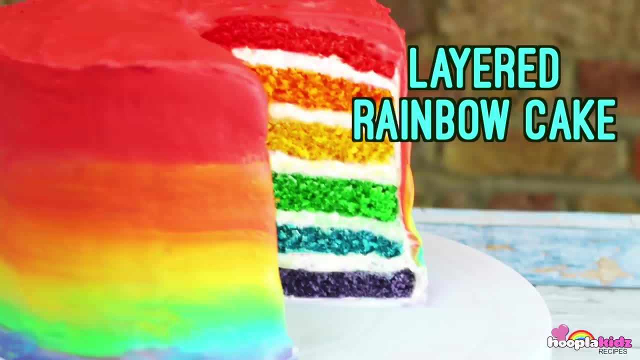 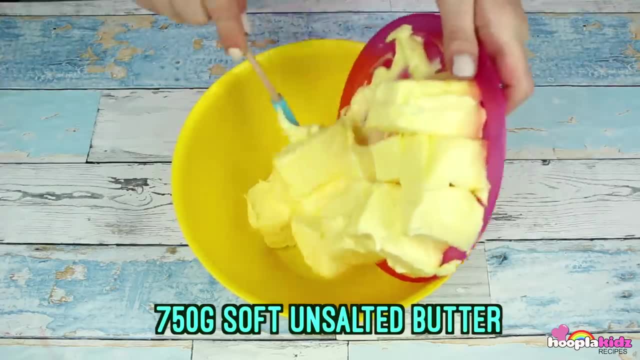 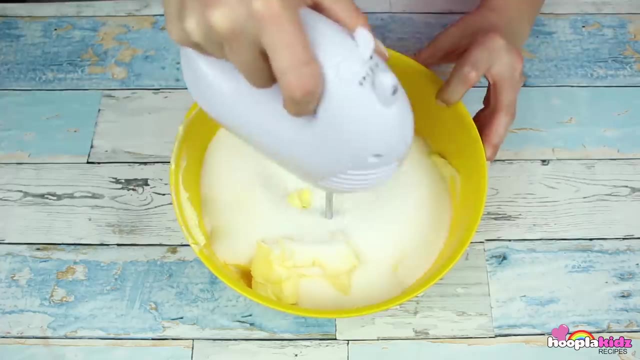 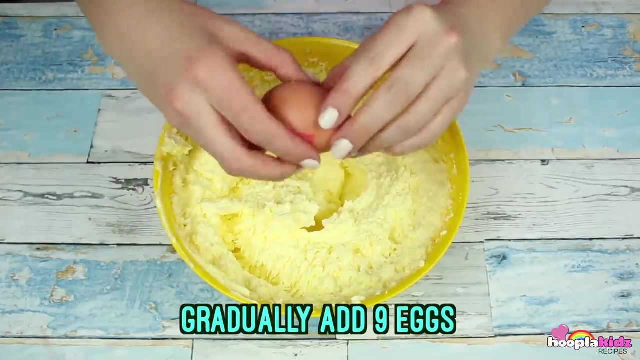 trust me, it tastes even better. A layered rainbow cake. This is fantastic. I love this recipe. So we're starting off with 750 grams of soft unsalted butter, And to this I'm adding 750 grams of caster sugar. Give it a good mix using your electric whisk. We don't want any lumps. We're going to gradually. 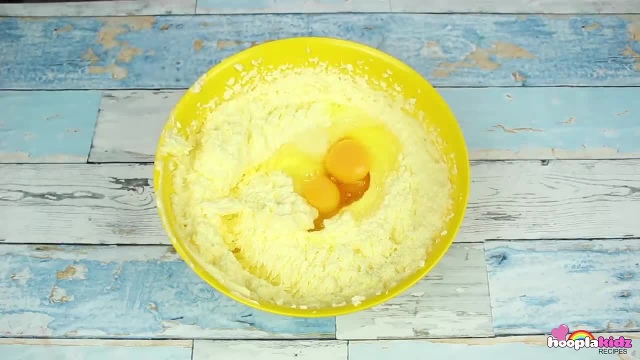 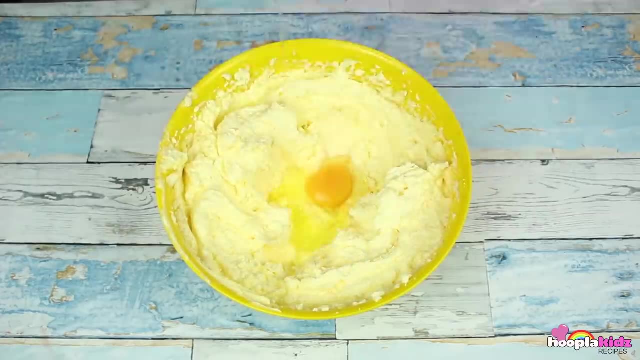 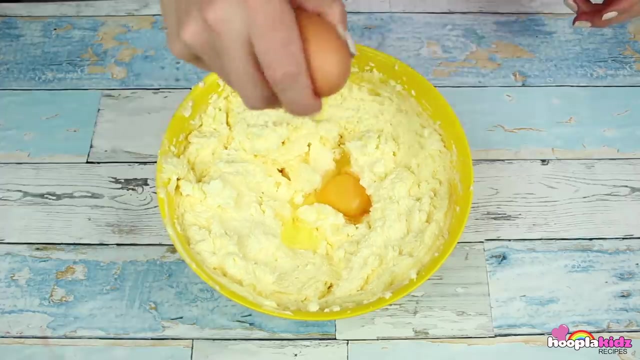 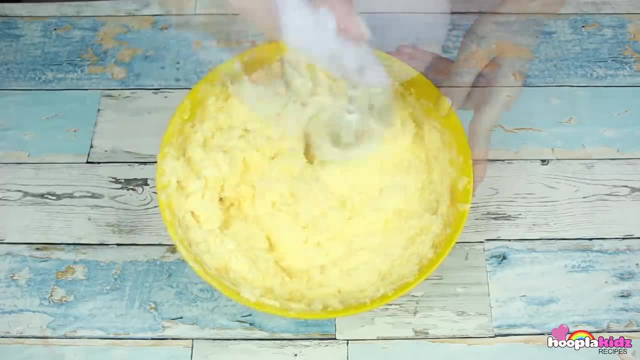 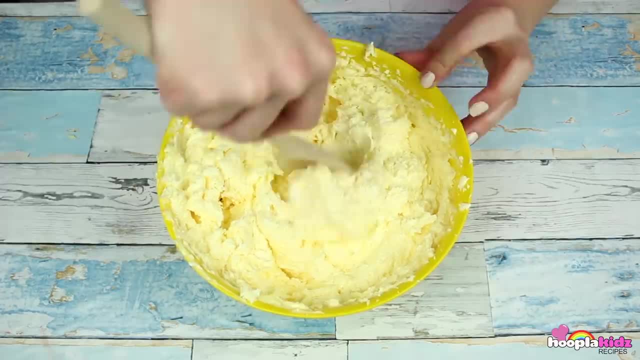 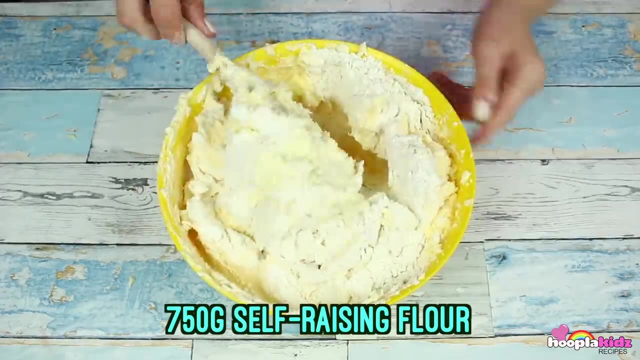 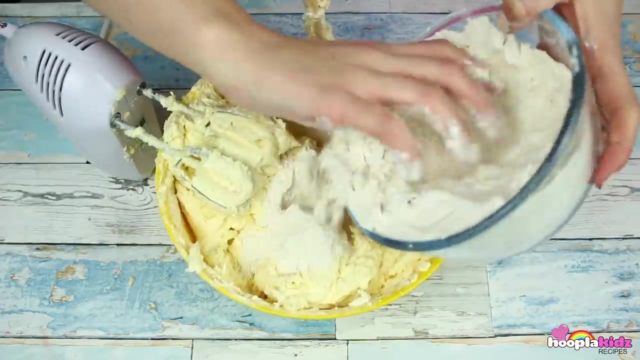 Perfect. It's light and fluffy, now- Just how we want it. I'm now going to add 750 grams of self raising flour, And I'm doing this bit by bit, Working it into the mixture. There's a lot of cake batter here. 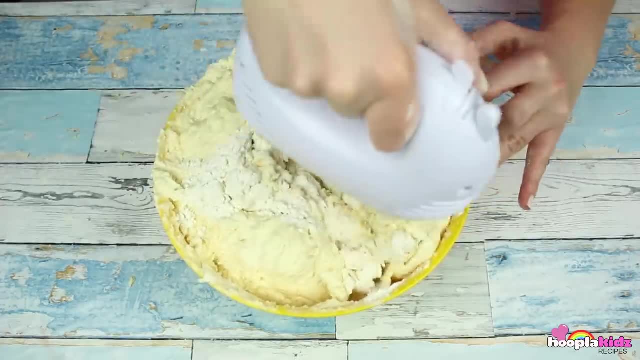 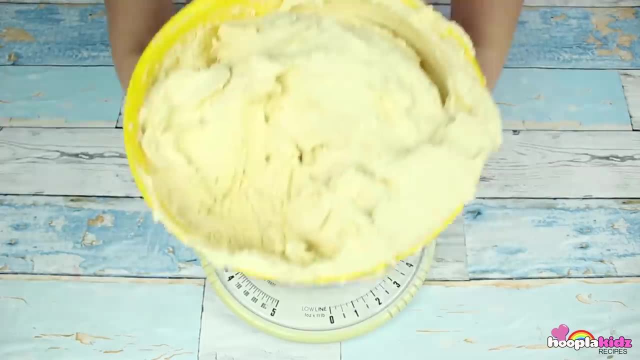 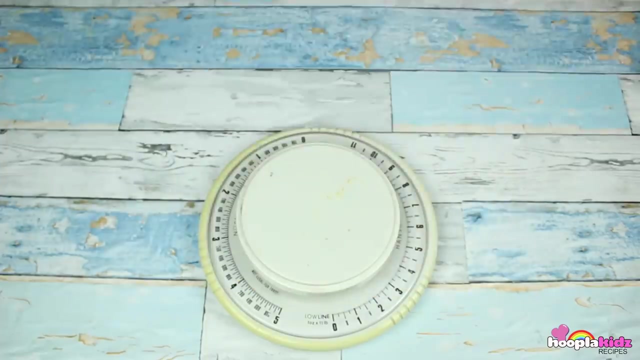 Keep adding And mixing, And adding and mixing- Wonderful. Now we're going to weigh the mixture. You need to make a note of the mixture's weight, Set that aside and prepare the food colouring. I have six different containers and I'm adding. 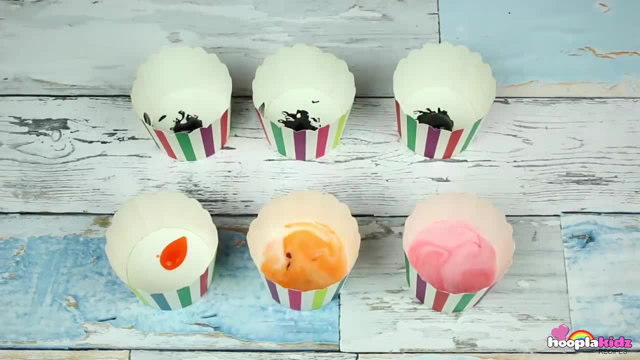 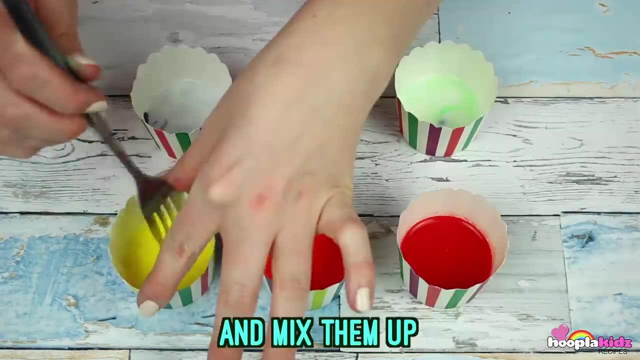 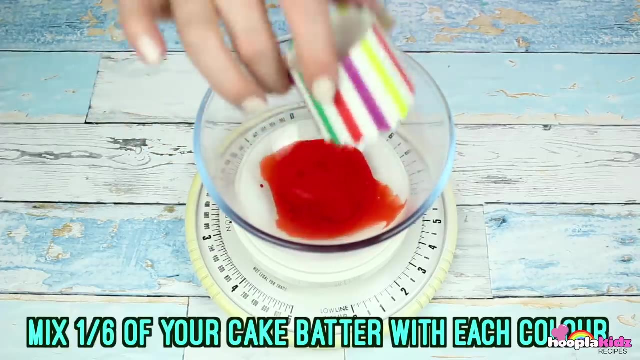 food colouring to each of them. I'm also adding a tablespoon of milk as well. This will help mix the dye into our cake base. Perfect, Now what we want to do is to add the food colouring. We're going to mix one sixth of. 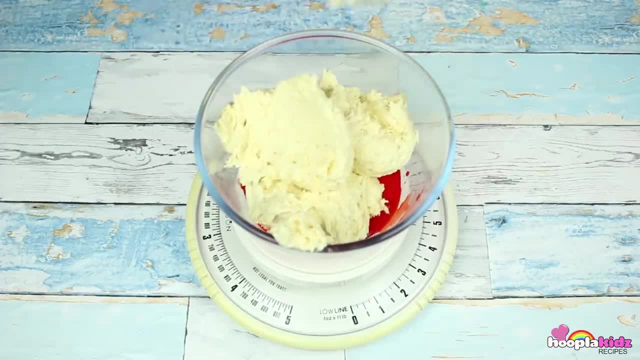 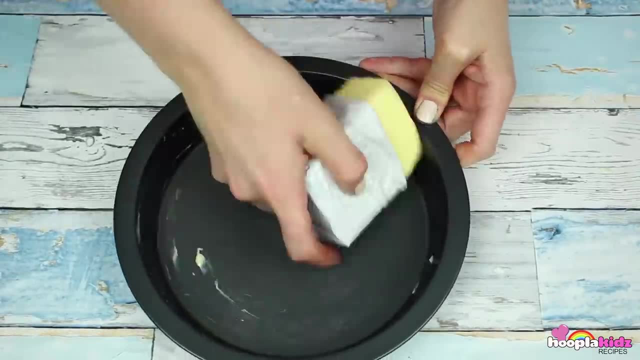 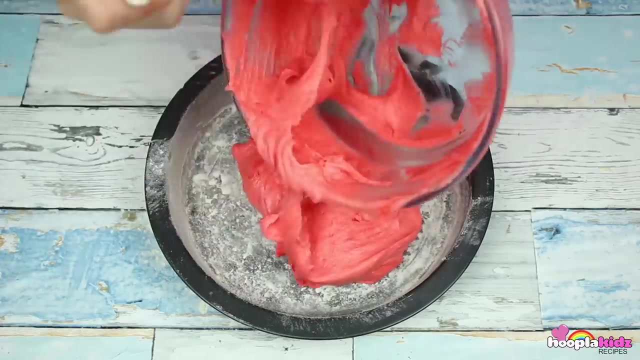 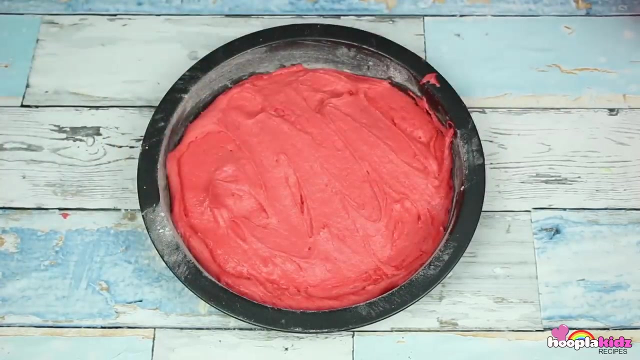 the cake batter with each colour. This is so we can have all the different layers. Next I'm greasing a small baking tray and then sprinkling some flour on top. Get rid of any excess and then pour the batter in. Make sure it spreads right to the edge. We're putting that in the oven at 170 degrees for. 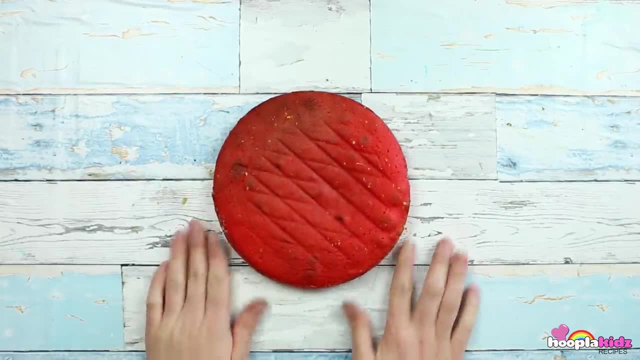 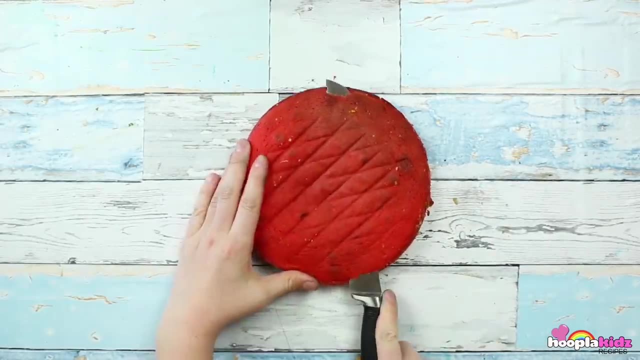 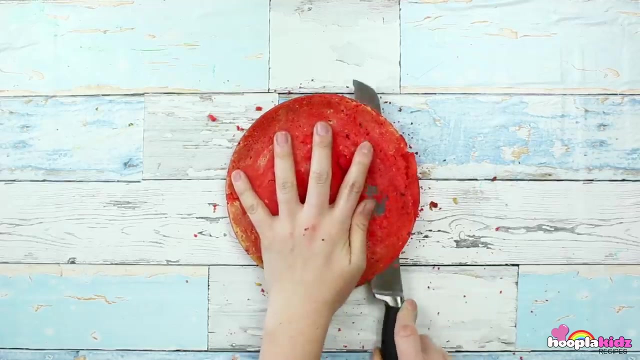 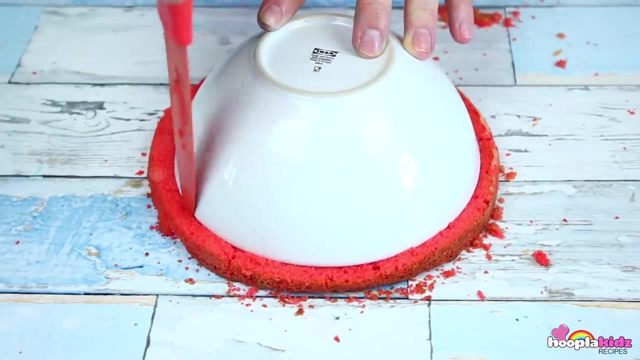 12 to 15 minutes. Perfect. Here are all our colours. Now I'm going to cut off the top of each of the cakes. This will make the colour super vibrant. We're going to use a bowl as a template. This is right next to each cake. We're also going to cut a little long circle, Just like. 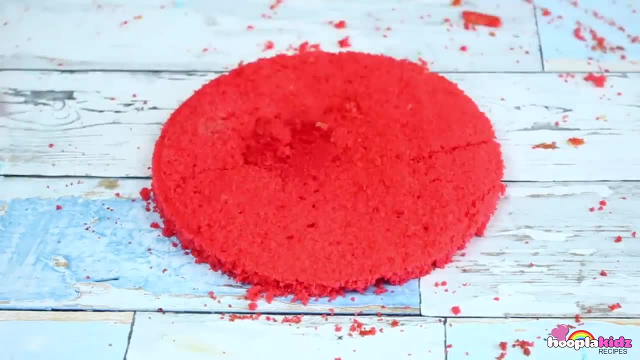 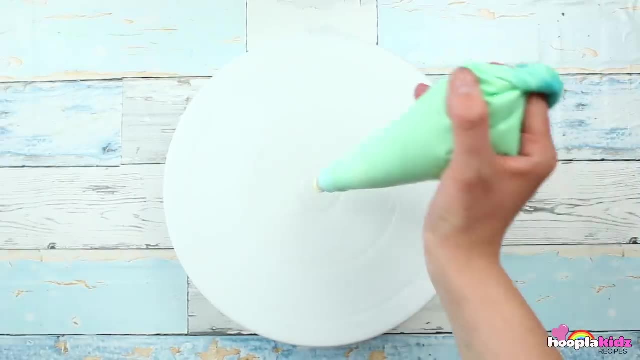 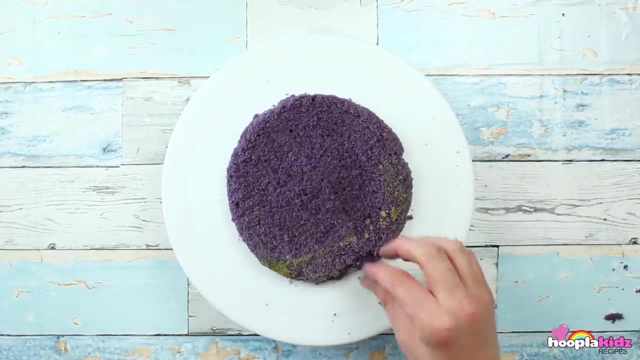 in our cake recipe, which is exactly the size we want. Voila Looking good, Don't? the colours look fantastic. Now it's time to layer them up. I'm using a little bit of icing as some glue- One dollop. 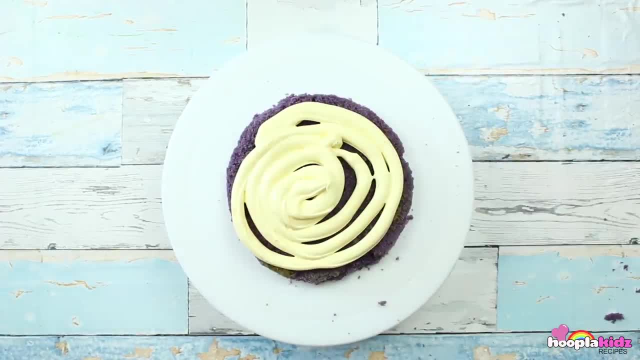 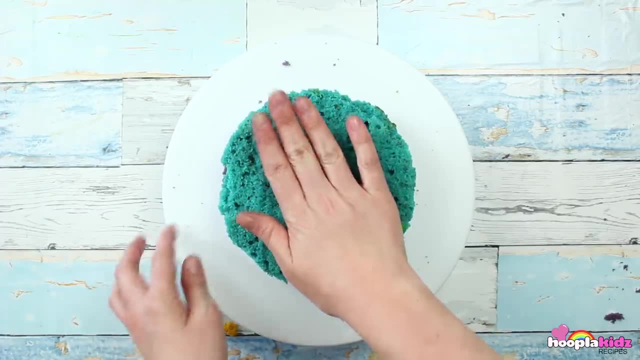 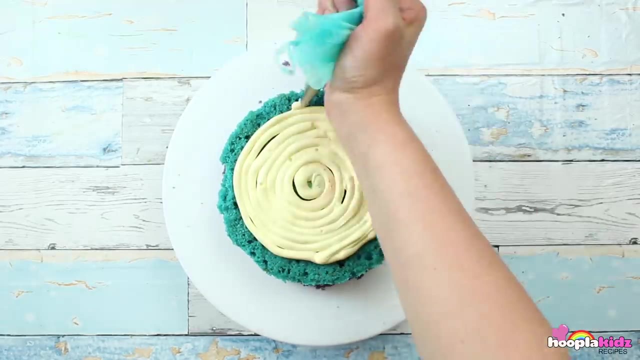 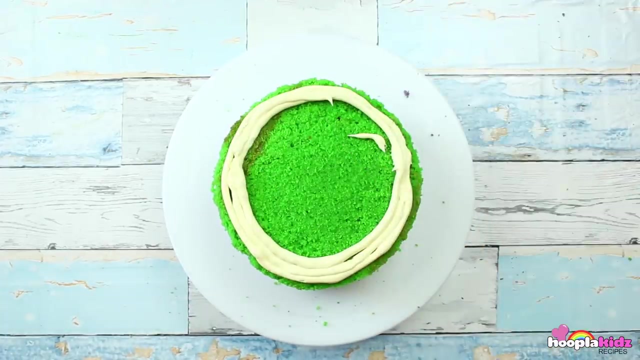 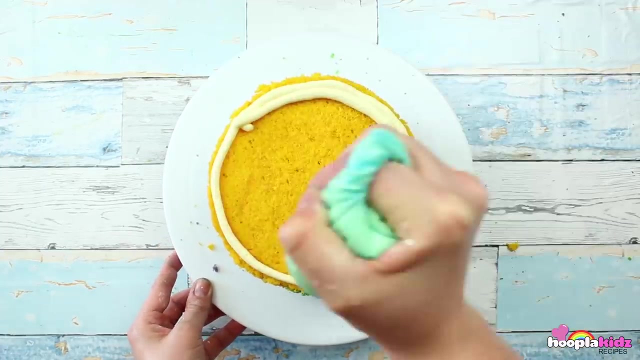 in the centre, and then I'm putting purple, And now I'm layering more buttercream frosting in between each of the colours. Next up is green, And we're repeating the process. Keep going. Yellow Looking good. Now we've got orange. 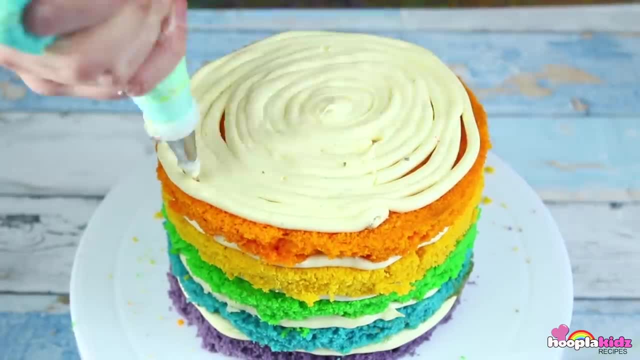 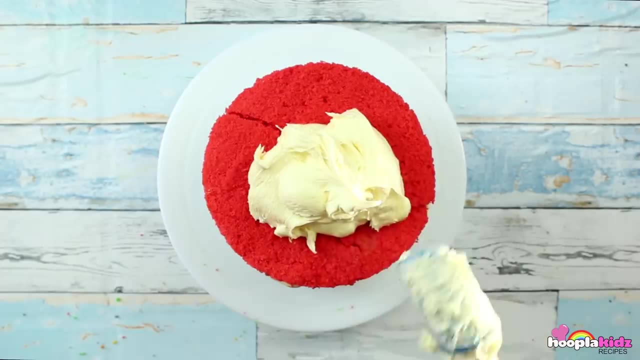 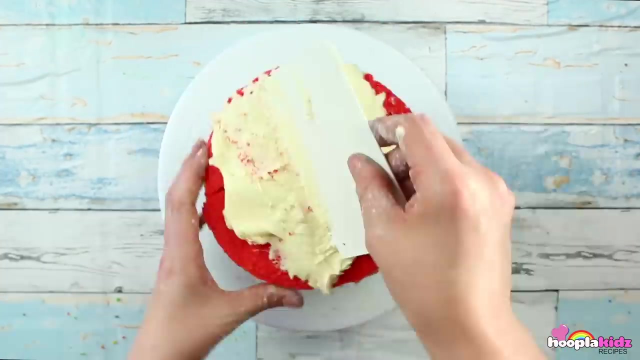 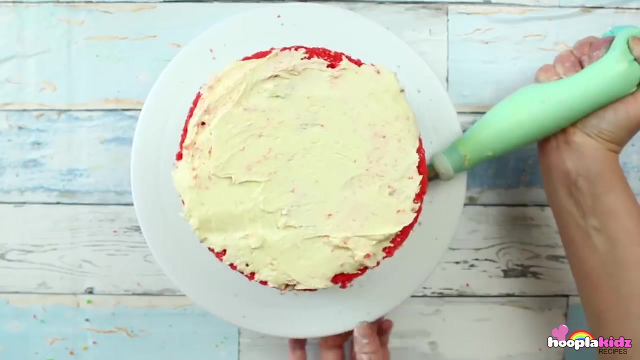 And finally, we're adding the top layer of red. I'm adding some more buttercream frosting over the entire cake and this is going to be the crumb coat. This will catch any of the crumbs. It means that when our top layer of icing is applied, it will be super smooth. 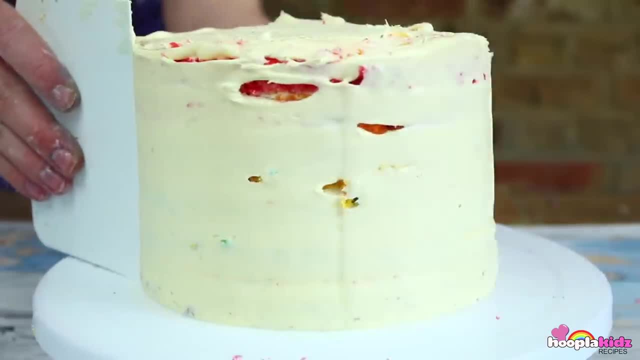 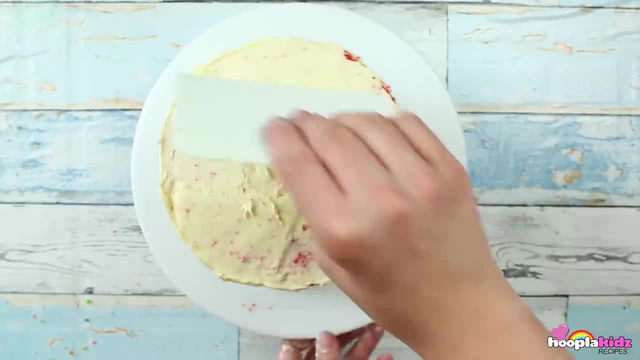 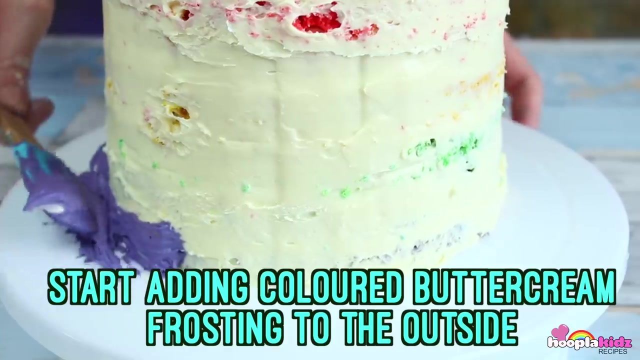 I'm using a cake scraper to press it all down on the side And the top Perfect. Now set that in the fridge for half an hour for the crumb coat to set. Next we're going to add the coloured buttercream frosting to the outside. 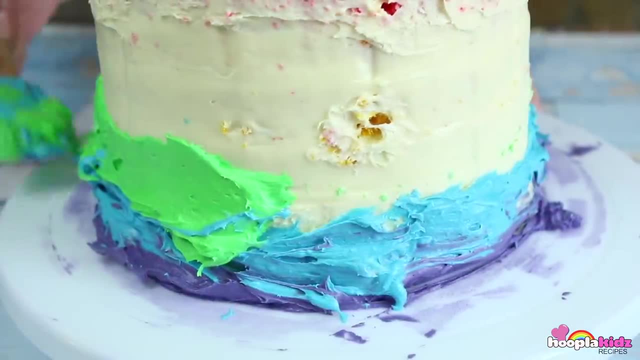 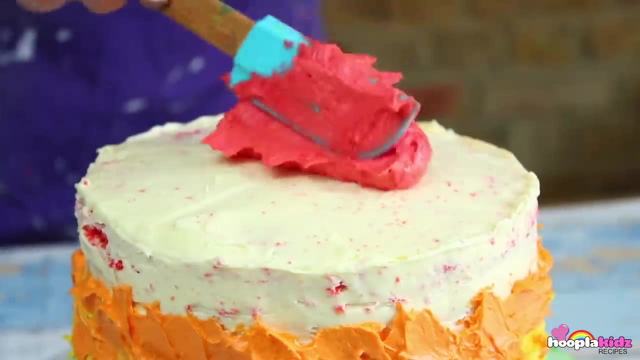 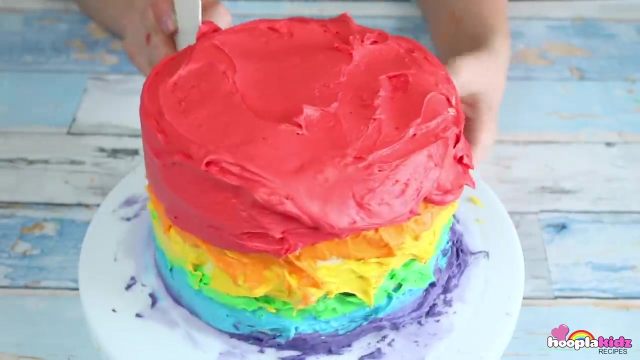 We're tiering this, It's going to create an awesome ombre effect. So start with purple. Then we've got blue, Green, Yellow, Orange And red. Red. goes on the top as well- Perfect. Now, this might look super messy, but once you start smoothing out the frosting, it's. 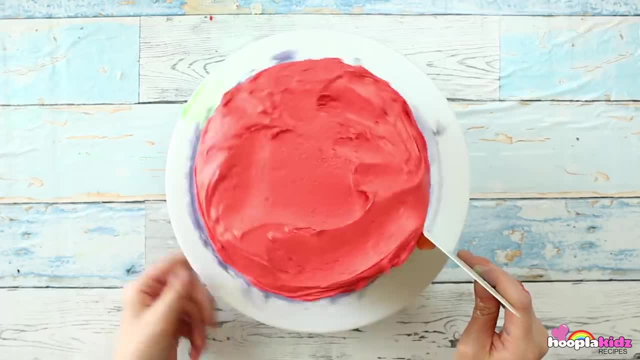 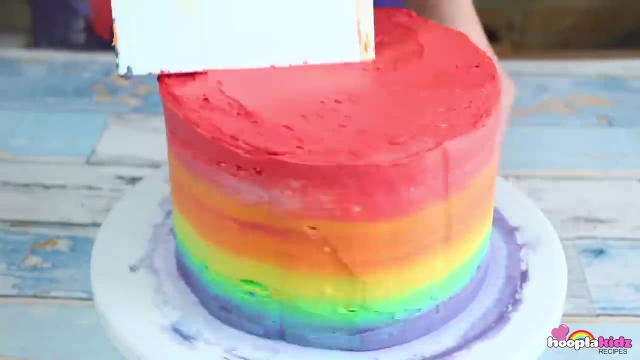 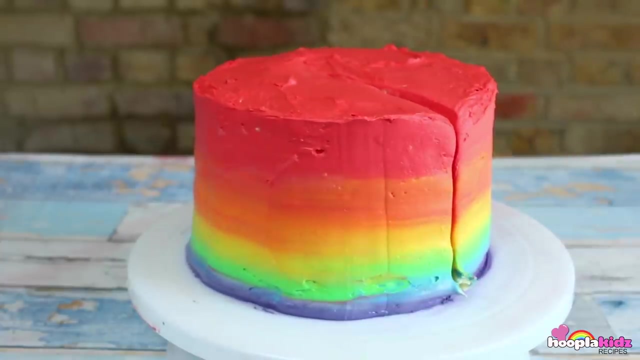 going to look amazing, Perfect. This creates an awesome ombre effect And it's rainbow. And there you have it: A perfect rainbow layered cake Moment of truth. Let's cut inside and have a look. We've got rainbow on the outside. 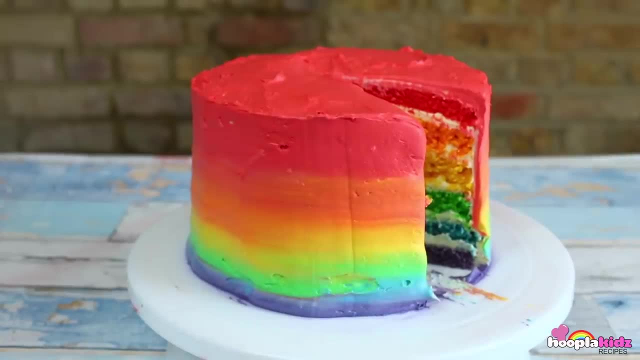 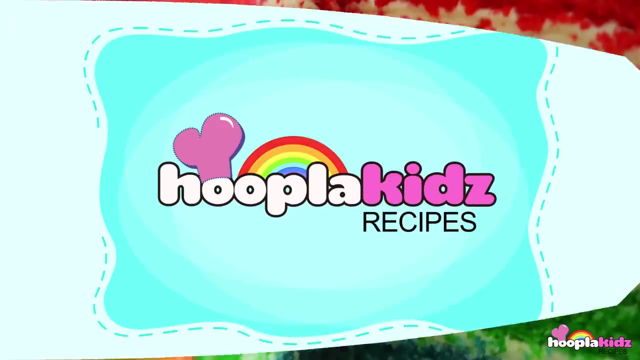 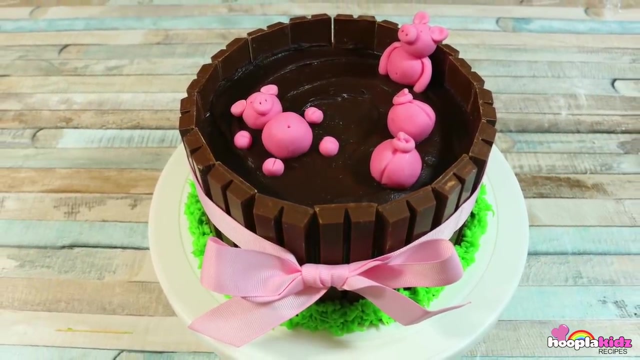 And voila Rainbow on the inside as well. Doesn't that look fantastic? There you have it: A rainbow layered cake. Pigs in mud cake. Doesn't that look awesome? It's lots of little pigs in some mud, So let's get started by making the pigs. 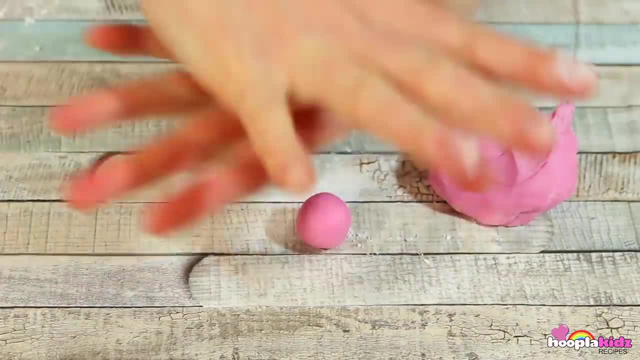 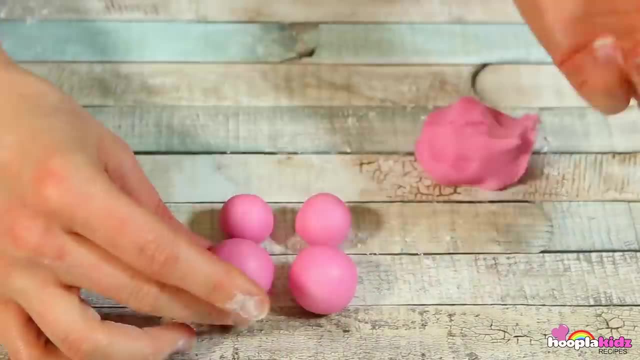 I'm using some light pink fondant icing And I'm rolling out some balls. These are going to form the bottom. These are going to form the body and the heads of the little pigs. We've got some bigger balls for the body and some smaller balls for the head. 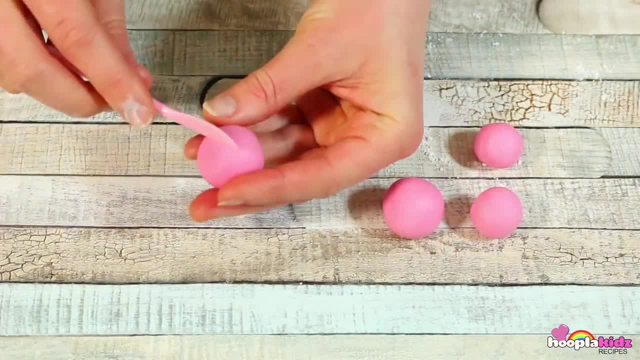 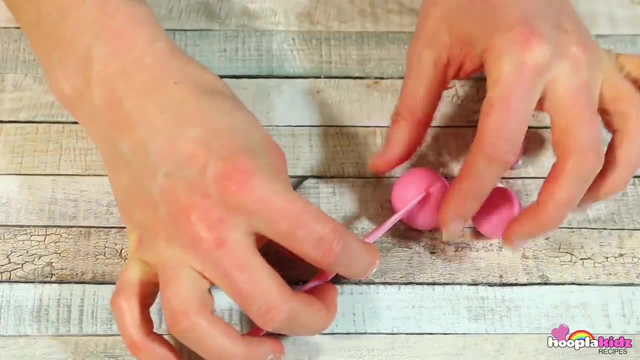 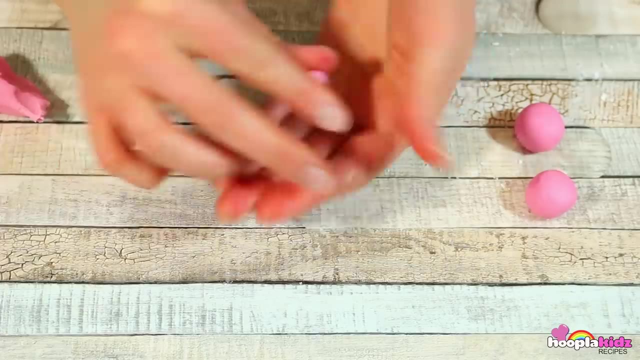 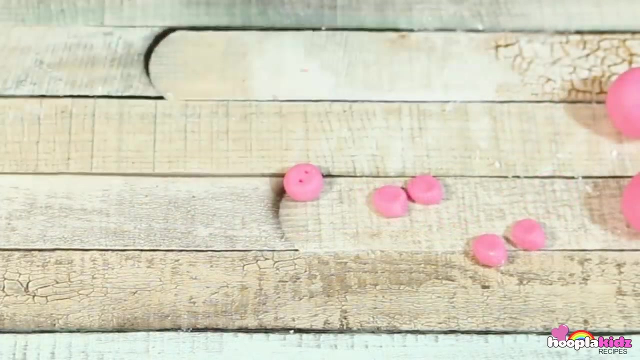 Perfect. Now I'm taking some tools. I'm going to add some detail. These are going to look super cute. Set the big balls aside. We're now making some smaller balls. These are going to be two ears and a snout. 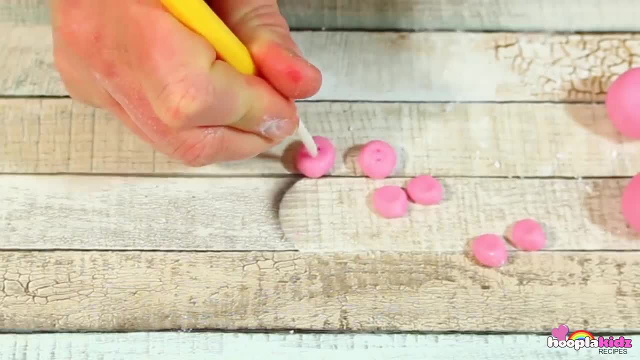 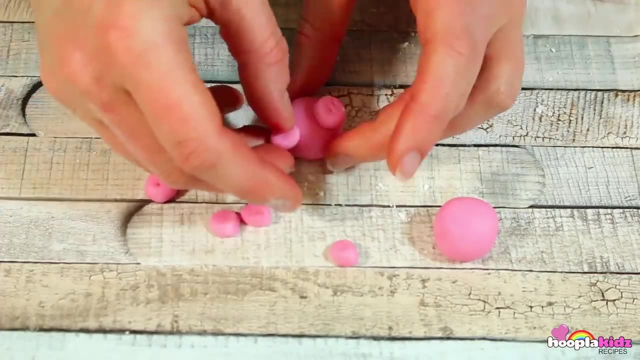 Press down the ball that's going to be the snout. Now add two dots. using a tool, Using a little bit of water, I'm attaching the two ears and the snout to one of our smaller balls. The water acts like glue. 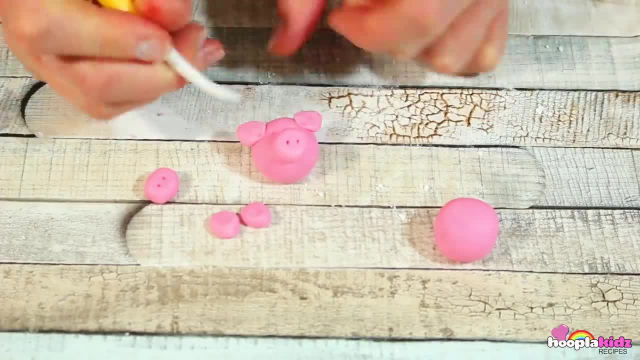 Isn't that cool. I'm adding some more detail: The eyes And shaping the ears using a tool as well. These are going to be two ears and a snout. Press down the ball. that's going to be the snout. These are going to be two better parts to it. 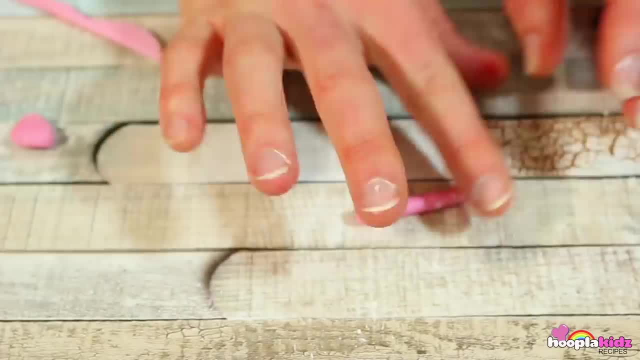 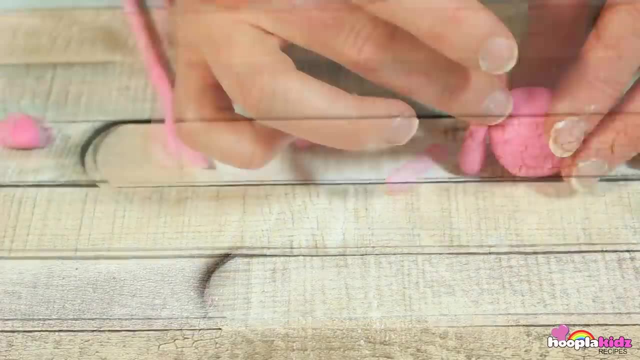 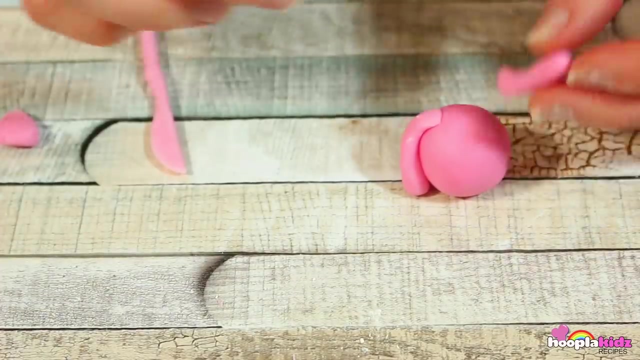 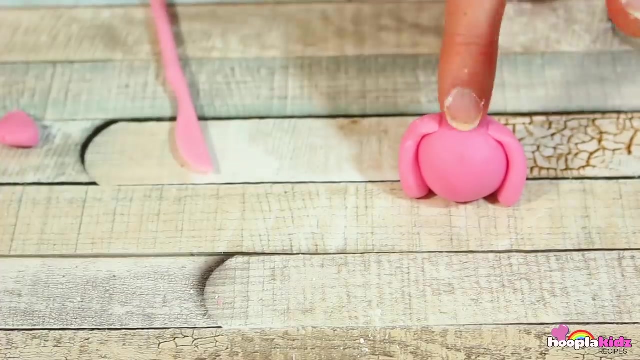 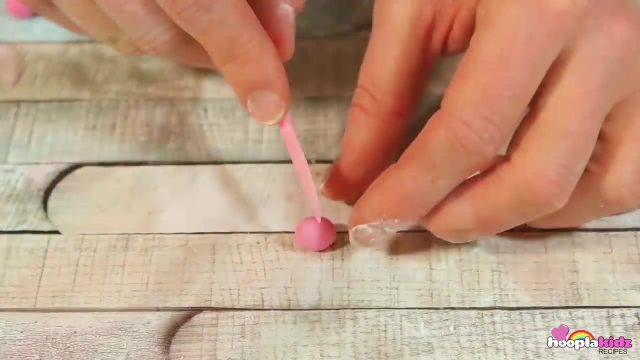 I've got two long sausage shapes that I'm using for arms. Let's add some. Just put them on one of the bigger balls And then stick the head on. Here we go, They're got to be over here. Perfect. Now I'm going to make some pig trotters. I'm rolling a ball shape and then I'm pressing. 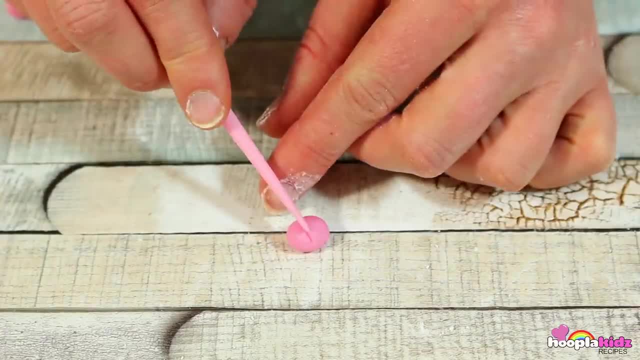 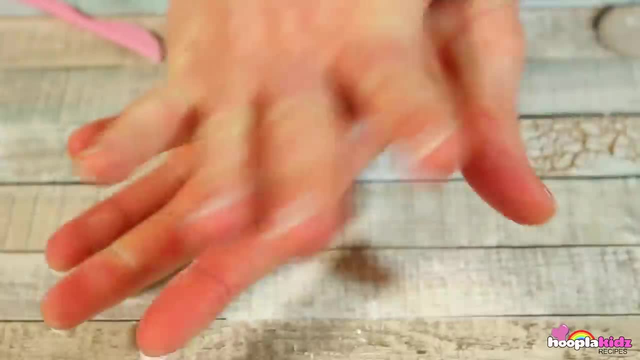 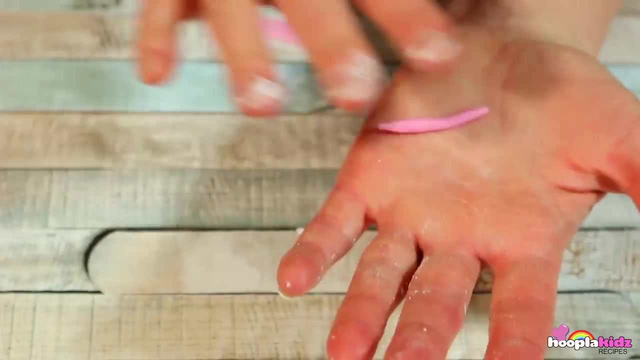 it using one of my tools. This creates an indent. It's going to look like cute little pig trotters. Perfect, Now it's time to make some curly pig tails. Roll the fondant icing into a thin sausage shape. Now it's time to shape it. We want. 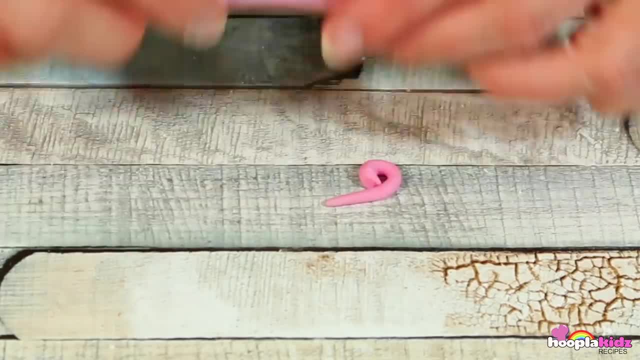 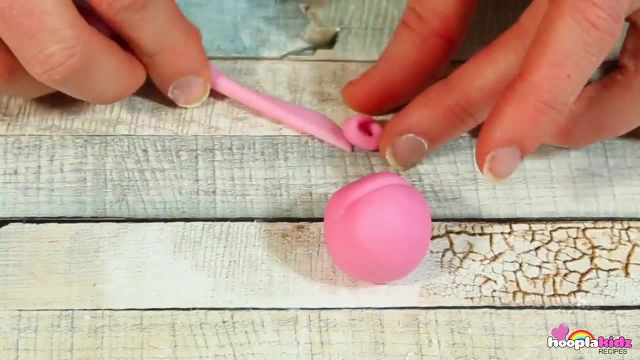 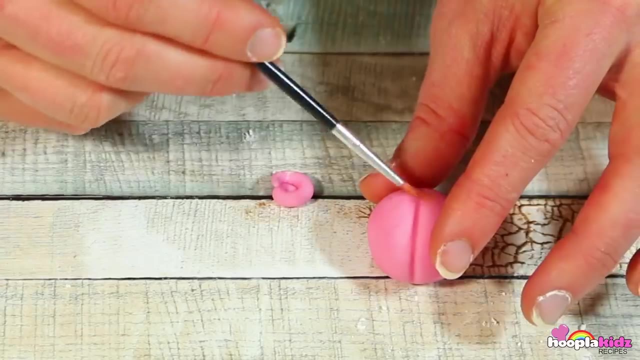 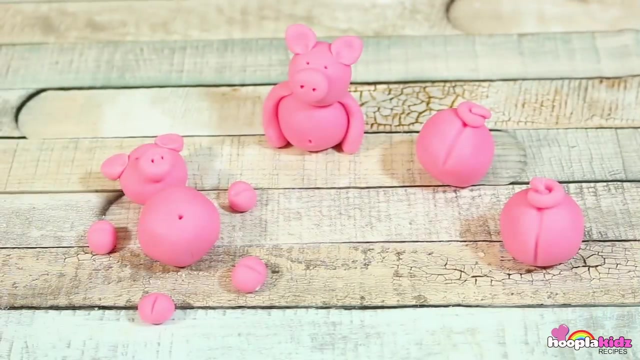 a curly, cute little tail. Use some water to attach it to the back of one of our pigs. Repeat that process. Looking good, Our pigs are starting to come together, Don't they look amazing? These are all the elements. Now, it doesn't matter that we don't have full. 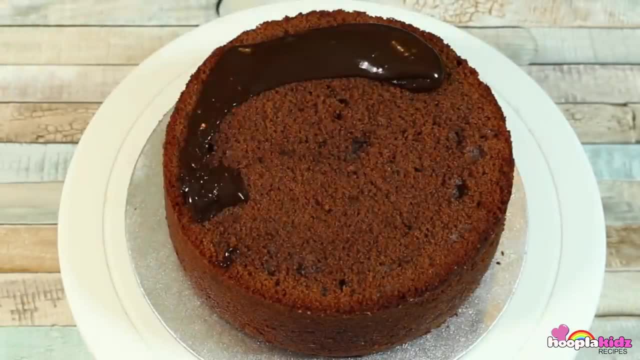 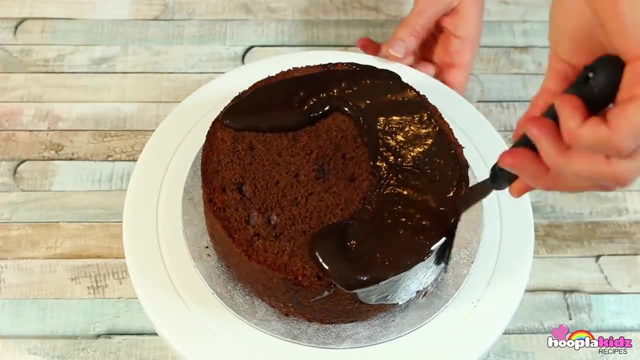 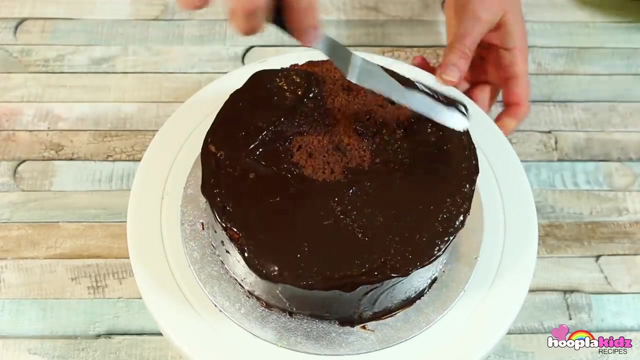 pigs because they're going to look amazing. Now they're going to be bathing in the mud. I have a chocolate cake and I'm covering it in chocolate icing. We want it to be goopy chocolate icing, because this looks like mud, Doesn't it look great? Smooth it down using a spatula. 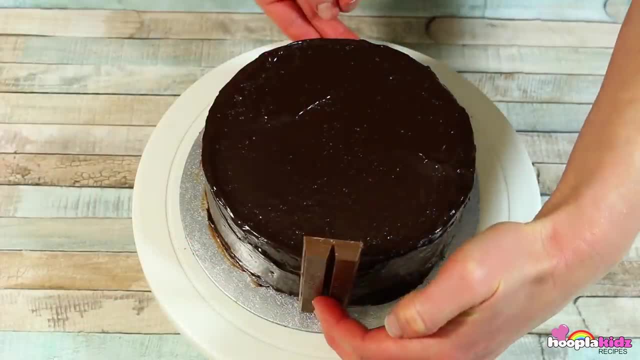 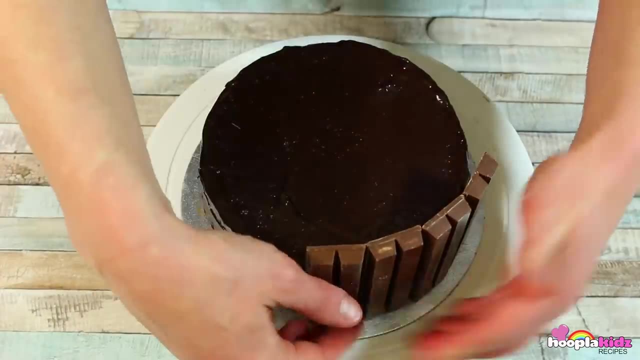 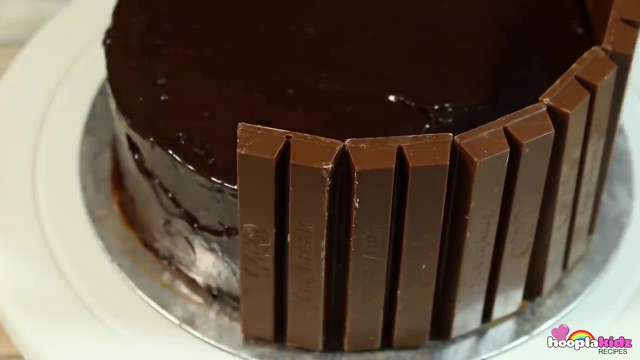 I'm now making the edge of the mud swimming pool. I'm using Kit Kats to do this and I'm simply sticking Kit Kats all the way around. the outside of the cake Looks great. This gives the impression that it's a mud filled swimming pool. 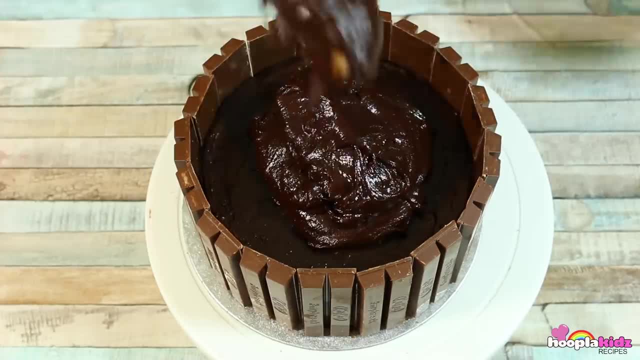 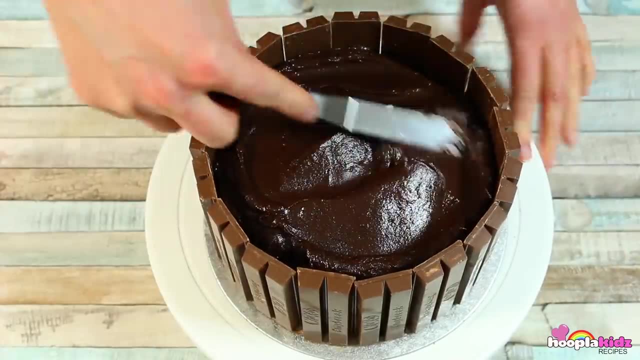 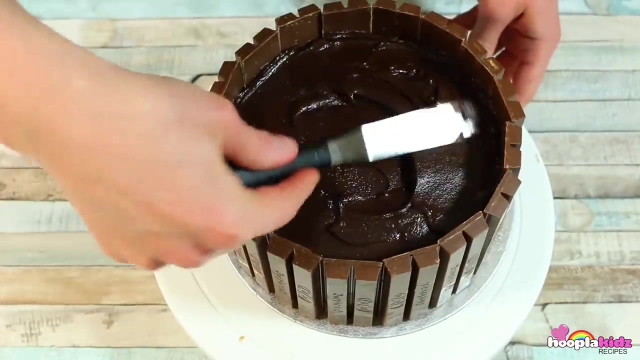 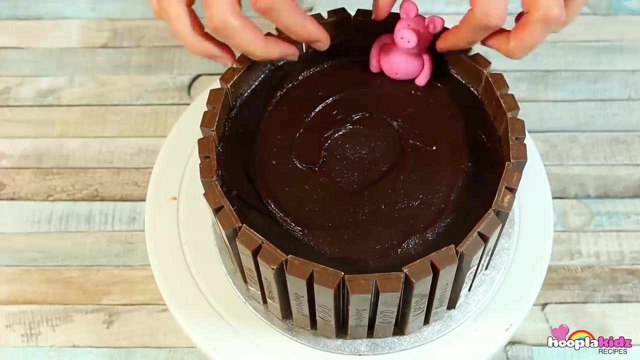 Let's add some more chocolate icing just for good measure. Delicious, Spread it right to the edge. Yum, This is going to look great and taste great. Now we just need to put our pigs in there. Let's sit one on top. You can't see the bottom. 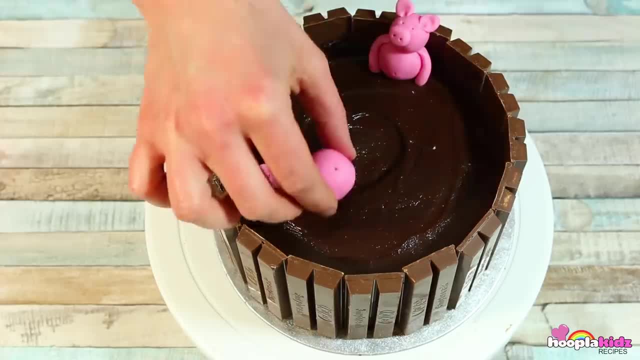 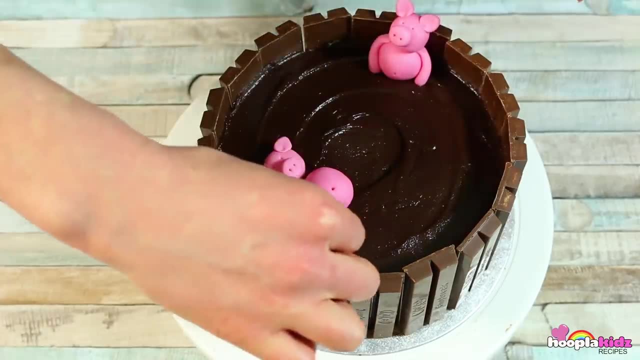 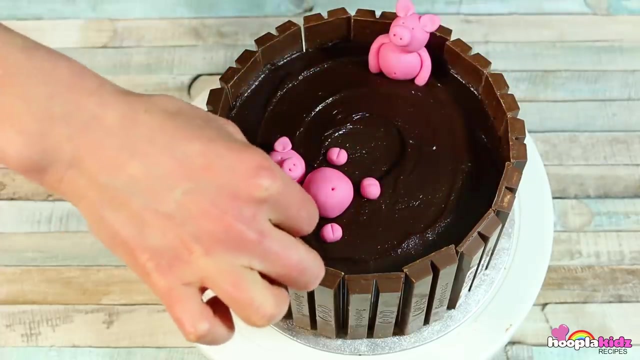 half because it's in the mud. This one's floating, so we've got a tummy poking out, Super cute. We're also going to add the feet, The little pig trotters And some hands. That looks great. It looks like he's part submerged. Now I'm adding two tails, Little bums and a little. 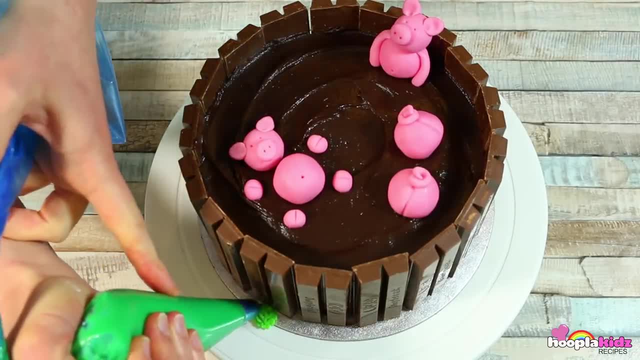 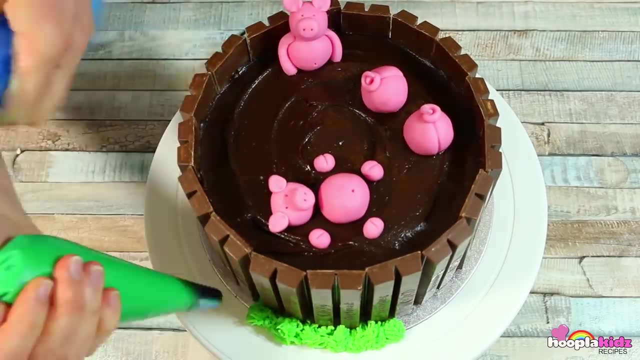 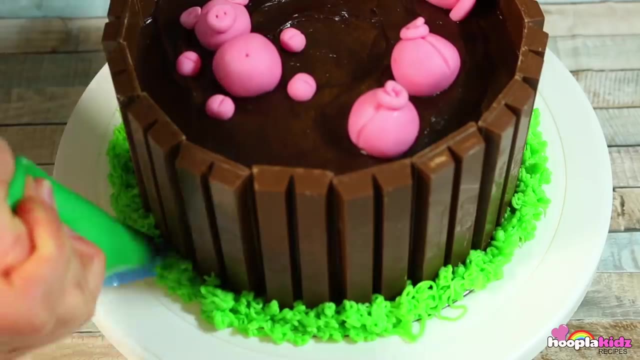 bum up in the air. Now I've finished putting the pigs in place, I'm going to use some green icing to decorate around the bottom of the fence. This looks like grass, Doesn't that look fun? Perfect. Finish it off with a ribbon around the entire thing. 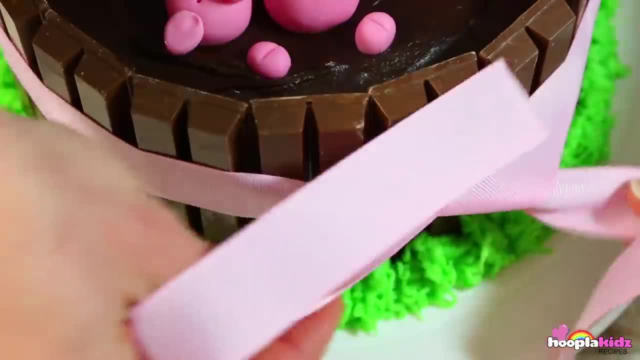 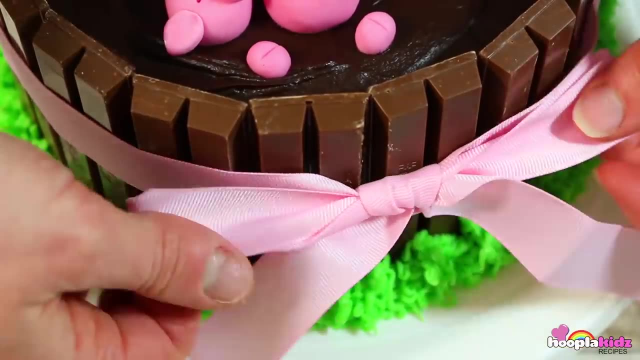 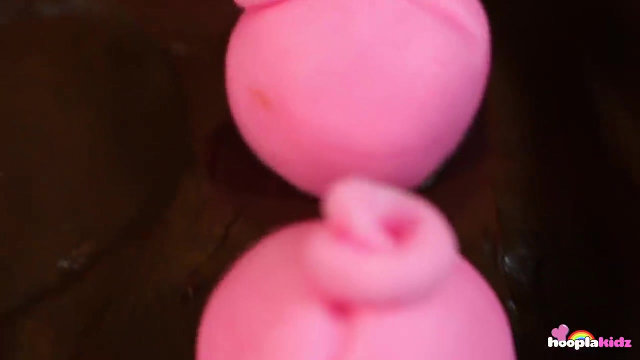 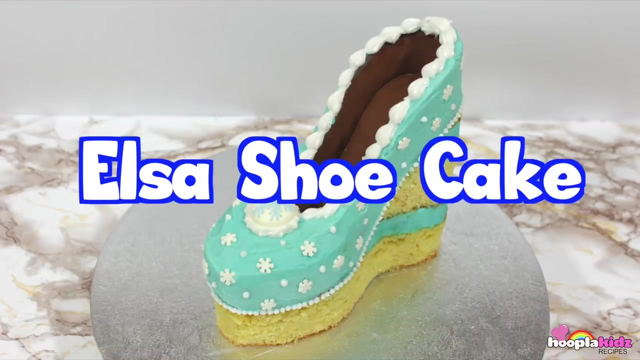 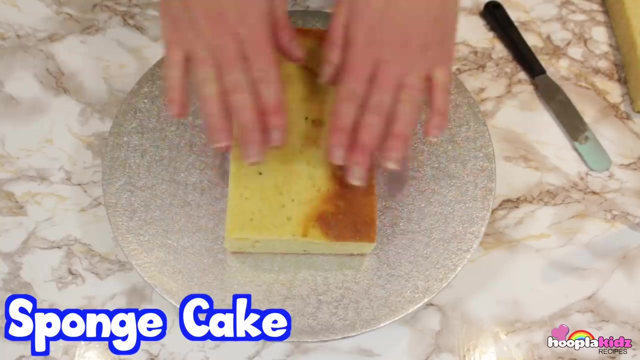 And what a great cake. It looks like there are little pigs in mud, Perfect. And there you have it. Don't they look fun? Elsa Shoecake, Doesn't this look cool? So let's start on that. To start off with our sponge cake, I'm using a bit of blue buttercream frosting to stick it onto a silver base. 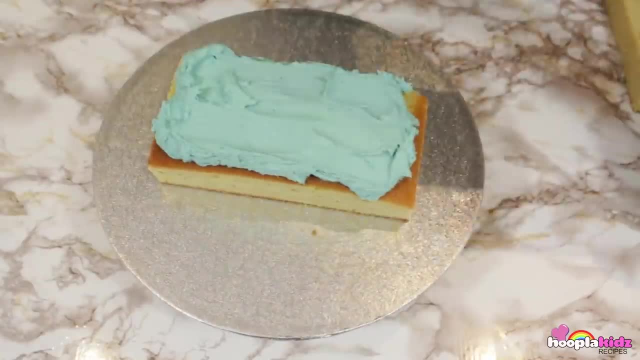 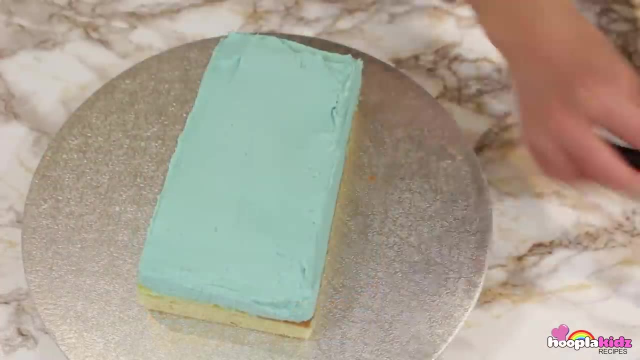 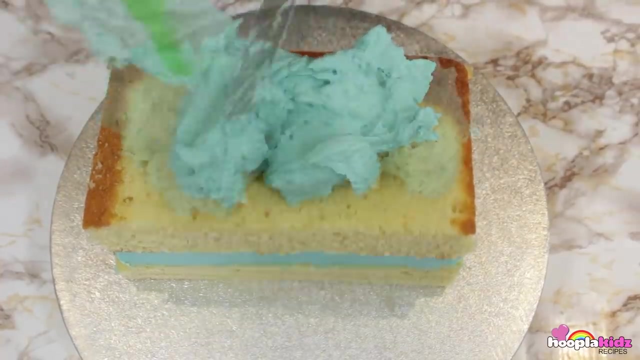 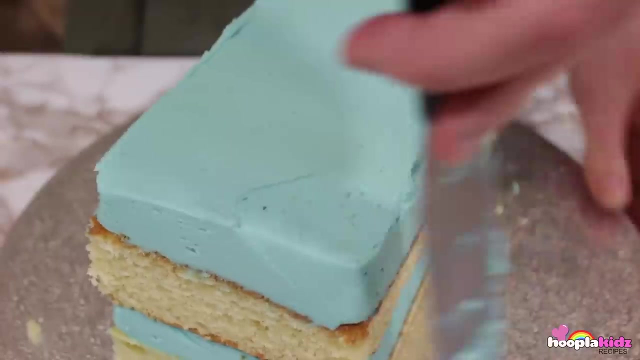 Once that's done, I'm going to add some more buttercream frosting on top. This is going to create the layer of the shoe. I'm now adding another bit of sponge on top of that and some more blue buttercream frosting Spread it out. We want to square it off and I'm using a palette knife to do this. 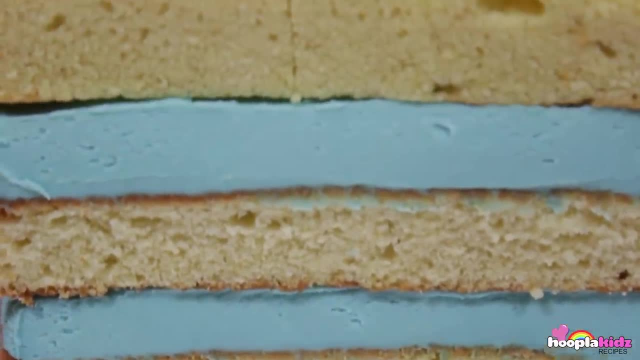 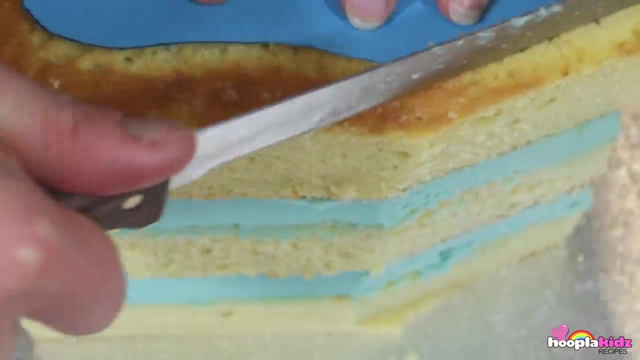 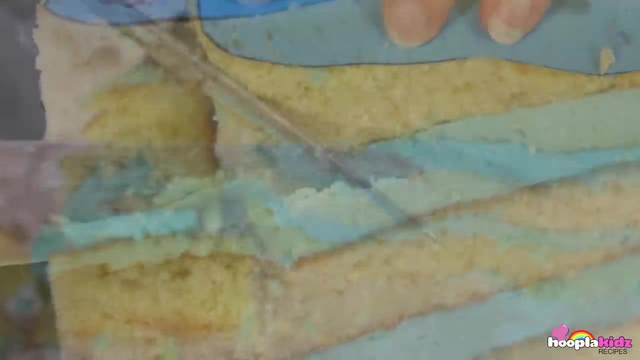 I'm going to add another layer on top of this. And doesn't that look awesome already? Now I have a shoe template. I'm going to cut around the shoe to make a giant footprint shape. Use your knife to shape the curves. We want to make sure that it's nice and smooth, Just like this. 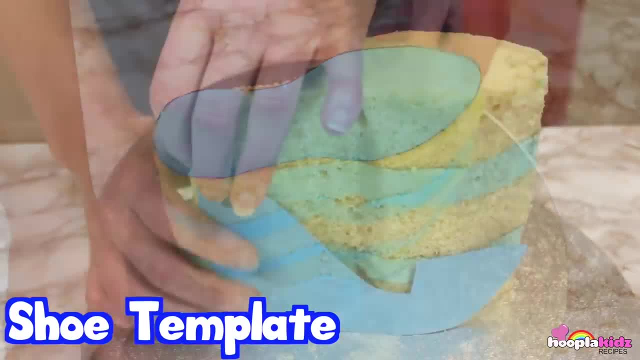 I'm going to cut around the shoe to make a giant footprint shape. We want to make sure that it's nice and smooth, Just like this, Perfect. I now have another shoe template which I'm sticking to the side of the cake. 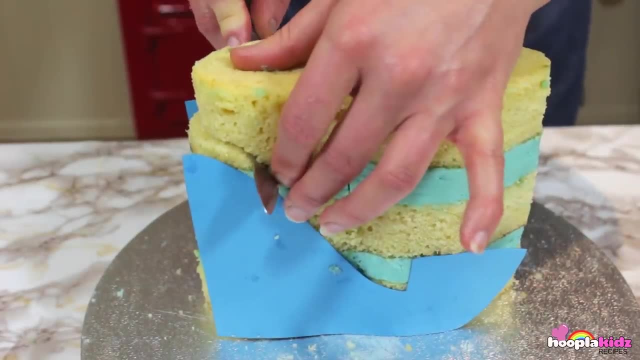 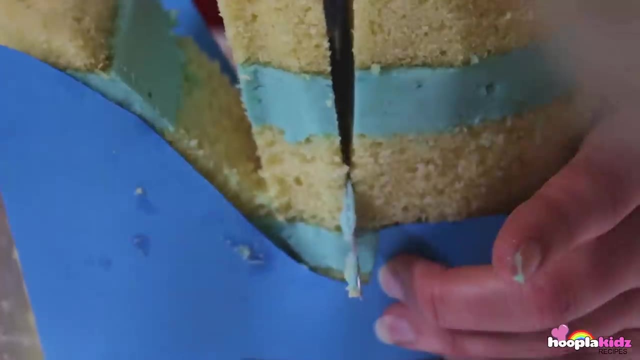 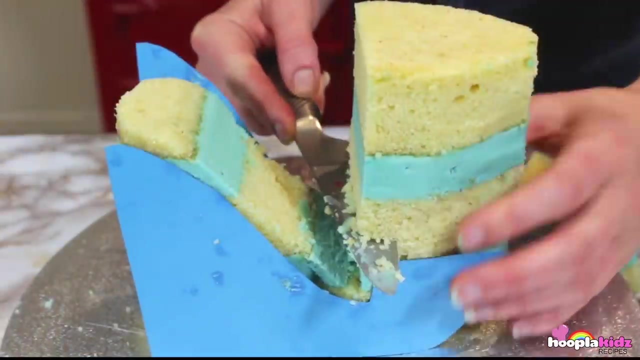 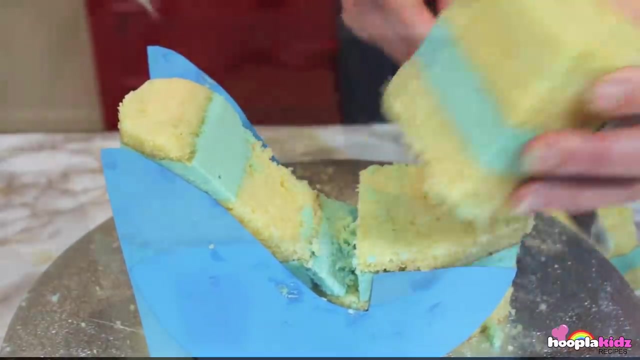 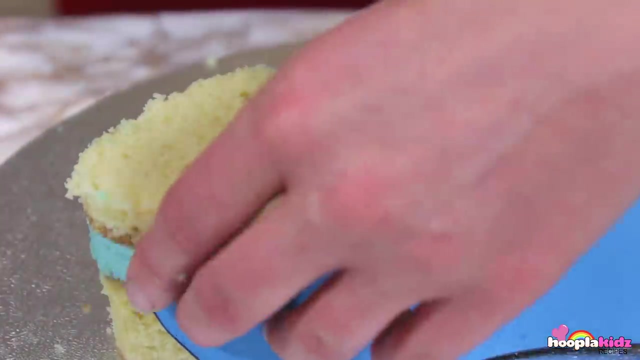 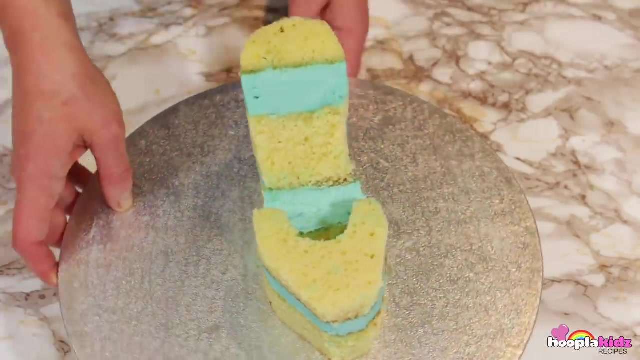 And I'm going to use this one to shape the top of the shoe. Looking good, I'm cutting out a semi-circle to make it look like a proper high-heel. great, this is already starting to take shape. I'm now going to do a bit more shaping at. 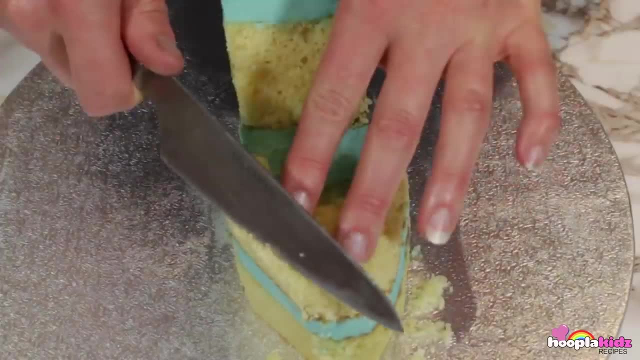 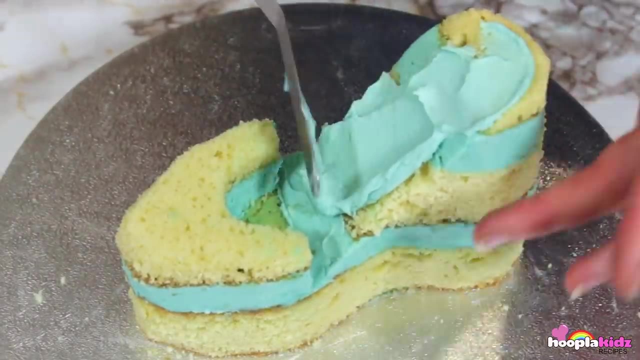 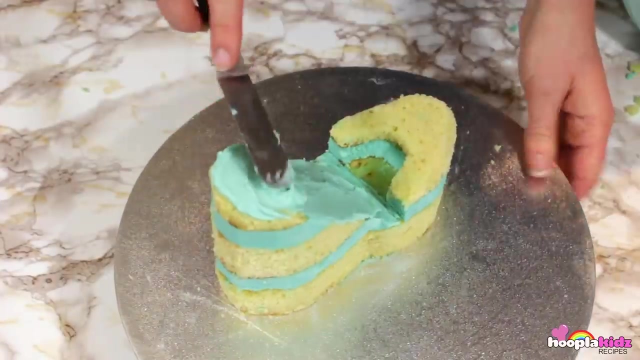 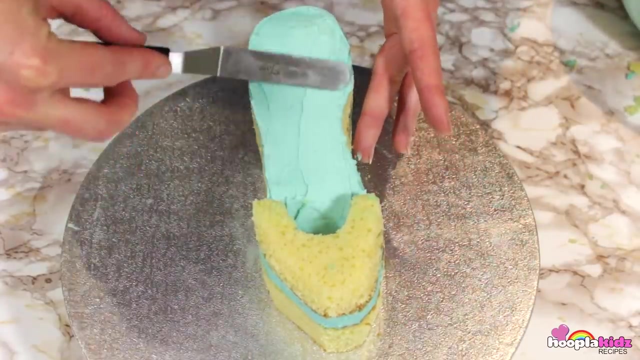 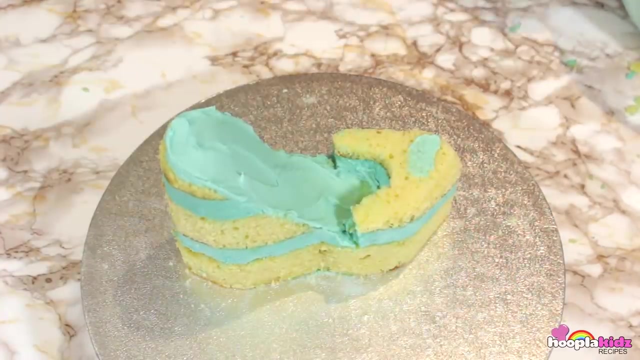 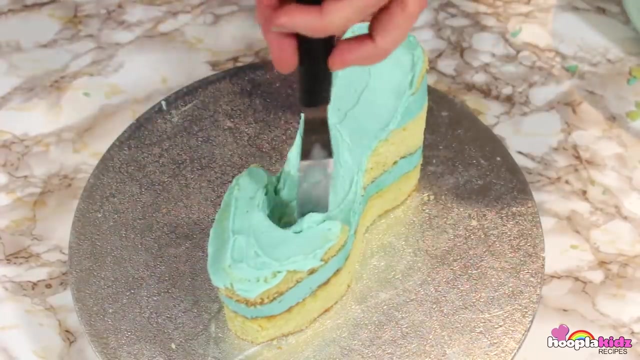 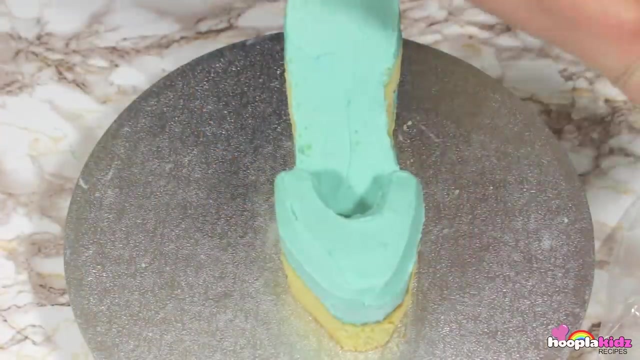 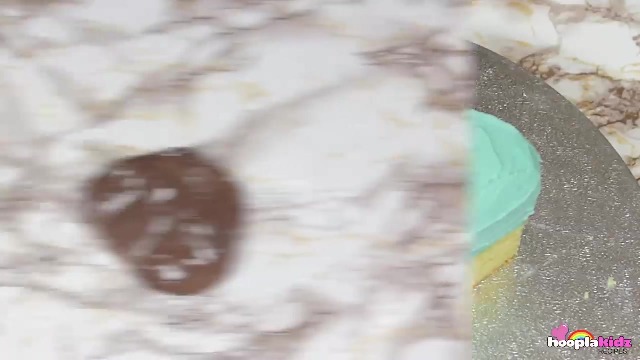 the toe, just to give it a bit of a curved effect. now I'm taking some blue buttercream frosting and I'm adding it to the inside of the shoe. I'm also going to cover the top of the shoe. use your knife to smooth down the icing to get a really smooth finish. dip your knife in some hot water. now I'm 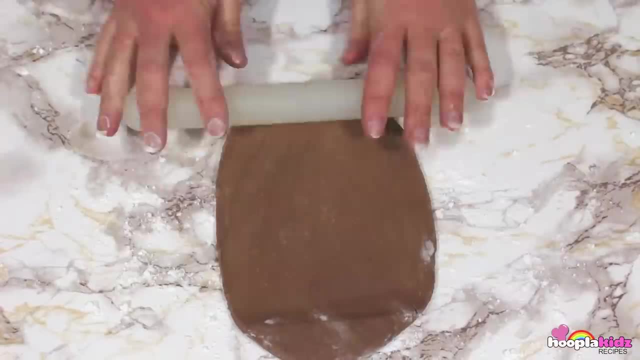 going to take some molding chocolate. I've lightly dusted my worktop and I'm rolling it out flat. I'm taking some chocolate and I'm going to take some chocolate and I'm going to take some chocolate and I'm going to take some chocolate and I'm going to 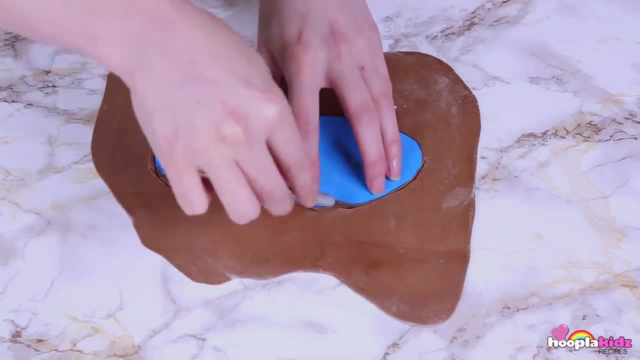 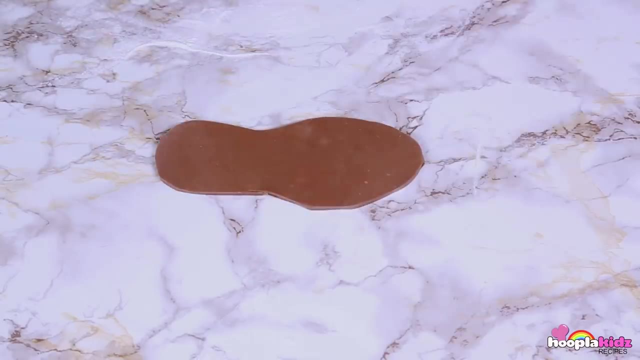 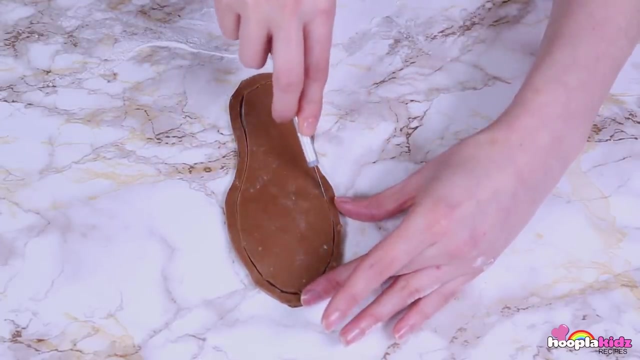 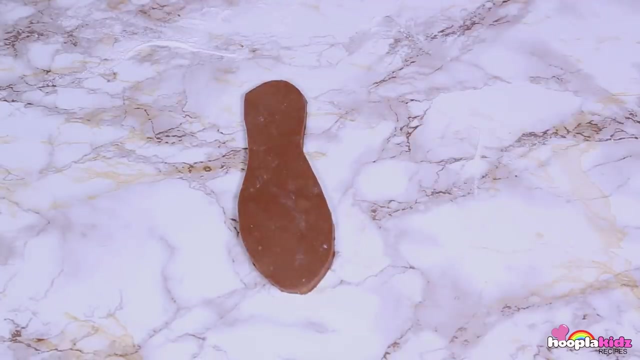 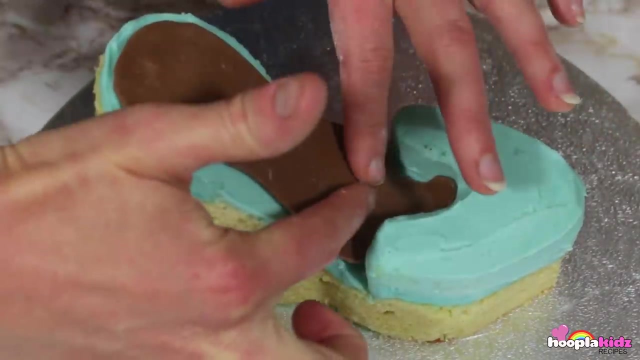 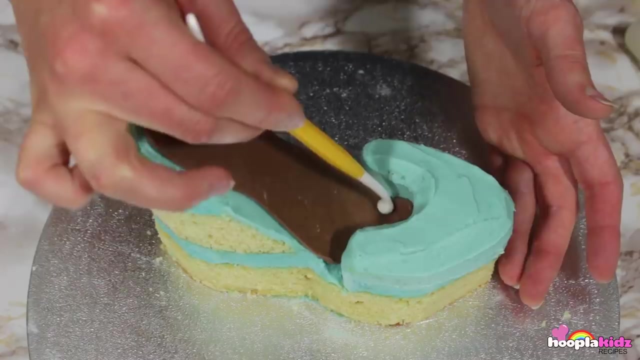 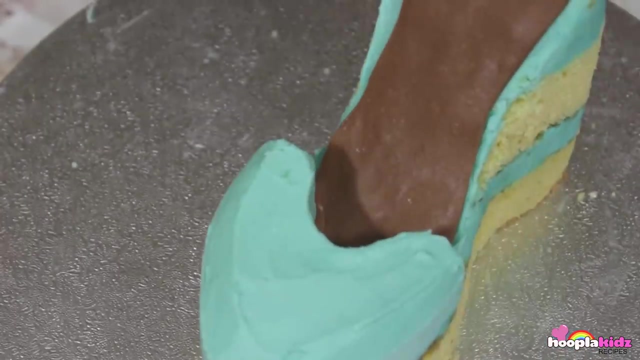 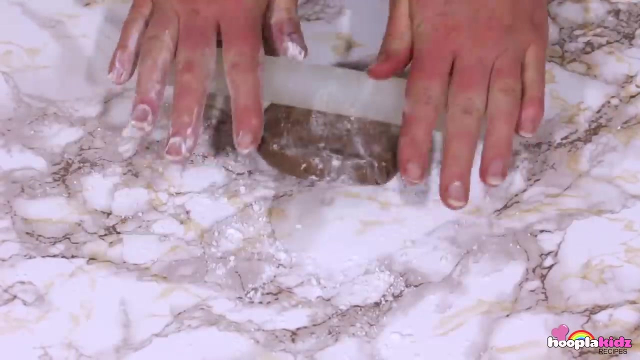 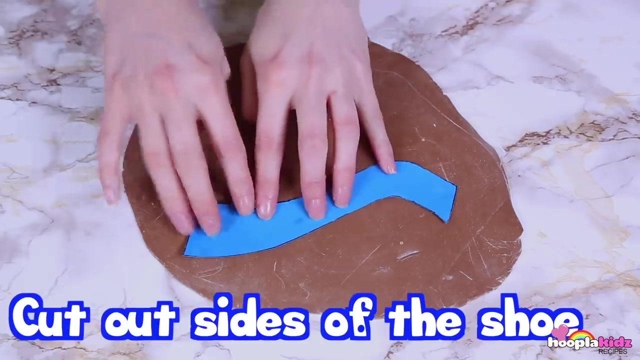 taking the inner sole template and cutting around it. perfect, I need this to fit inside the shoe, so I'm making it slightly smaller. looking good, press it into shape. Wow, it already looks amazing. now I'm taking some more molding chocolate, roll it flat again, and now I'm cutting out the side of the shoe. 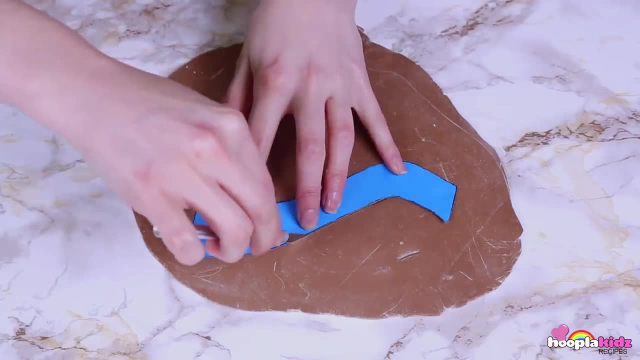 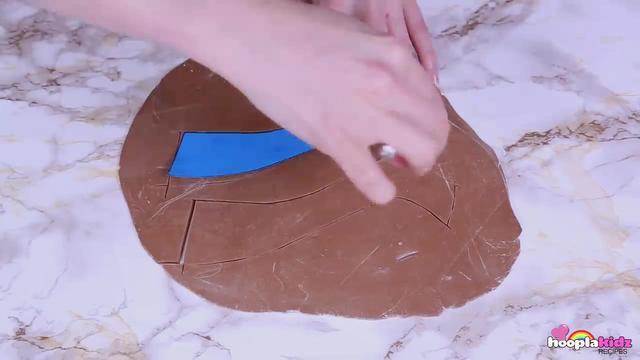 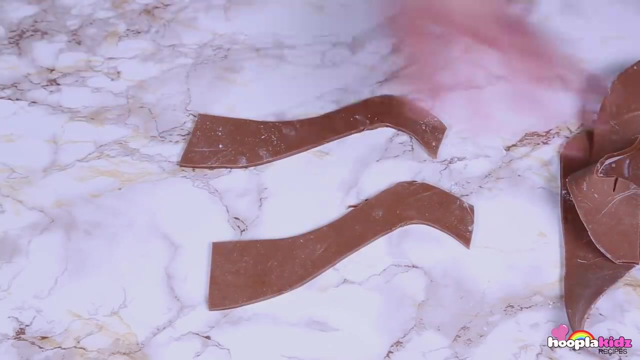 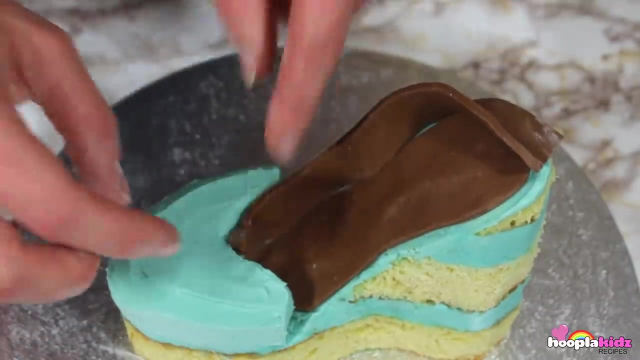 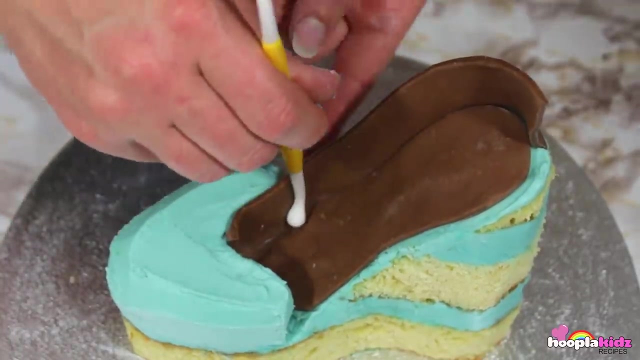 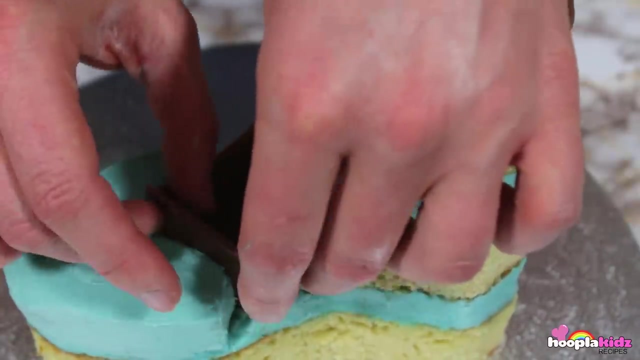 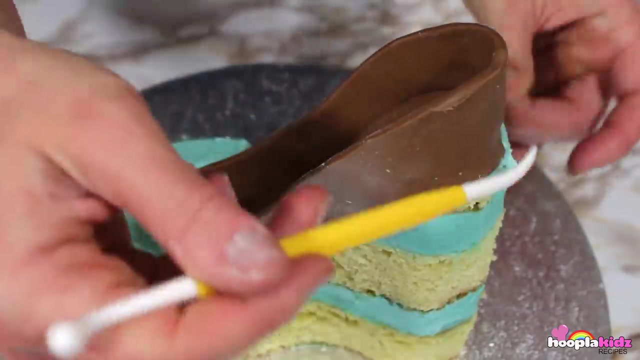 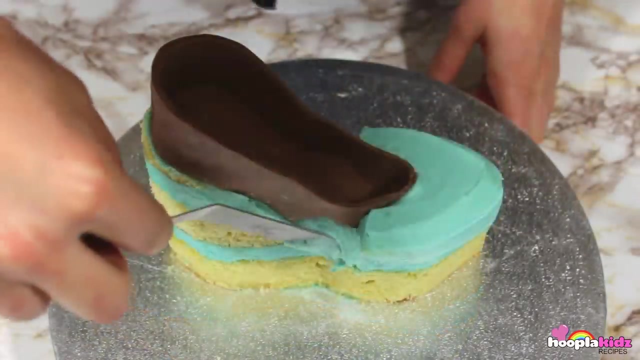 using the template. perfect, This is going to wrap around the shoe, just like so. This is why it's important to use the molding chocolate, because you can bend it to shape. we're repeating that process on the other side of the shoe. I'm now covering the chocolate in the molding chocolate. 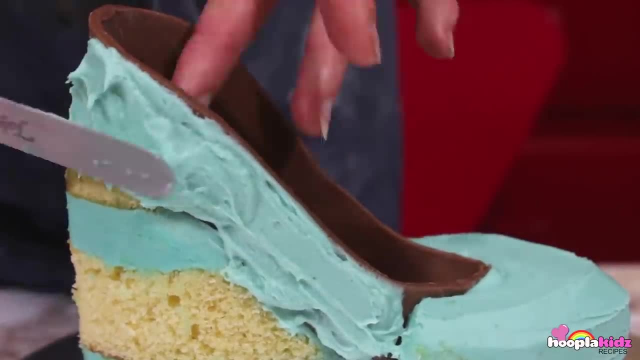 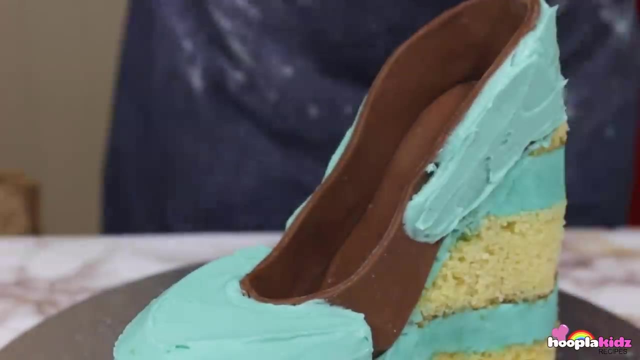 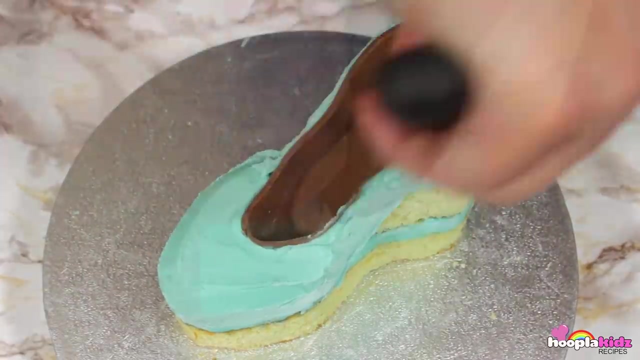 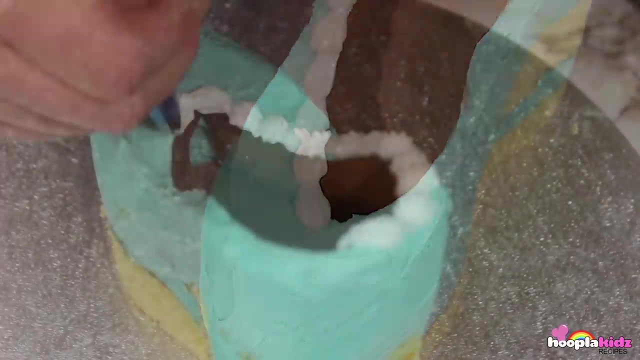 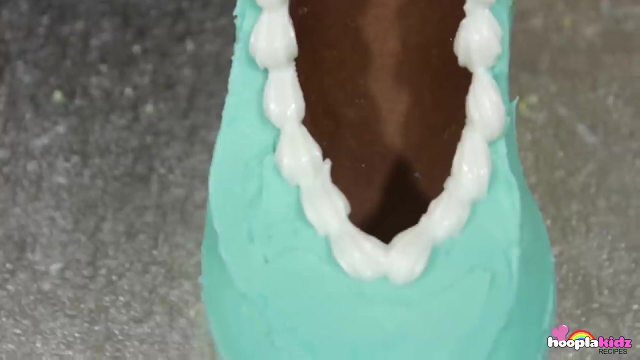 in some more blue buttercream frosting- looking good. smooth it down and now take some white icing in a piping bag with a special nozzle to do some trim. we're going to do this all around the rim of the shoe, just like, so I'm going to add one giant dot at the bottom and put on a snowflake piece of candy. 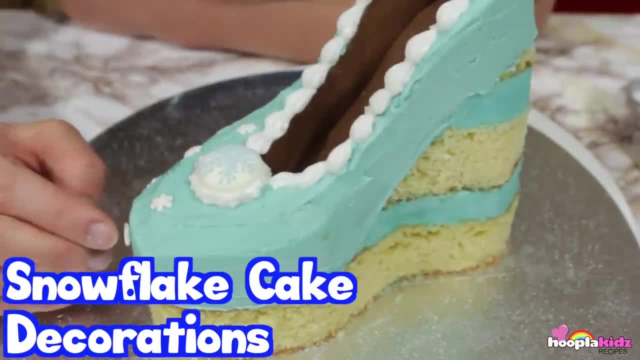 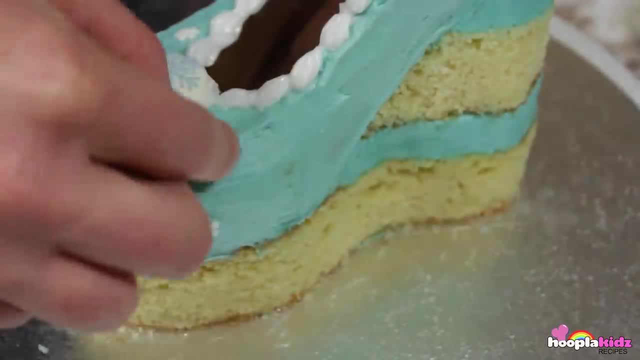 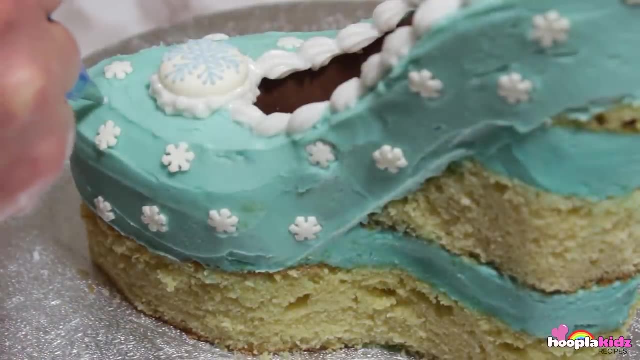 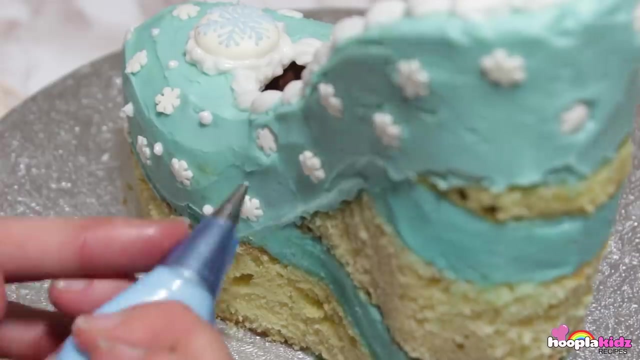 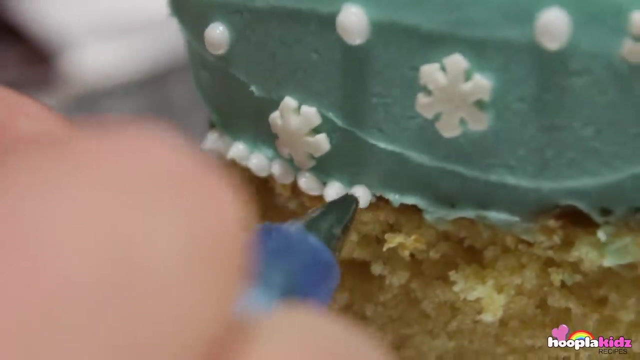 I'm now decorating the rest of the shoe with some tiny snowflakes. These look super cute. once you finish doing that, add some white dots to add a bit more decoration and texture to the shoe. I'm using some plain white icing to do this. finally, I'm adding white dots in between the sponge and the blue icing. 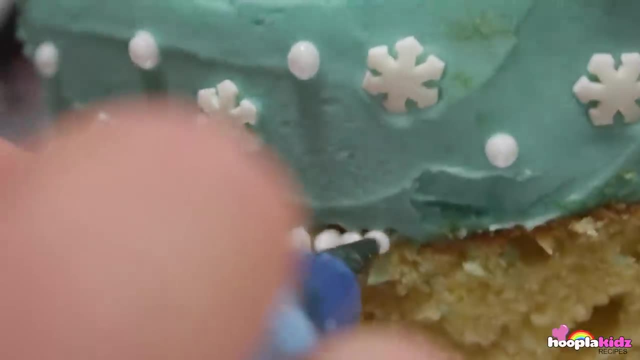 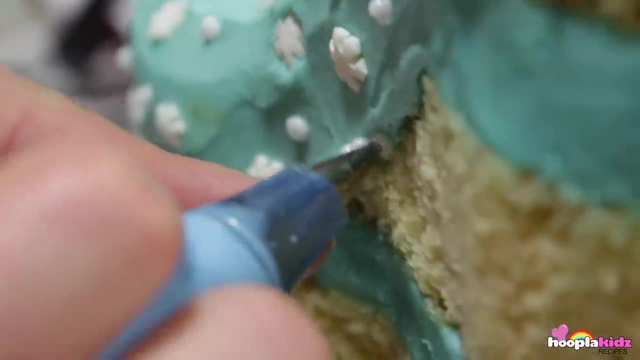 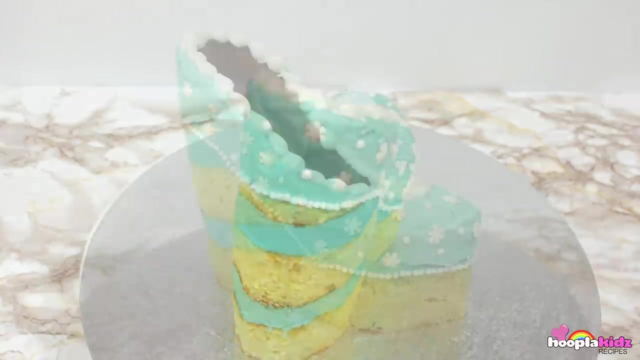 this is really intricate work, so you'll need to be patient. this is going to go all the way around the shoe, and there you have it. doesn't that look super cool? Not only does it look amazing, but it's also going to look really cool. 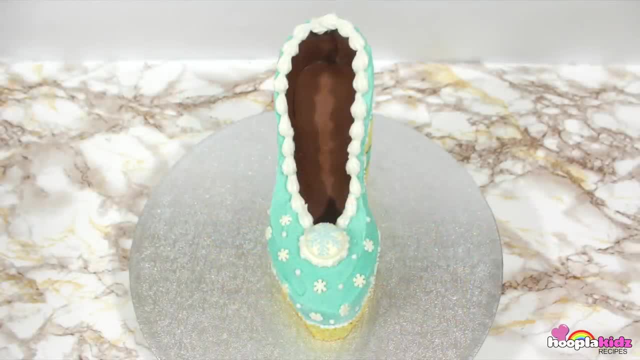 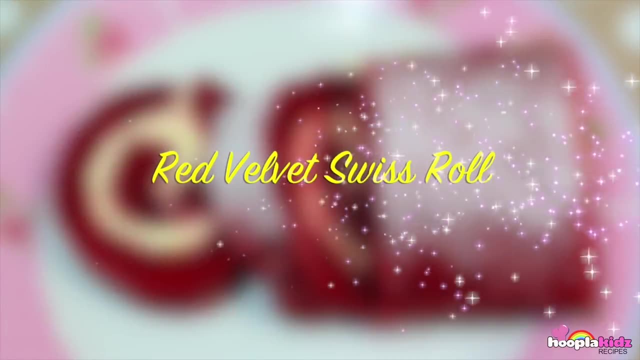 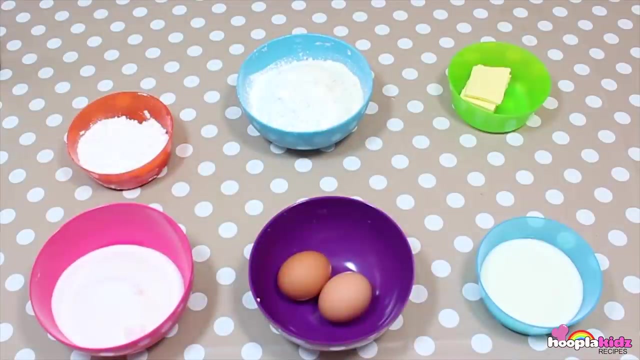 There you have it: an Elsa shoe cake, A red velvet Swiss roll- Delicious. For this you're going to need icing sugar for dusting. 200 grams of sugar, 190 grams of flour, 2 eggs, 60 grams of unsalted butter, 120 mils of buttermilk. 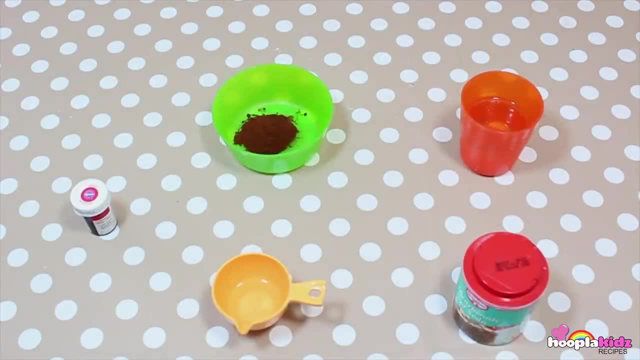 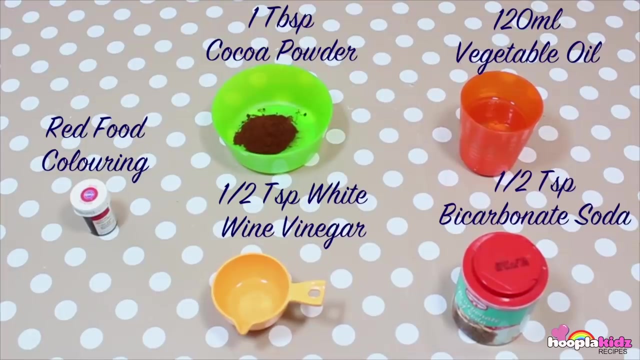 You're also going to need some red food colouring: 1 teaspoon of cocoa powder, half a teaspoon of white wine vinegar, 120 mils of vegetable oil and half a teaspoon of bicarbonate of soda. and for the cream cheese filling you are going to need: 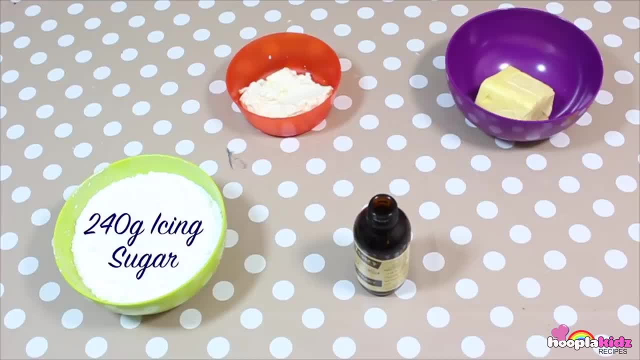 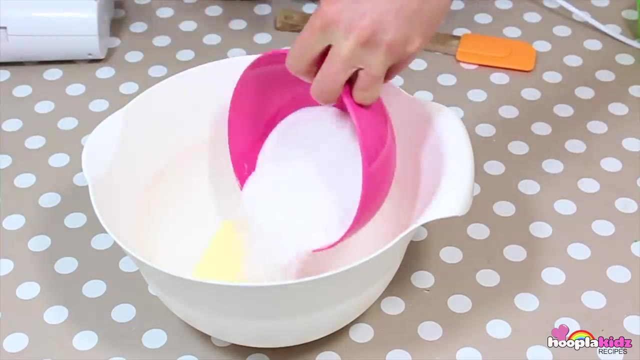 240 grams of icing sugar, 150 grams of cream cheese and a little bit of sugar, 1 teaspoon of vanilla extract and 100 grams of unsalted butter. so let's get started. we're going to add the butter, then the sugar to a bowl and, using an electronic, we're going to whisk it. 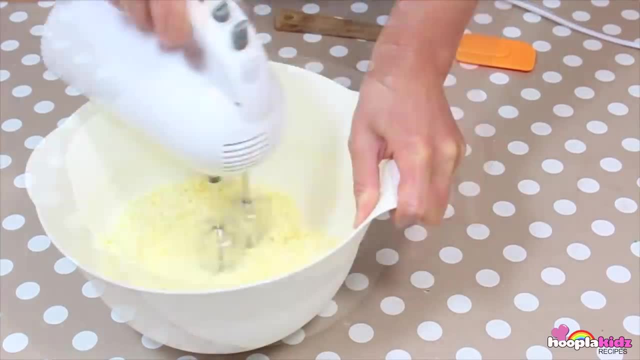 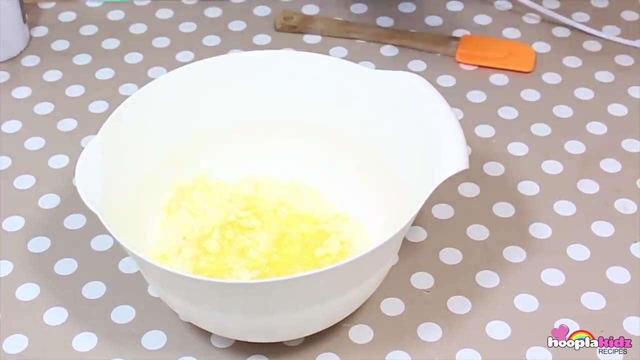 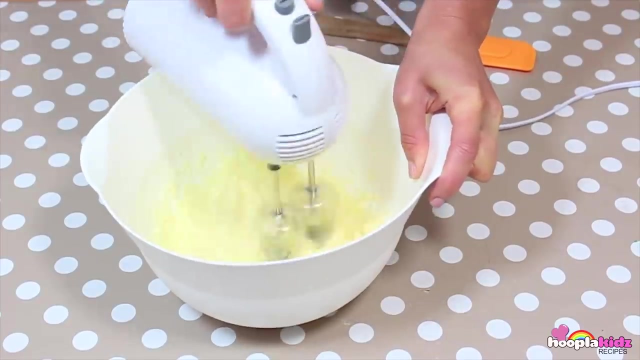 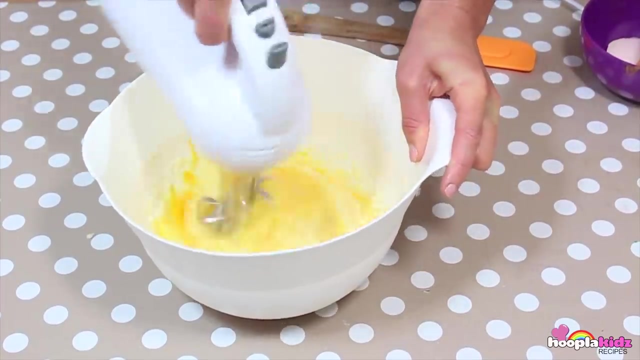 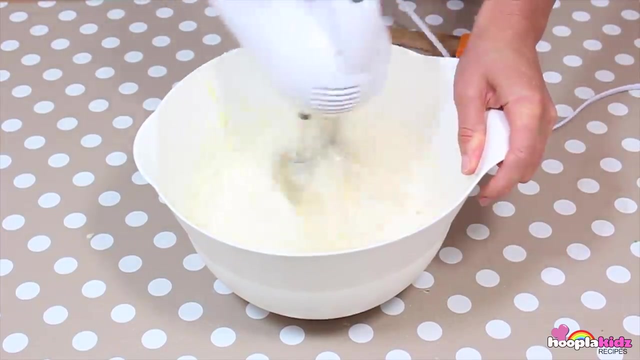 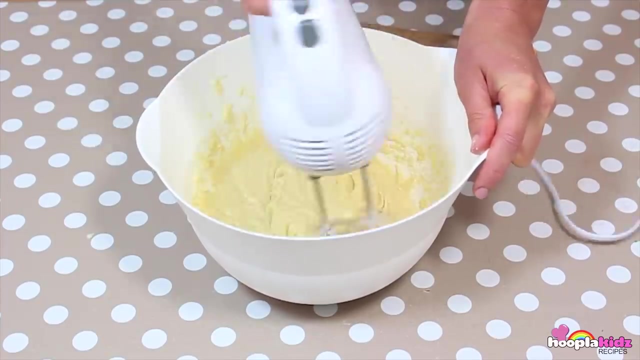 we don't want any lumps. now we're going to add the vegetable oil, give it a good stir, and then we're going to add the eggs. next we're adding both of our eggs, then add flour, keep stirring. now we're adding our cocoa powder. I can't wait to take a bite. 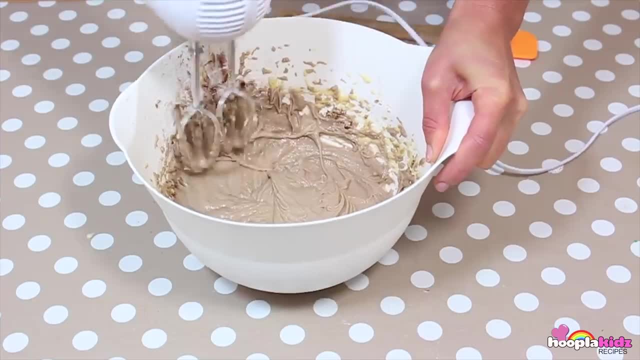 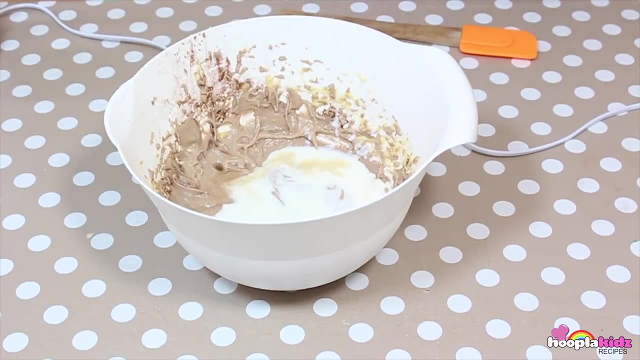 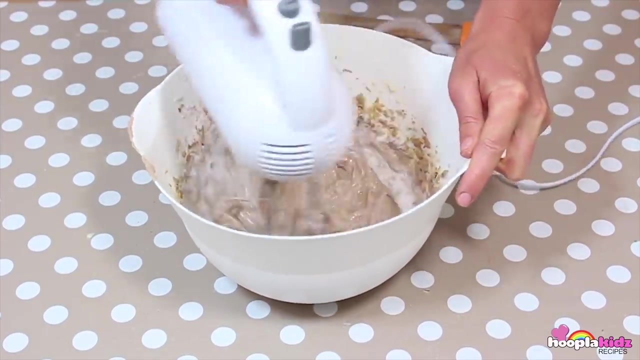 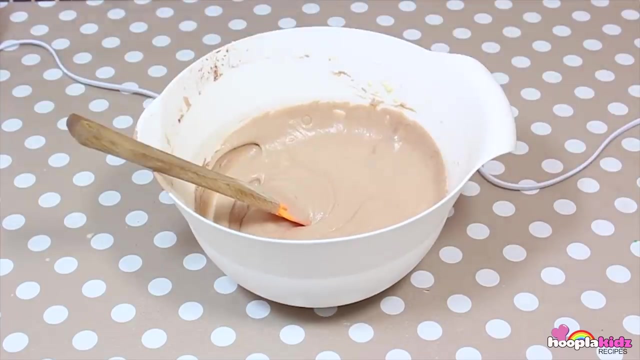 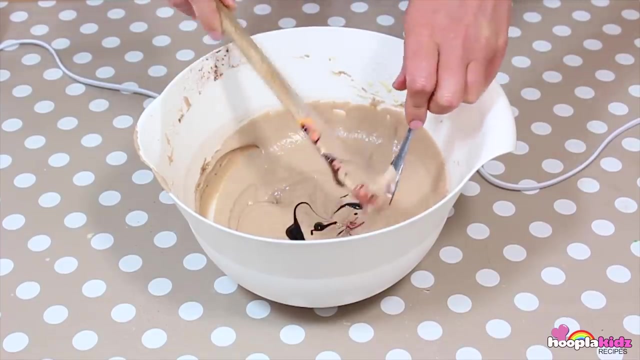 I can't wait to taste this. we're also going to add our buttermilk and our white wine vinegar, add the bicarbonate of soda and give it a good mix. now we need to colour it, because we all know that red velvet is red, so add the food colouring. 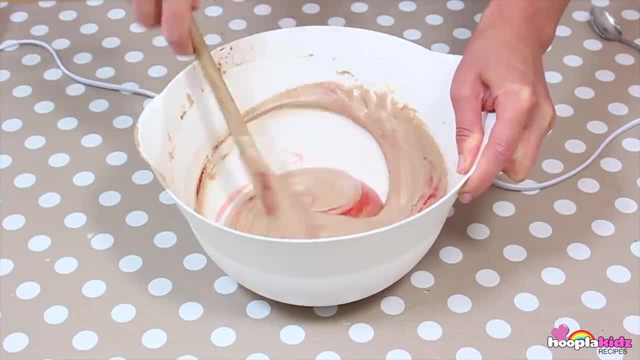 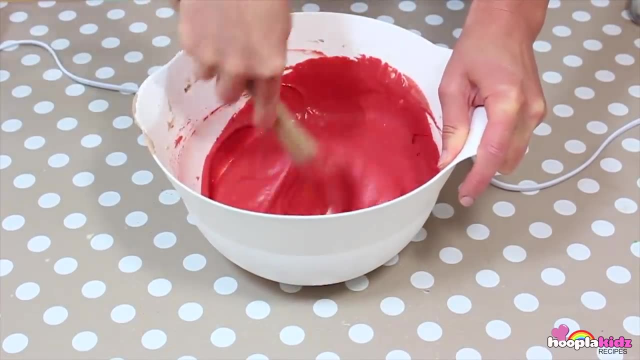 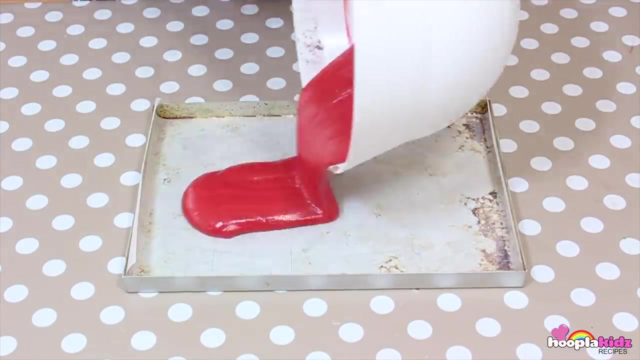 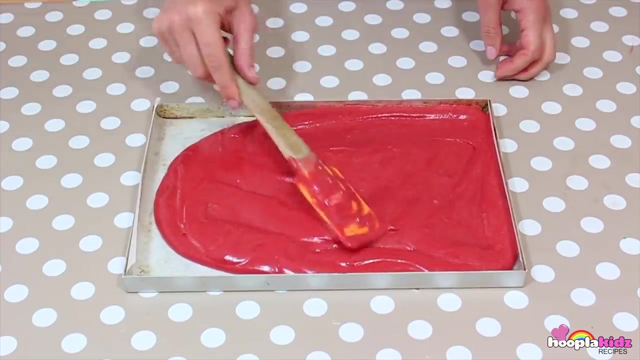 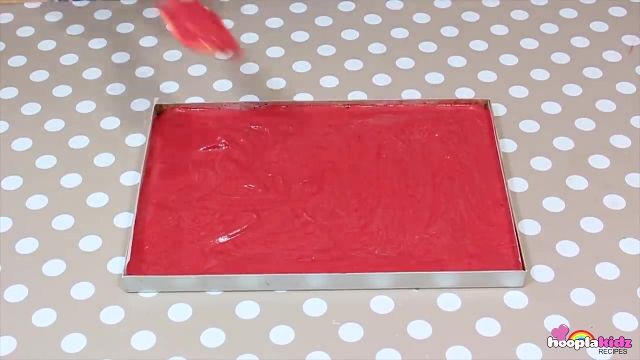 and stir. you want it to be a dark, deep red, just like this. now we want to take that and fill a lined baking tray. smooth it down so it goes all the way to the edges and the top is smooth. put it in the oven for 15 to 20 minutes. 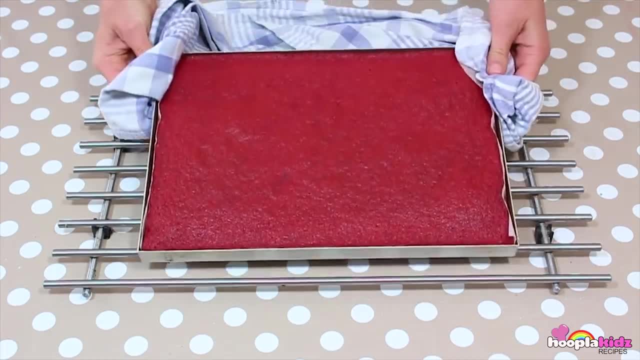 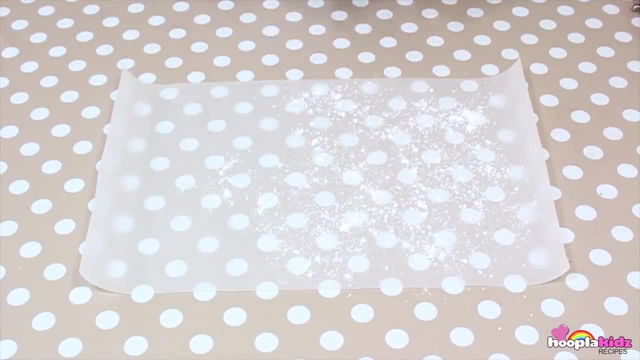 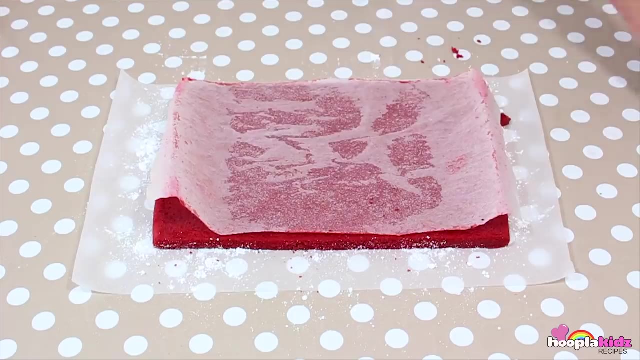 at 180 degrees celsius, and this is what it will look like: delicious. we now need to roll it before it cools so that it keeps its shape. lightly dust some baking paper and then add your red velvet cake on top. but be careful, it is still hot. 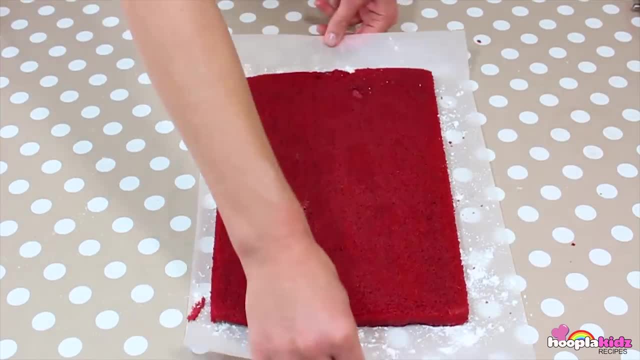 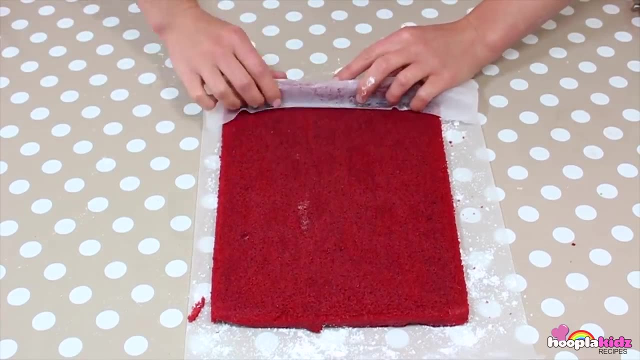 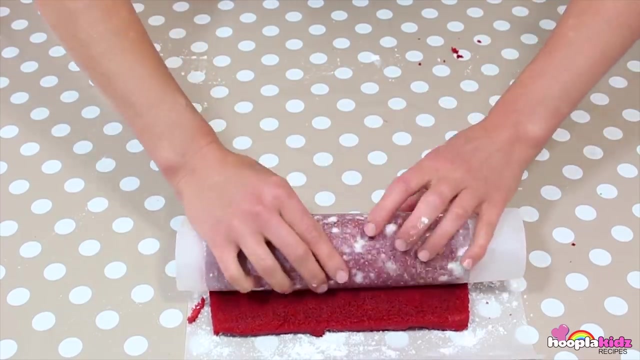 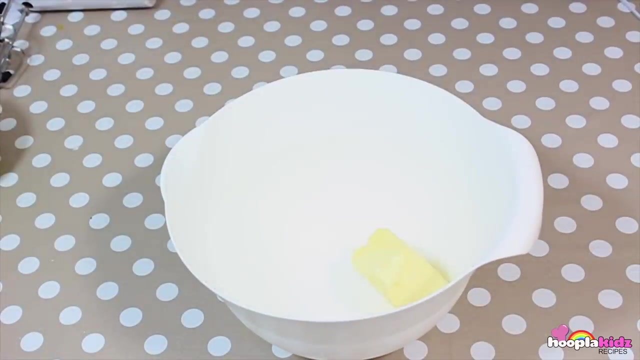 so don't worry, if you don't have a baking paper, you can use a kitchen towel. now it's time to roll. keep rolling. we're going to roll it with the baking paper in place and set it aside for it to cool. now we'll make the cream cheese filling. 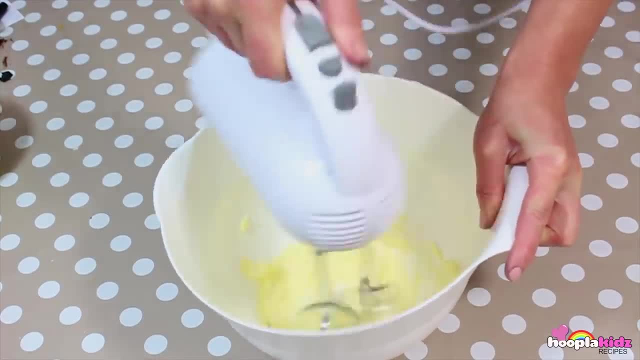 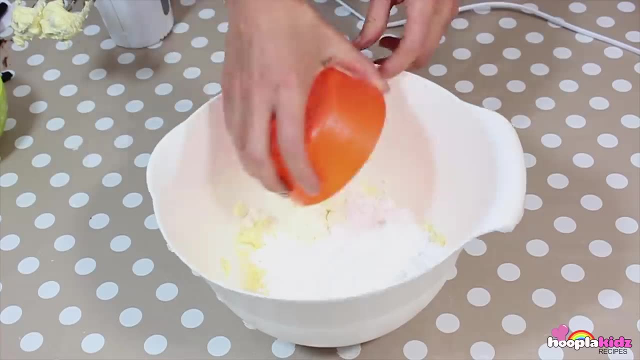 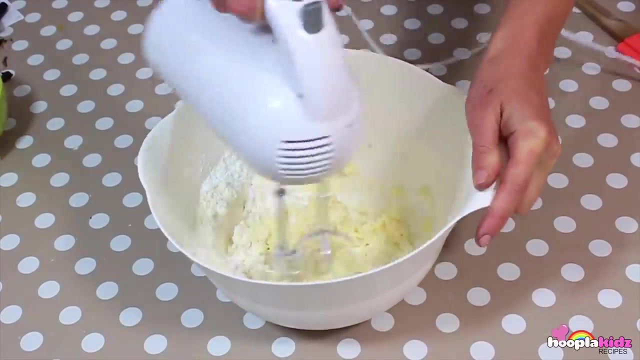 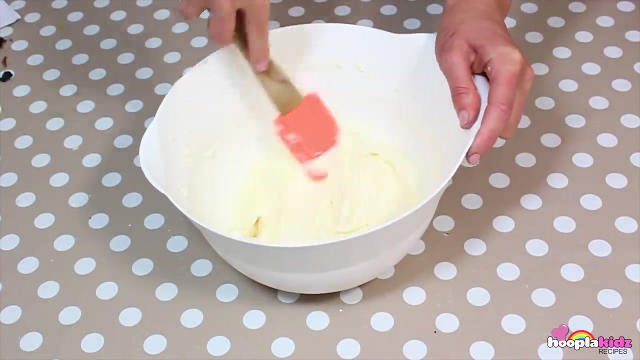 add your butter to a bowl, add a dash of vanilla extract and mix it all together. now add your icing sugar and your cream cheese, add a dash of vanilla extract and mix it all together. super yummy. now we're going to add our vanilla extract and mix it all together. 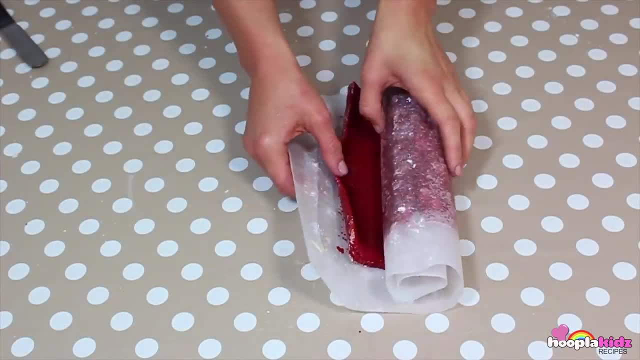 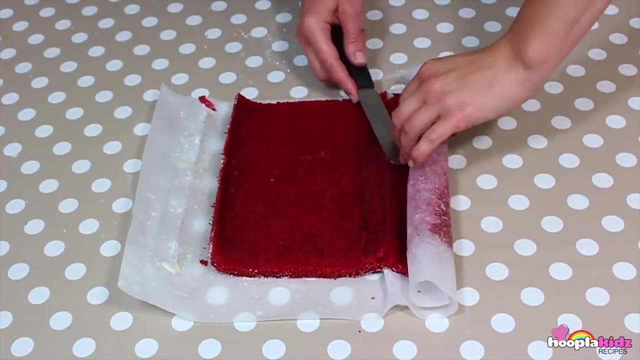 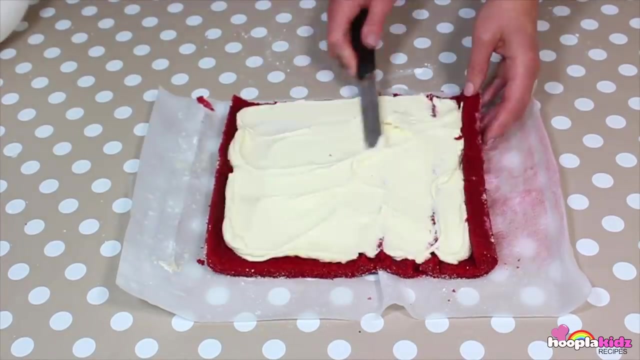 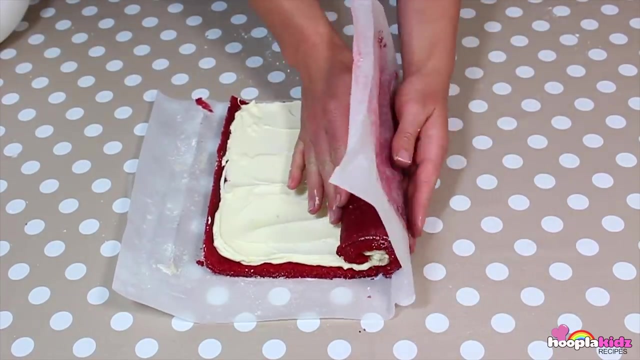 now we want to go back to our roll. now we want to go back to our roll. we're going to unroll it and add the cream filling. now it's time to re-roll it, without the baking paper in the middle. now it's time to re-roll it. 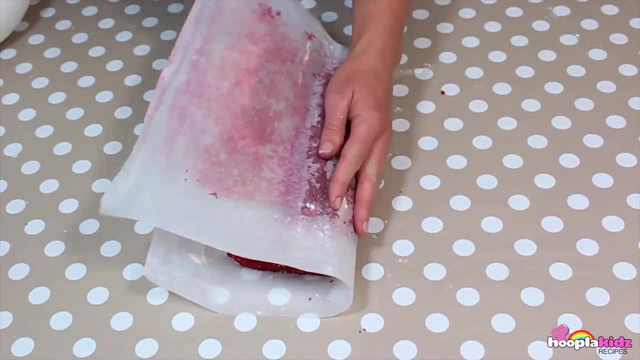 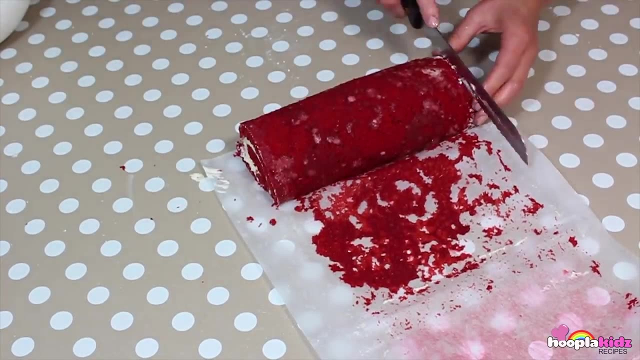 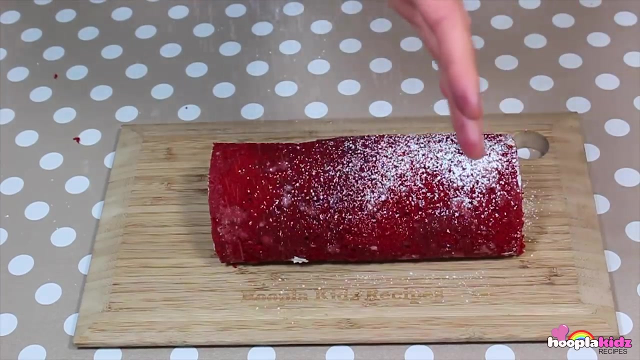 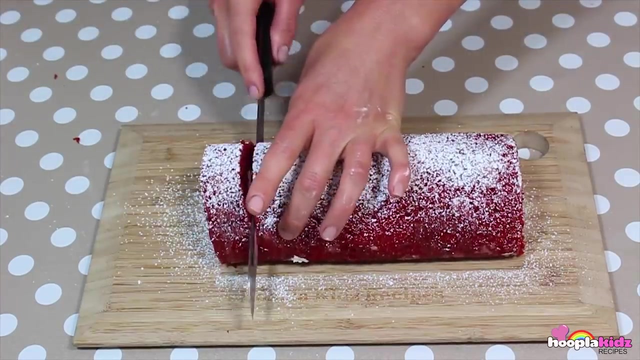 without the baking paper in the middle. now it's time to re-roll it without the baking paper in the middle- delicious. neaten up the ends using a knife, and then we're going to dust it with icing sugar. now, all you need to do now. all you need to do. 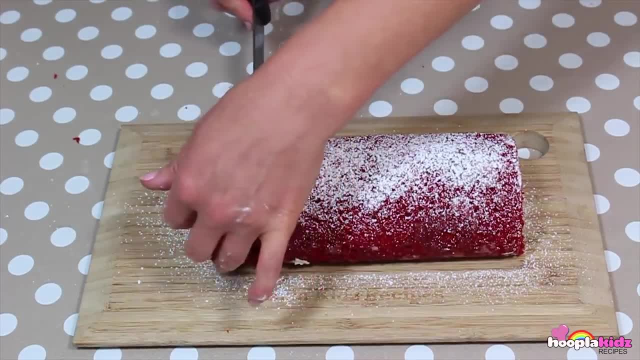 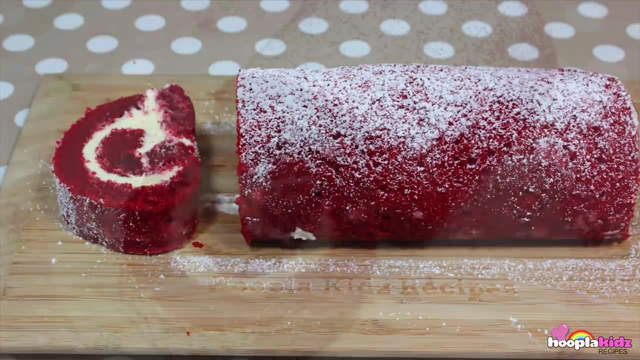 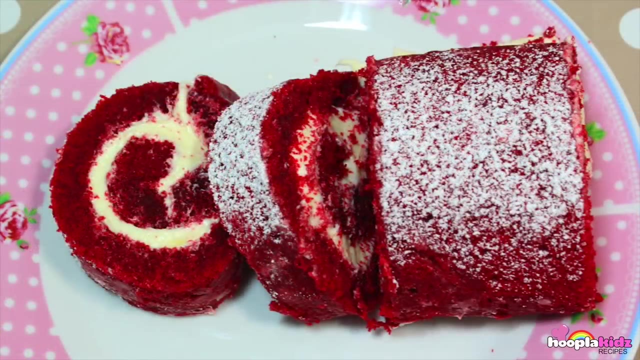 is to eat it. super delicious. yum. this looks amazing, doesn't it? this looks amazing, doesn't it? a red velvet swiss roll, a red velvet swiss roll, two of my favourite things. two of my favourite things. melting candle rainbow cake. melting candle rainbow cake. doesn't this look amazing? 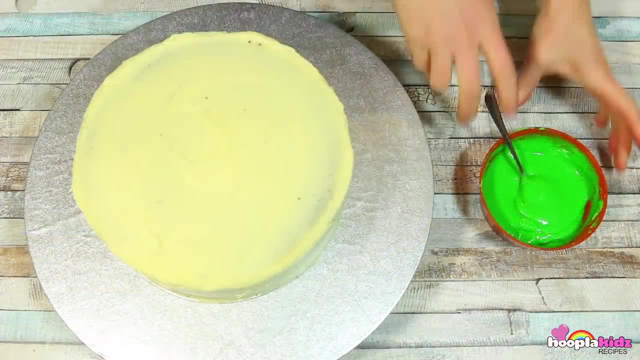 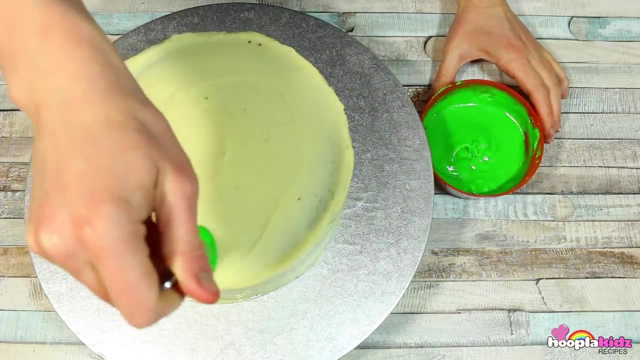 and it's so easy. let's start off with an iced cake. I've now got some buttercream icing that I've melted in the microwave. I'm drizzling it on top. it's going to look like melted wax and when it's not, it's completely edible. 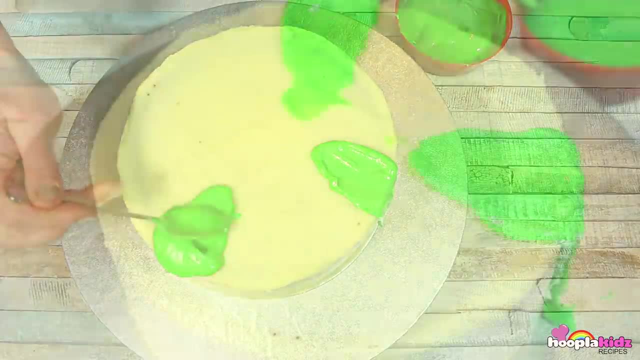 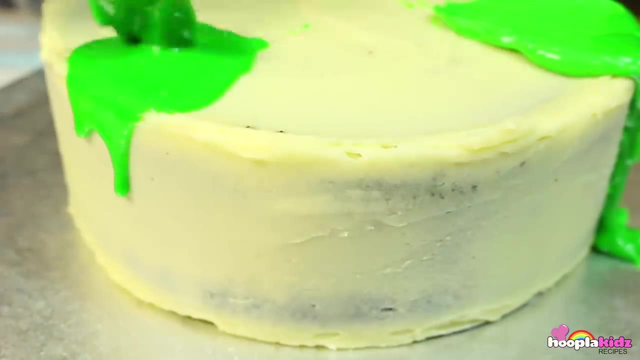 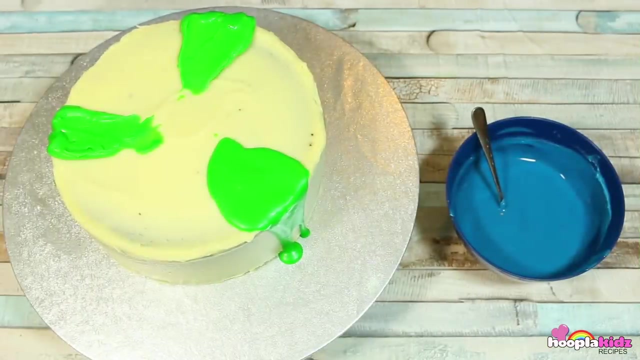 and super delicious. I don't want to cover the whole thing in one colour, so I'm only putting the green icing on a few sections. look at it. dribble down the side, doesn't it look great? it looks like melting wax. now I've done some green. 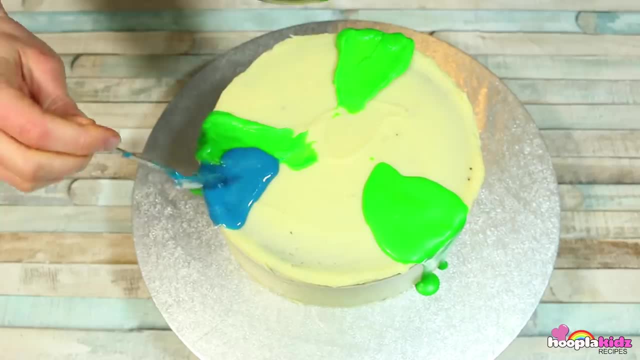 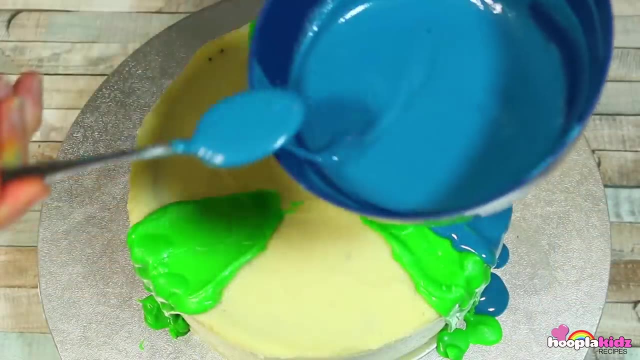 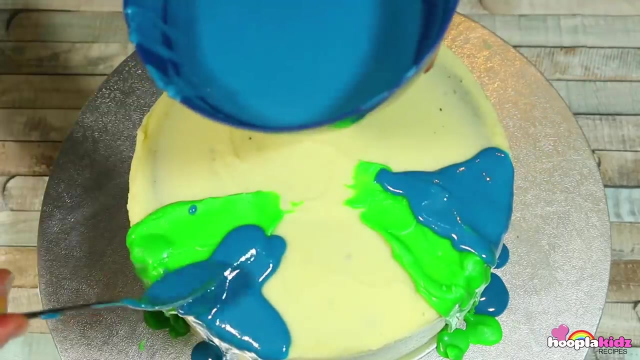 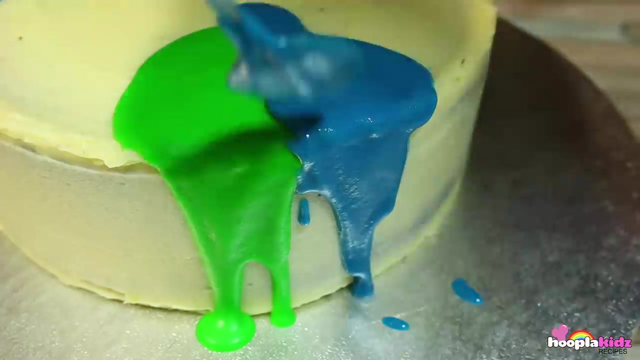 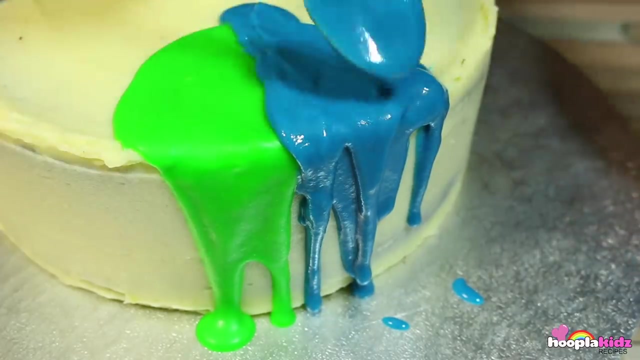 it's time to do some blue. I'm letting the blue dribble down over the green. it looks like a real candle would do. this is so much fun. look at it, go looking great. you can see it starting to harden. now let's do some yellow wax. 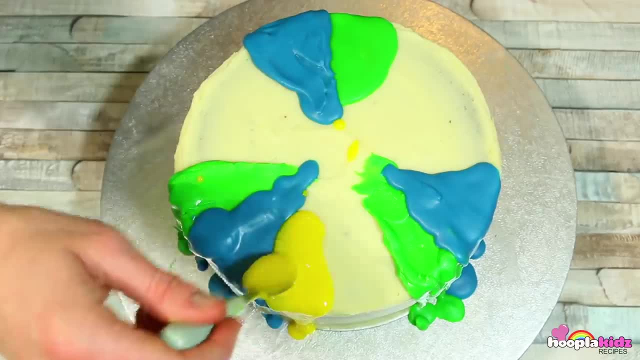 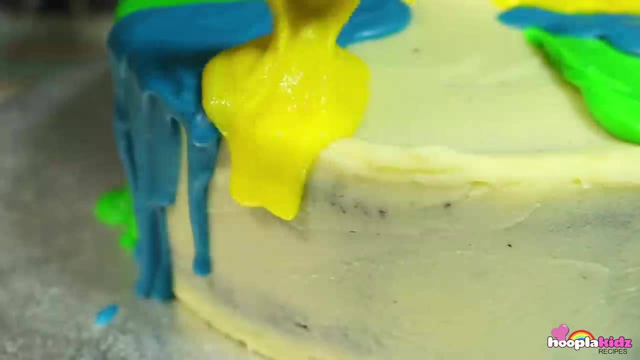 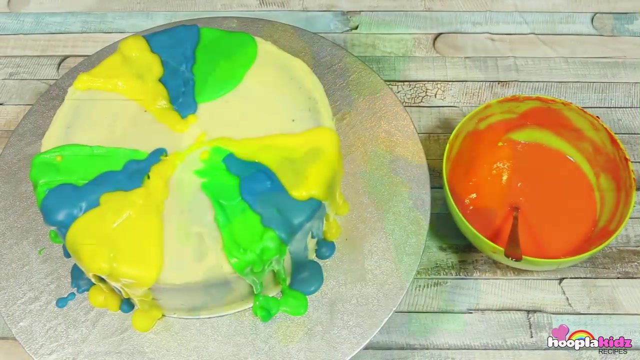 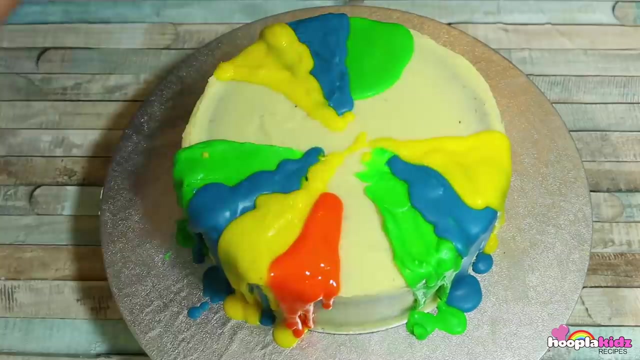 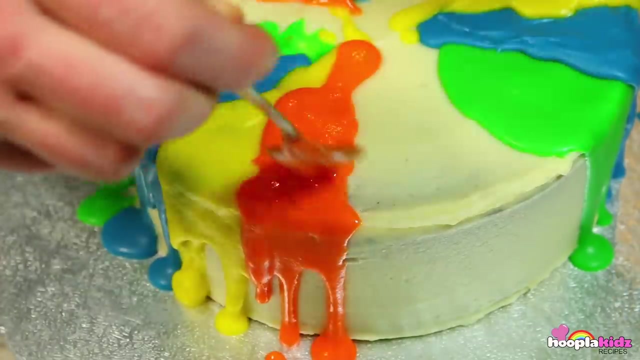 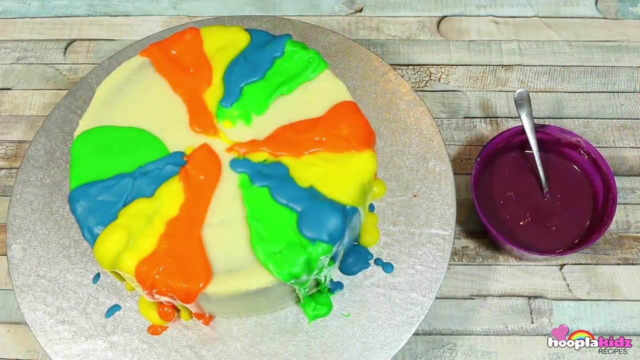 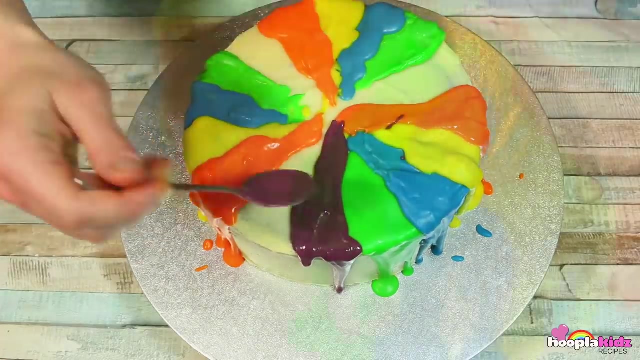 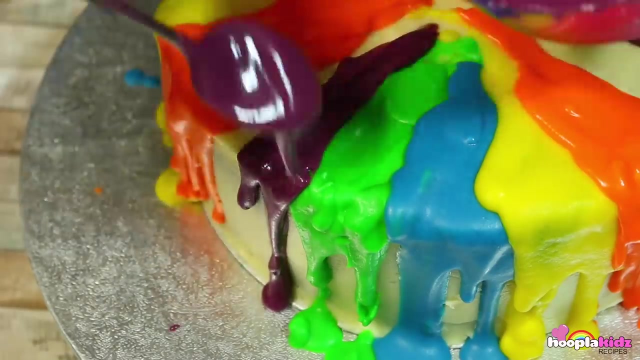 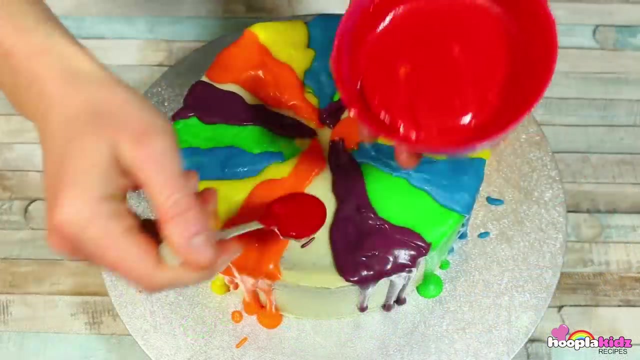 I mean icing. after yellow, I'm going to do orange. it's dribbling down and looks so cool already. it looks like candle wax right now. let's do some purple. finally, I'm doing red. finally I'm doing red. I've got all the colours of the rainbow. 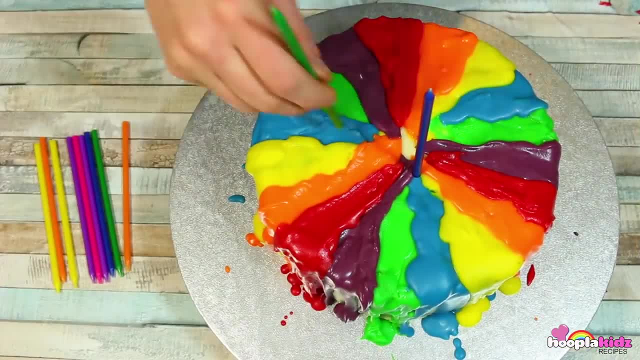 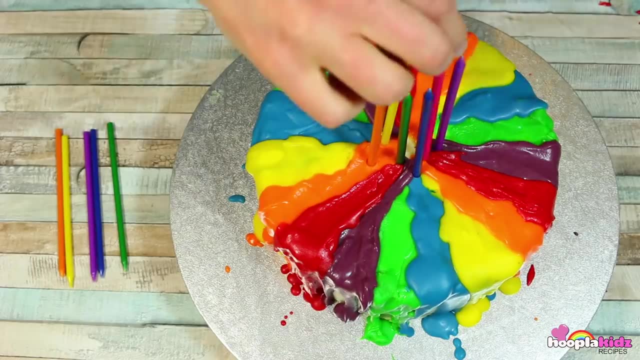 once that's done, we're going to put some different coloured and different sized candles in the middle of the cake. this will give the impression that these candles are what's melted, but of course you and I know it's completely edible and it's not the candles. 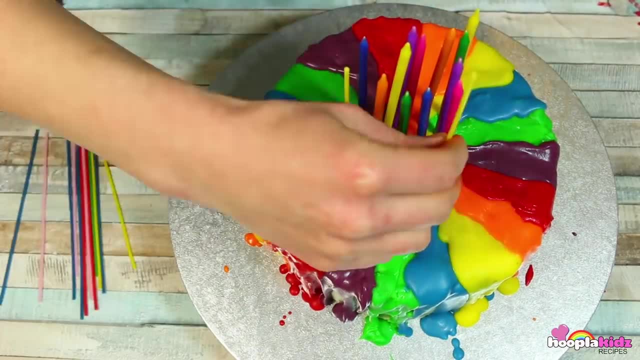 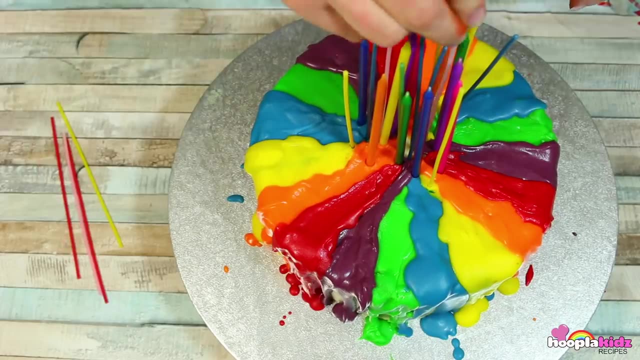 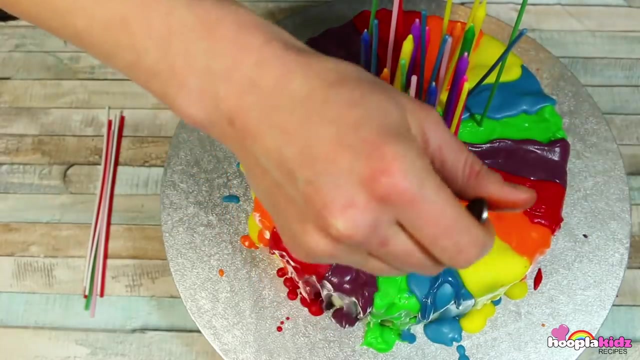 it's just icing looking good. I've got thin candles and thick candles. I've got thin candles and thick candles. once the candles are in place, we're going to start building up the buttercream icing. this will give more of an impression that the wax has melted. 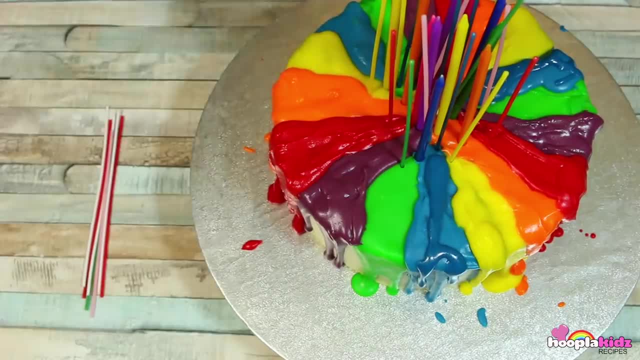 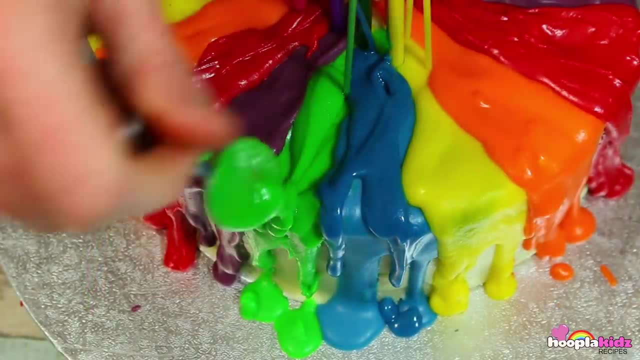 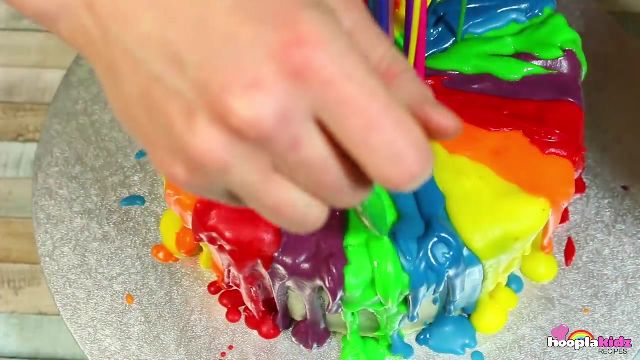 it will create a 3D effect on the top of the cake. on the top of the cake. on the top of the cake. you can only do this 3D effect once one layer has already dried and hardened. already dried and hardened. you want it to slightly overlap. 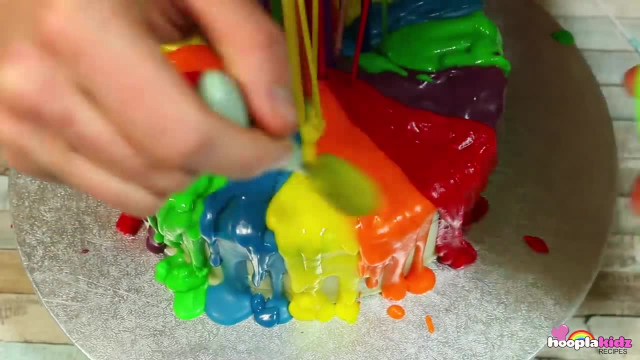 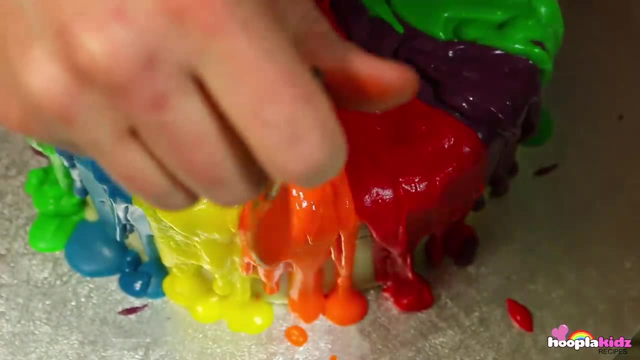 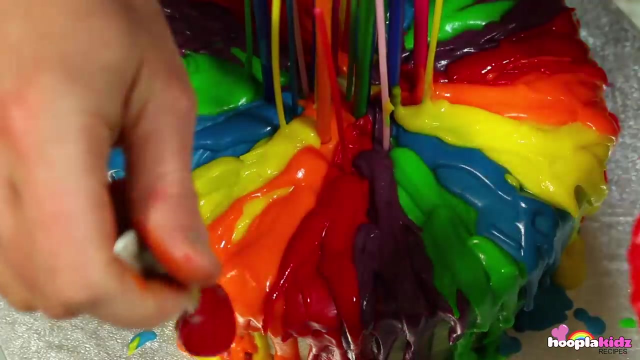 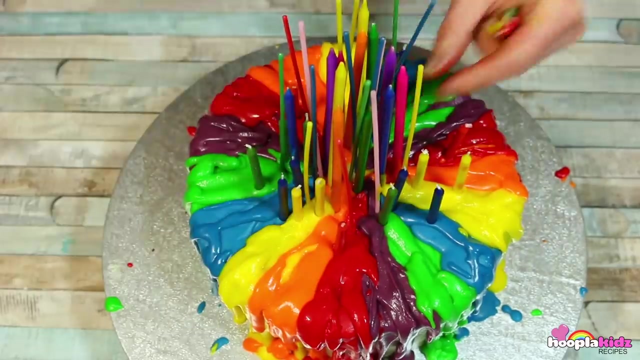 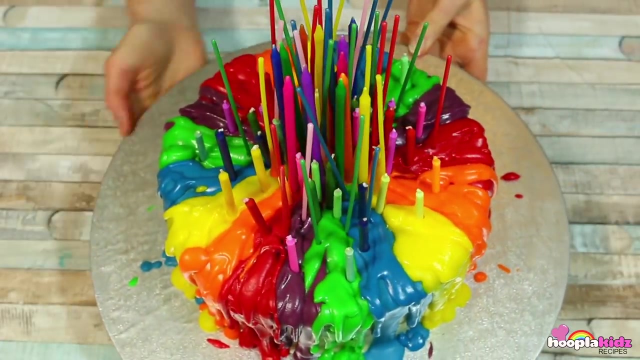 it makes it look even more realistic. it makes it look even more realistic, looking good Nearly there. wow, this looks amazing. Now I'm adding some more shorter candles and some more tall ones, And there you have it. Isn't it incredible? It looks like all the candles have melted and run off the plate, but it's not, it's. 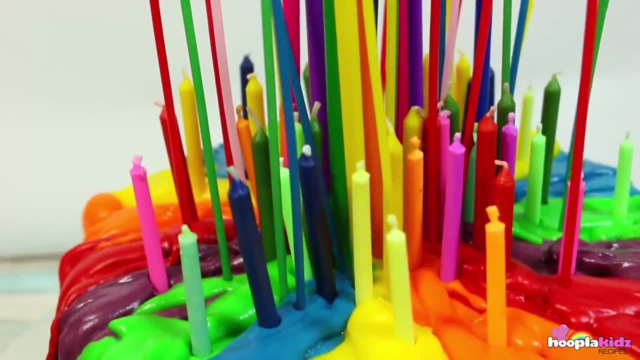 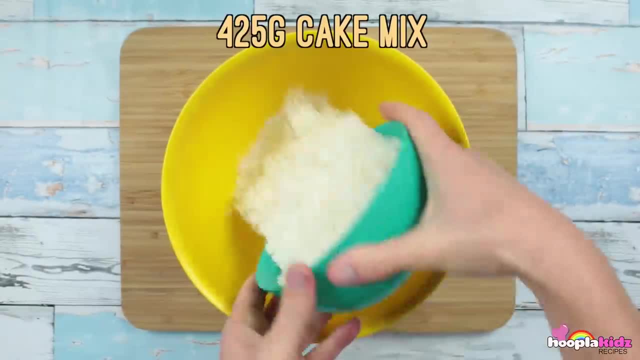 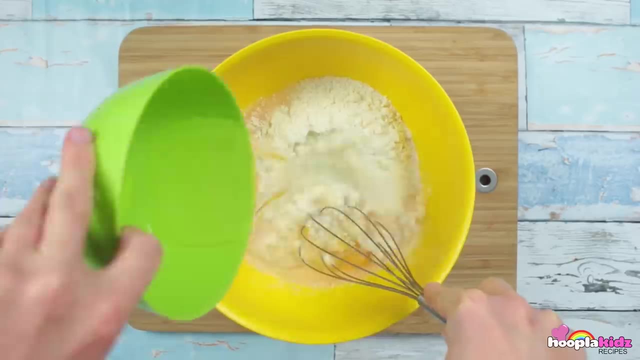 super edible and super delicious Pumpkin Pound Cake. Doesn't this look fantastic? So let's start with 425 grams of cake mix. I'm adding 2 eggs and 1 cup of water, and then I'm mixing it all together. 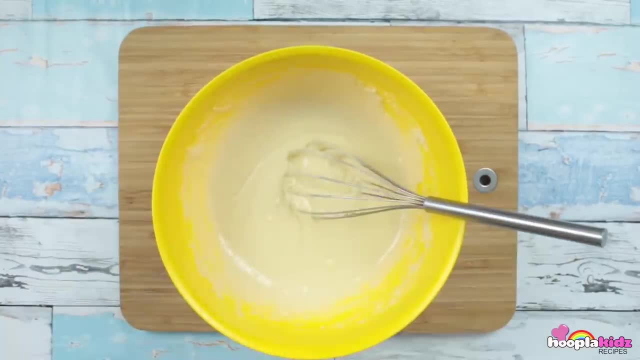 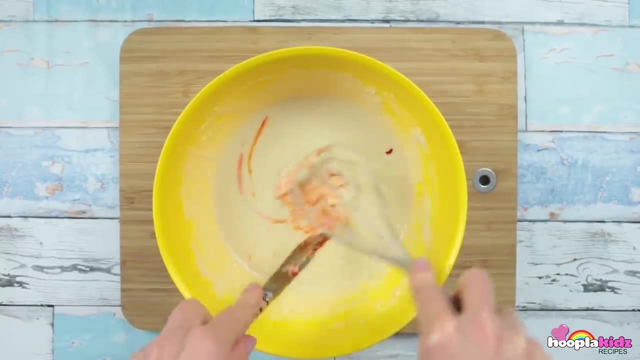 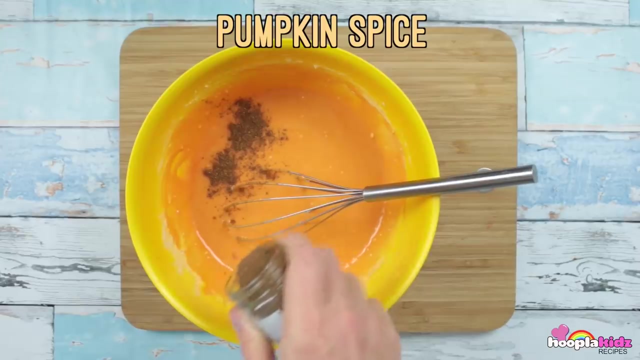 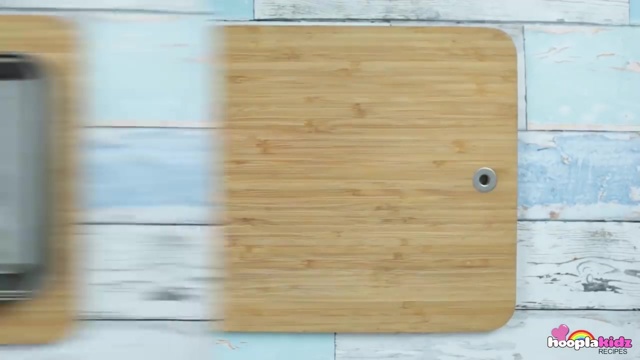 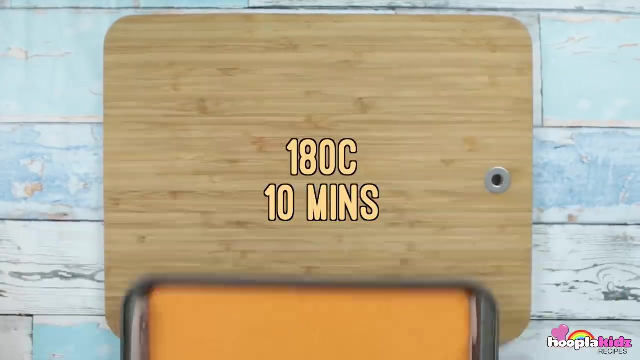 We don't want any lumps, if possible. Next, I'm adding some orange food dye. Give it a good stir. I'm also adding half a teaspoon of pumpkin spice. Let's add this to a lined baking tray. Bake at 180 degrees for 10 minutes. 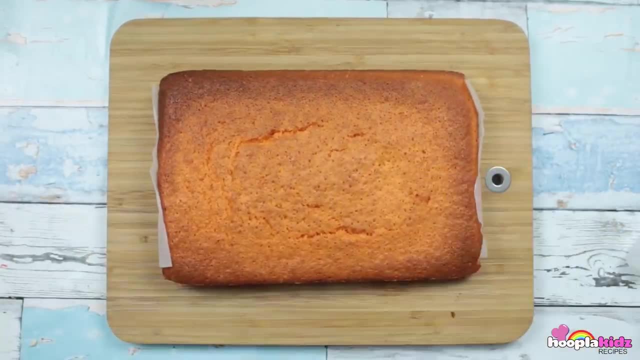 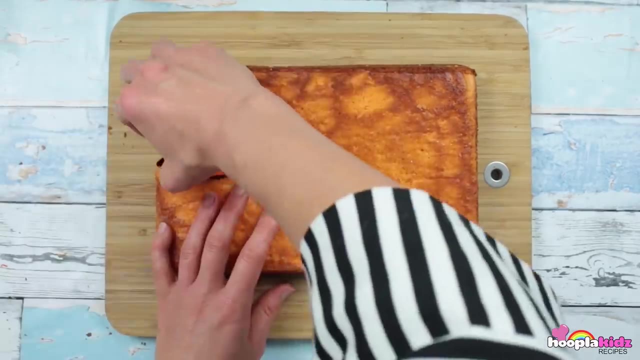 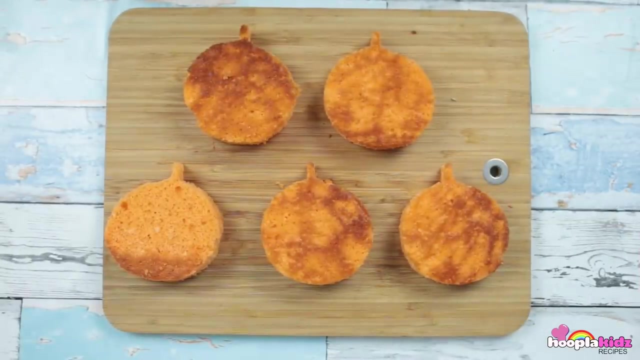 This is what it'll look like, so let's pop that out And there you have it. It's super delicious, Enjoy. I have a pumpkin cookie cutter and I'm going to cut out the pumpkin shape. Perfect, I have 5.. 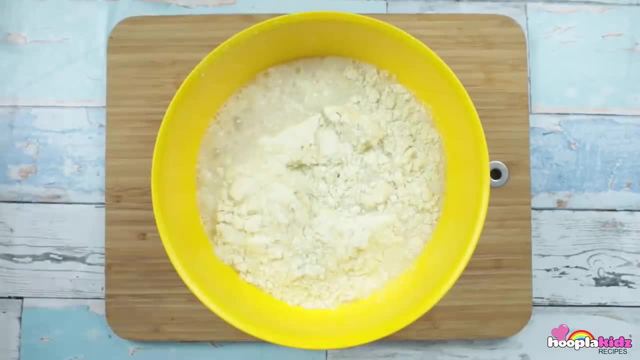 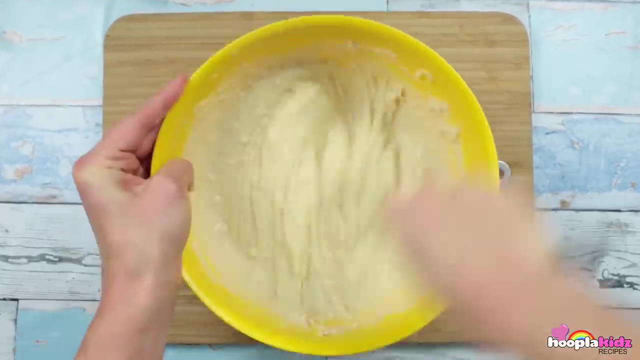 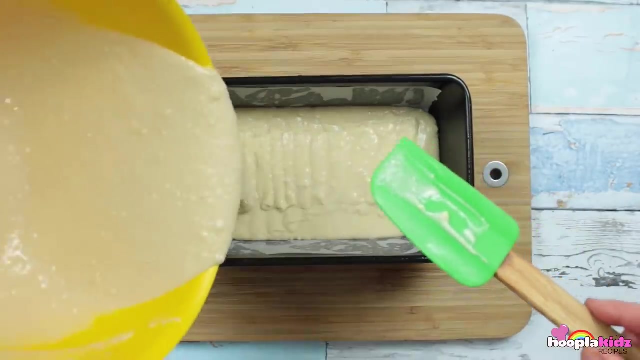 Now we're going to repeat the cake making process with 450 grams of cake mix, 1 cup of water and 3 eggs. Give that a good mix. We're going to add the pumpkin to a loaf tin that's been lined with baking paper. 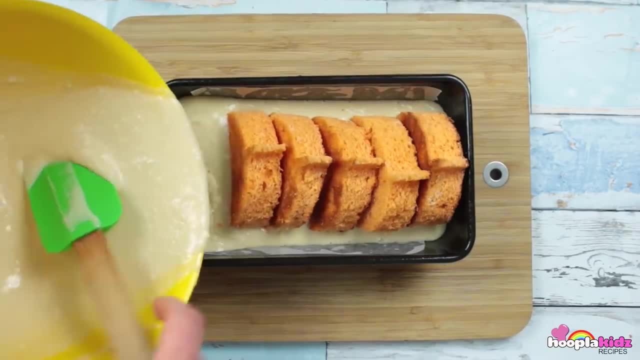 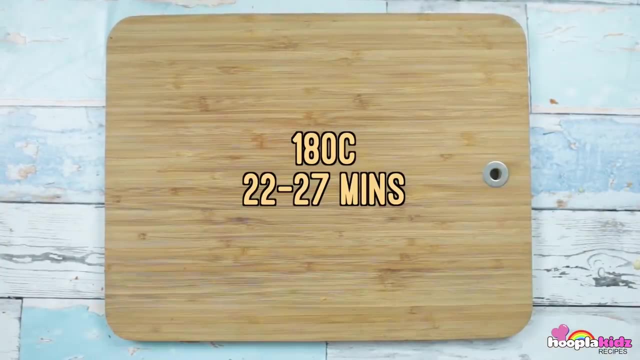 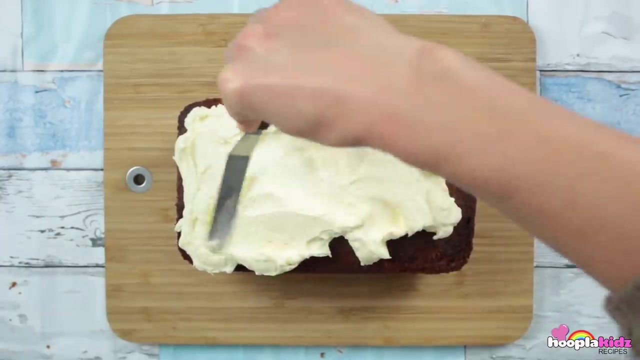 But don't fill it all the way up, because next up we're going to add our pumpkin shapes. We're going to bake that at 180 degrees for 22 to 27 minutes And what happens is that the wet cake mixture will overtake the orange pumpkins inside. 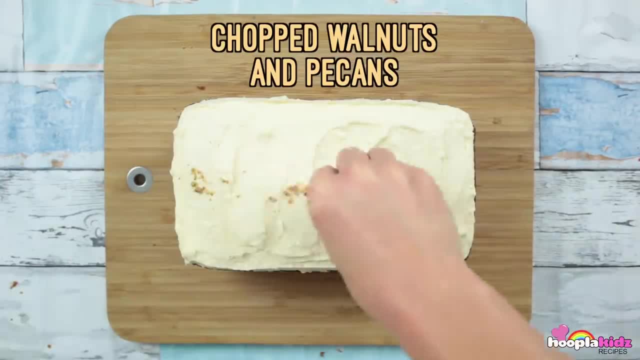 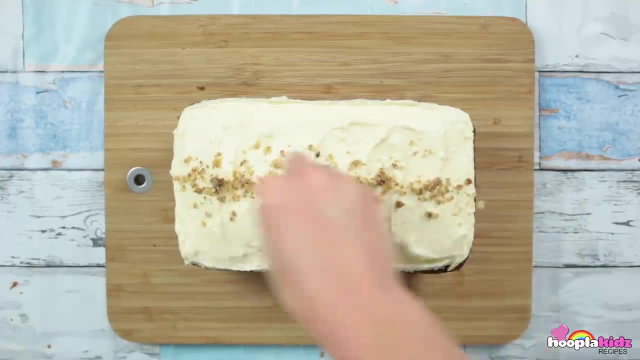 and you'll get an amazing loaf. Once the cake is baked, you can take it out of the oven. Once that's cooled, we're going to cover the top with buttercream frosting. Add some chopped walnuts and pecans to decorate. 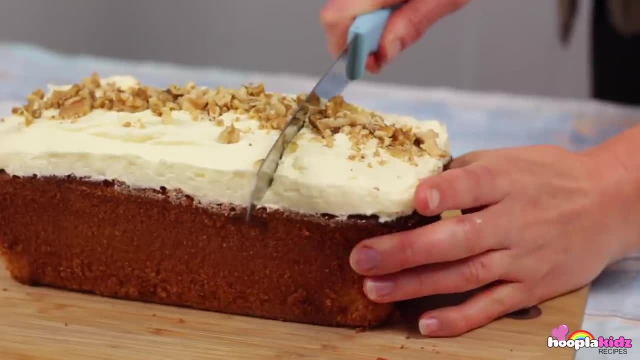 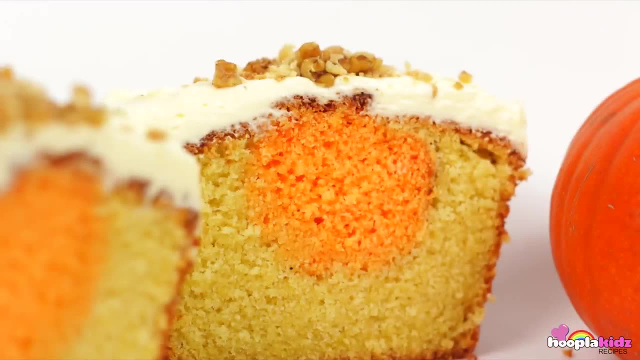 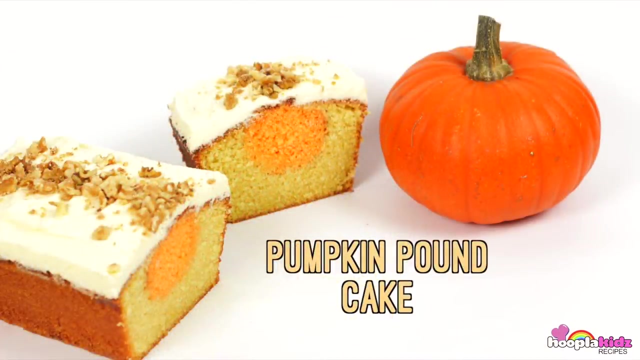 Delicious, Doesn't that look fantastic. And what's amazing is that when you cut into it, you'll see an awesome pumpkin. Very cool, A pumpkin pound cake- Super delicious. Thanks for watching everyone. we'll see you again next time. 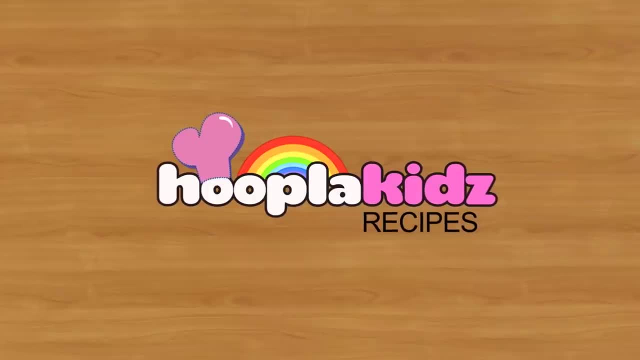 Bye, Bye, Bye, Bye.